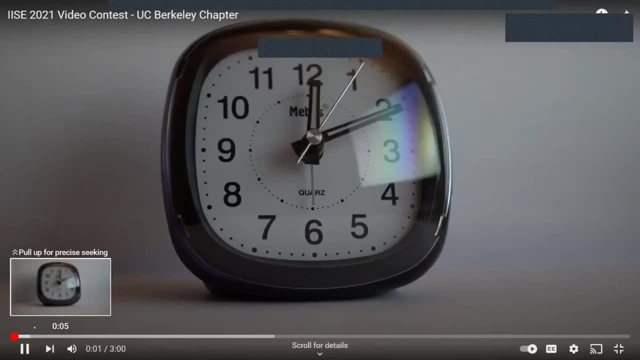 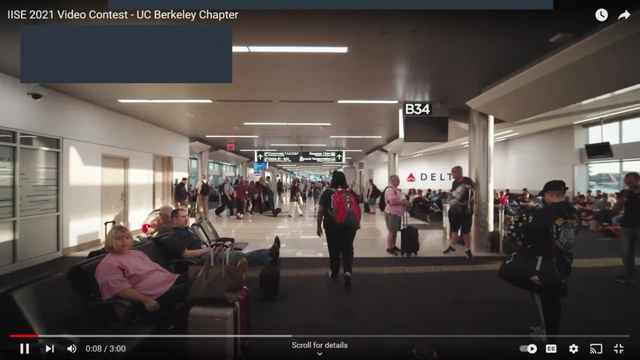 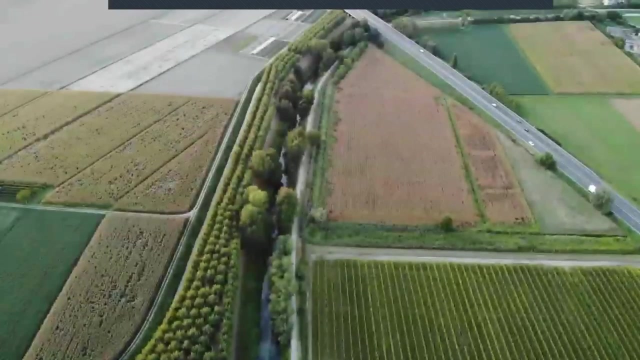 We spend so much of our lives waiting, Waiting for packages to arrive in the mail and waiting in line at the store. We wait and we wonder: is there a way for all this to go just a little bit faster? Industrial engineers work to solve this and so many more problems, But what? 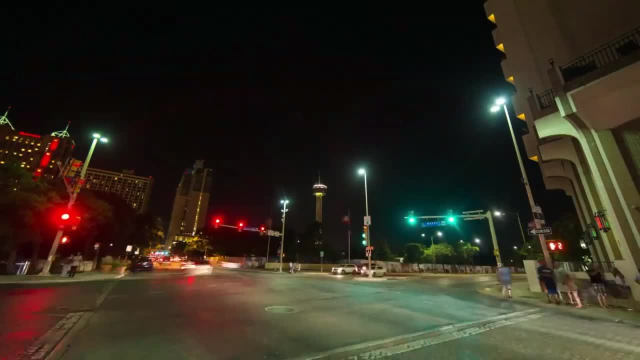 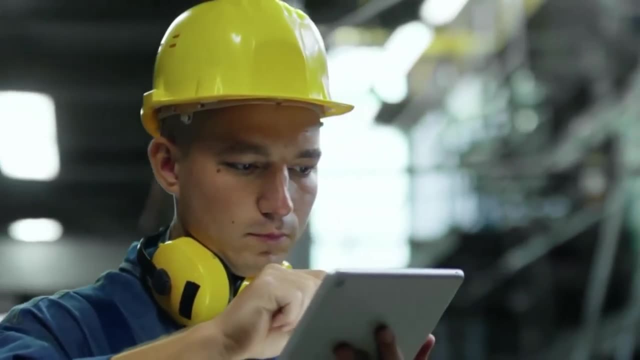 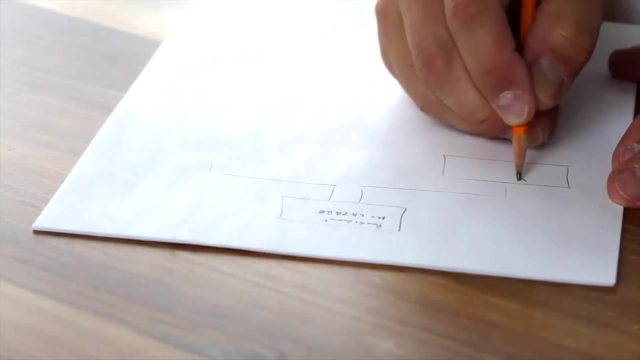 you might be asking yourself: exactly is industrial engineering? Industrial engineering is the process of inventing and designing ways to analyze and improve complex systems. It is about building better processes, not physical objects, in order to improve our world. We do this by studying math and statistics to understand. 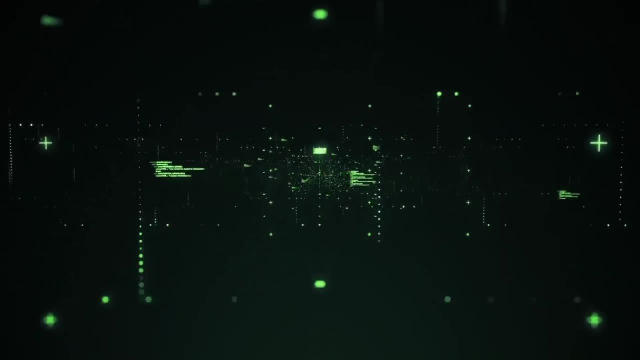 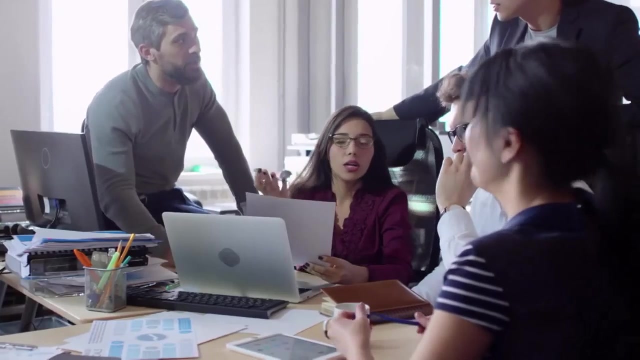 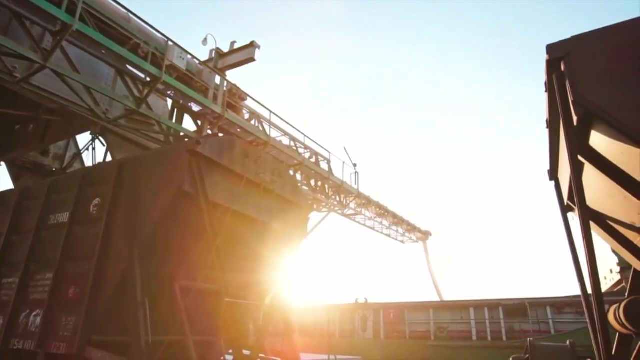 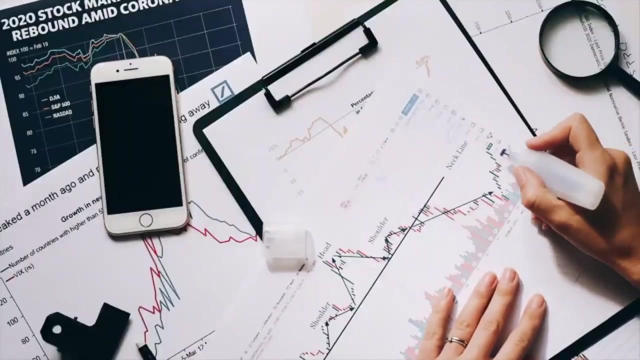 how to quantify everything around us. We study computing to better manage the massive amounts of information that are available today, And we study business to communicate these findings with leaders of industry. And how does this knowledge translate from the classroom to the world beyond? Industrial engineers work in all fields, from manufacturing to finance to entertainment. 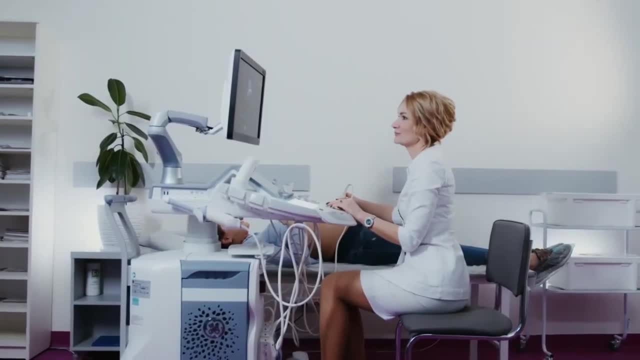 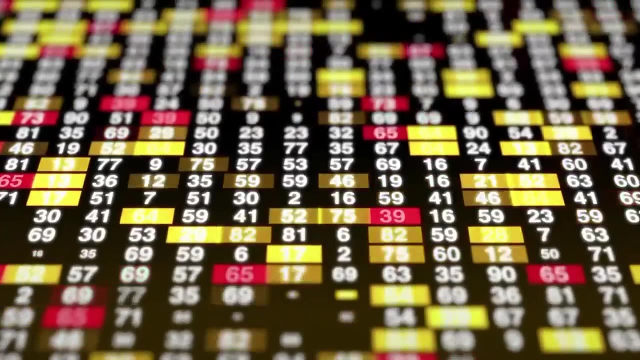 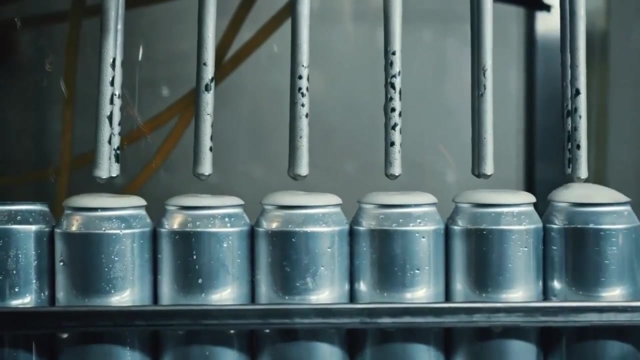 and everything in between. We standardize processes in hospitals, ensuring patients are able to see doctors and get treated as soon as possible. We analyze risk and finance helping companies and individuals make smarter investments with their money. We automate dangerous processes with the use of machines to reduce both the time to complete tasks. 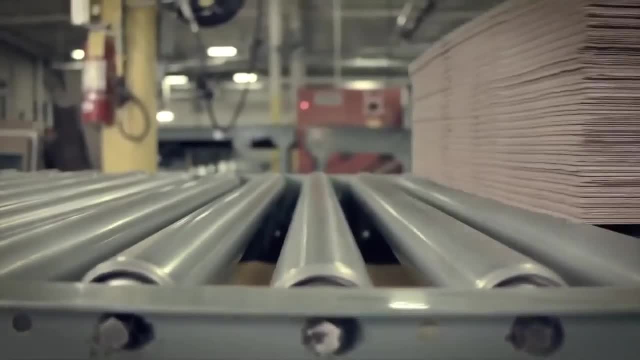 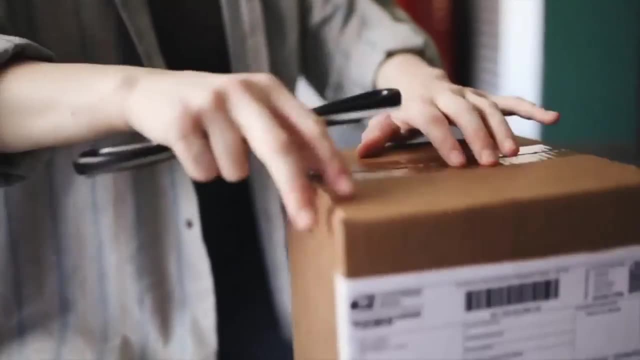 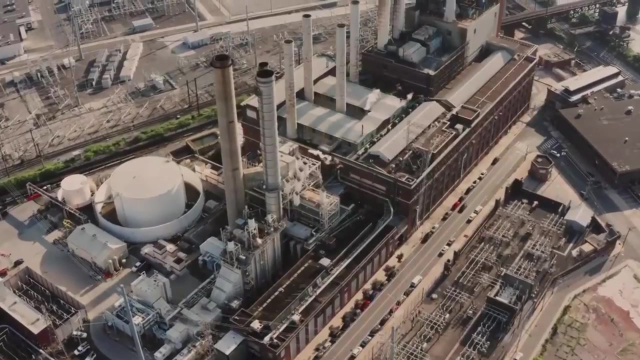 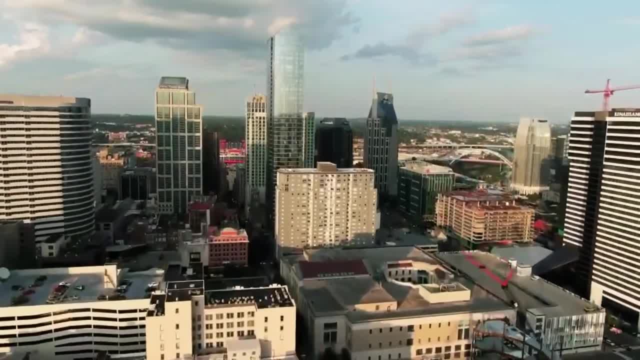 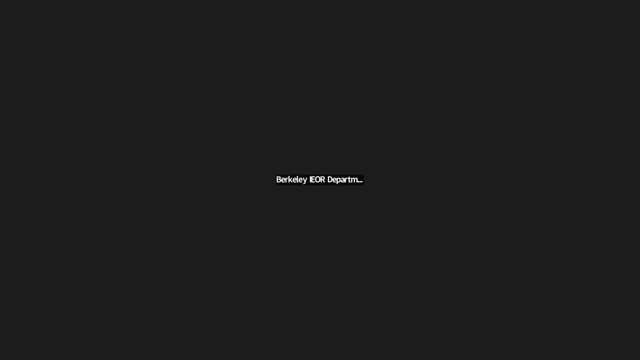 Made by our incredible students who are a part of the IISE student group. So now I will let Alper Adamturk, Professor Adamturk, take over. He is the department chair for IEOR and he's going to present. 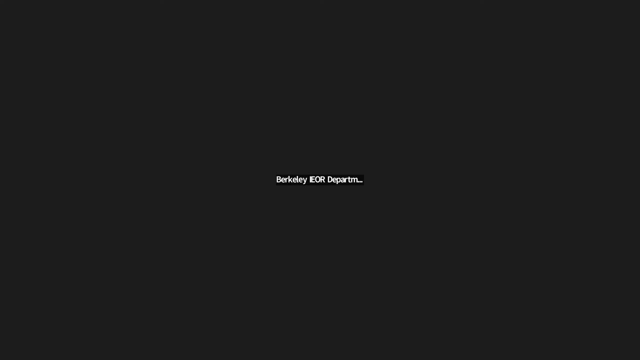 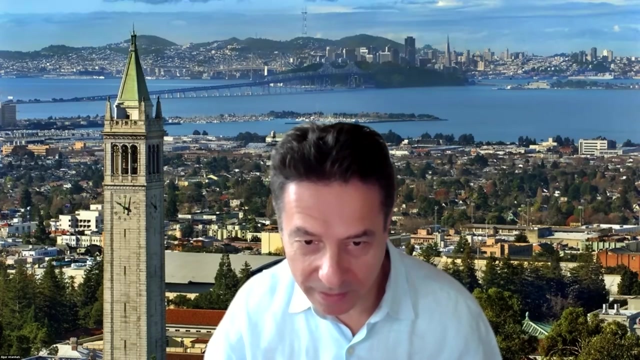 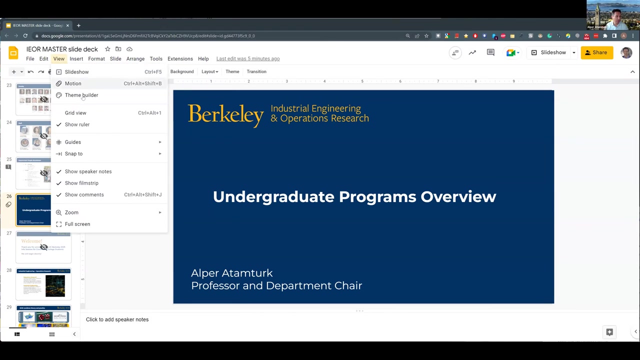 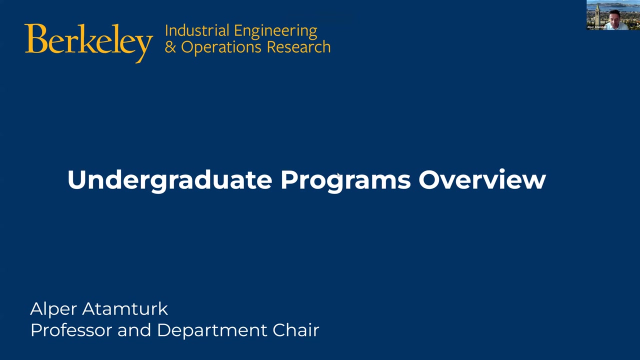 So, without further ado, Thank you very much, Goldie. Let me see All right, great Well, welcome everyone. Thank you very much for making time with us. We're delighted to have the opportunity to present to you what our department is about. 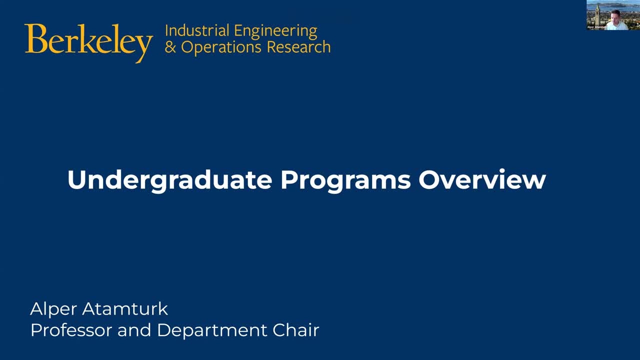 Our graduates, Our program. I hope you find this information session useful Together with me. we have a panel of faculty and staff members, as well as IEOR students, with us, And I'd like to introduce them first before starting the presentation. So I 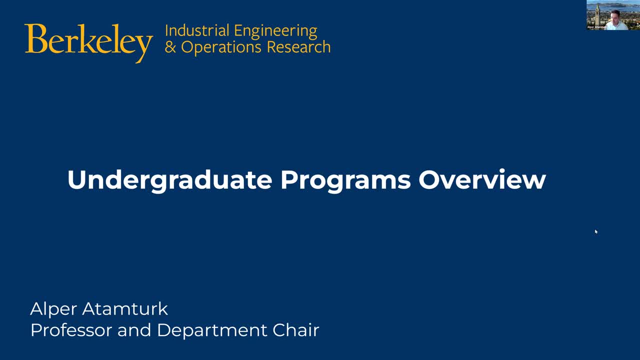 You heard from Goldie, So how about we start with Goldie? maybe a sort of quick introduction and then: Sure, Hi everyone. My name is Goldie Negalev, I do communications for the department And, yeah, that video is like gold for a communications manager. 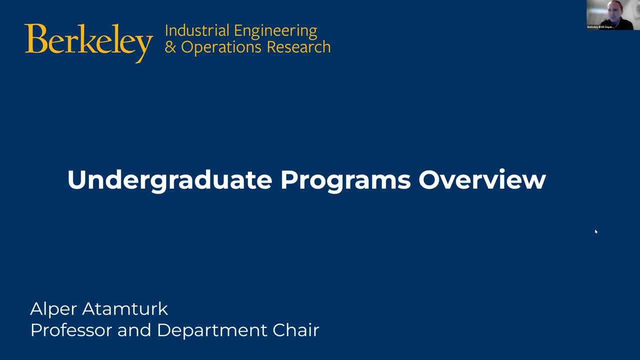 So every time I watch it I'm just really blown away by how amazing The students are at this department. There's really something special about Everyone I've I've encountered all of the students. They all share in common that they want to make an impact and they want to improve the world. 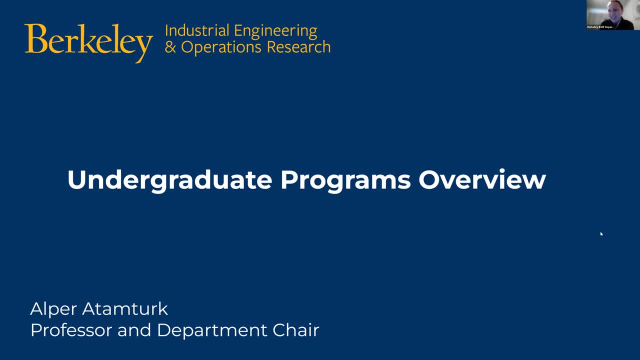 And it's very inspiring To do my job every day. So, yeah, I am excited for everyone to learn more about IEOR And I hope we get a chance to continue Talking With with all of the community college students who are on this call today. 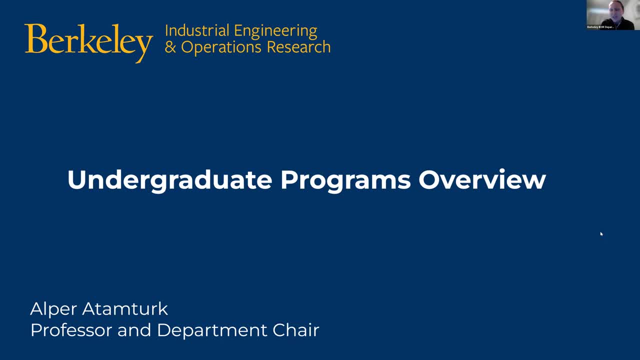 And hopefully This will lead to a longer You know, Conversation with with all of you. Okay, And then we have a genie. Hi, I'm in IOR undergraduate student services, So I can answer questions about The curriculum. 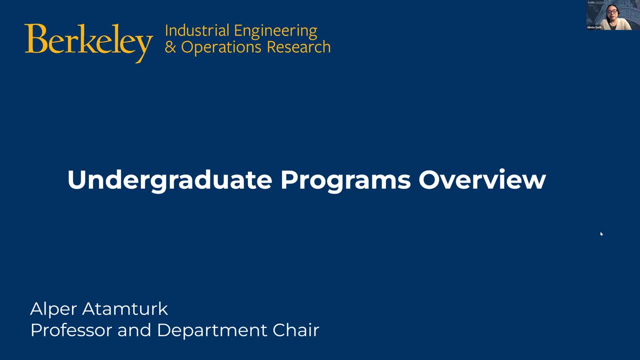 Once you get to campus, I'm your one-stop shop for the questions that you have about being at Berkeley. Work with closely with our undergraduate students to help them with classes and finding resources on the Berkeley campus. Great, Thank you. And then we have. 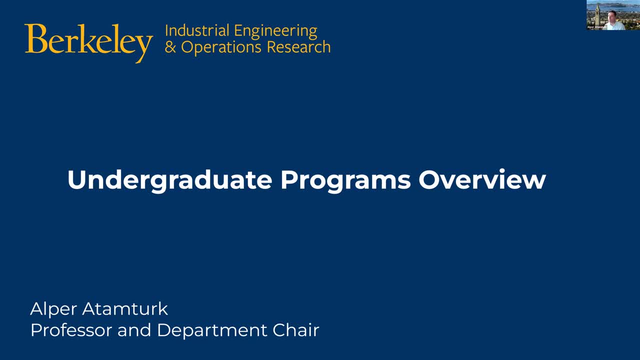 A faculty member, Rajan. Hi everyone, I'm Rajan. I'm, I guess, a relatively new faculty. I've been here for three years, I'm an assistant professor and I guess My research is related to online markets You saw a little bit about in the introduction of processes, So I'm quite interested in the processes. 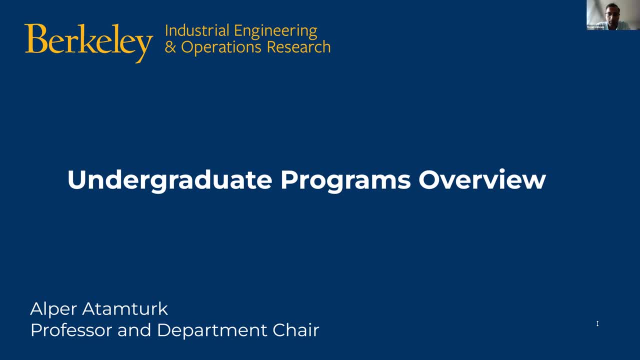 That we use in various kinds of online platforms, and I'll be more than happy to answer any kinds of questions you have, So please don't hesitate, Whatever the questions. Thank you, And then we have four IUR students, So let me start with. 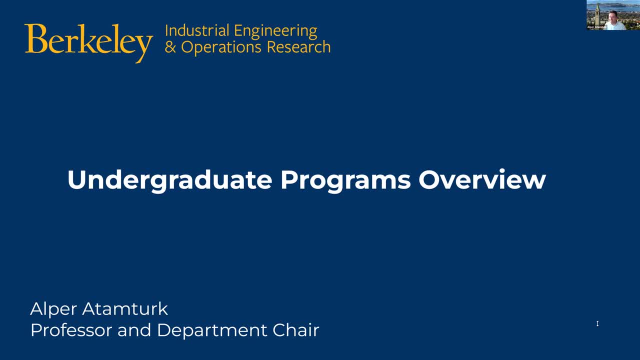 Jello, Jello Francisco. Everyone, My name is Jello Francisco. I am A transfer student from Danza college And it's my first semester here at Berkeley. Thanks, Jello. And then Victor. Hey, hello everybody. My name is Victor Gutierrez. I transferred from. 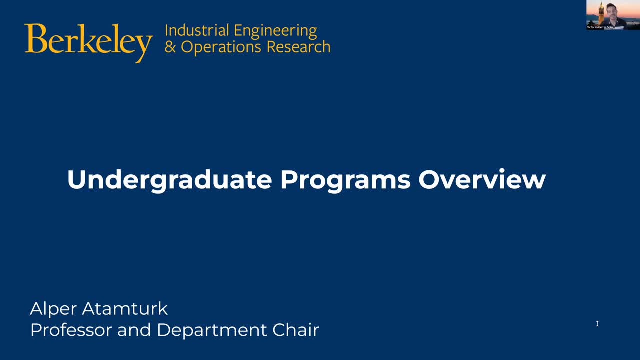 Mousa community college. She's in LA. Thanks, Victor Shrijal. Hi everyone, My name is Shrijal And I went to Contra Costa college, which frankly is Too far from Berkeley, But I'm currently in my third year at Cal. 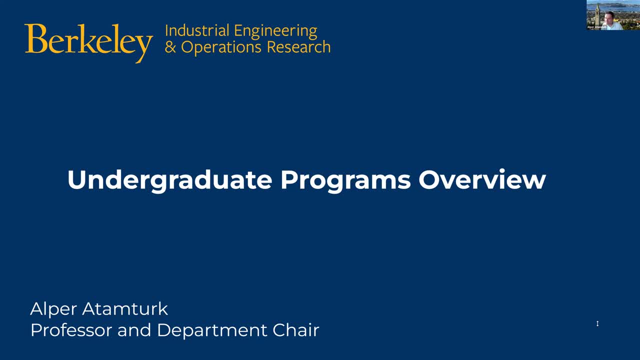 Thanks, Shrijal. And then finally, Avigyan. Hey everyone, I'm Avigyan And I am a proud transfer student. I transferred from Ohlone college In Fremont, So not too far away, And I am currently a senior in the IUR department. 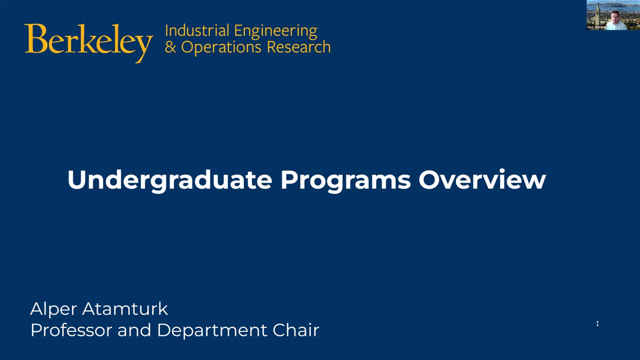 Thank you very much, Avigyan. Thank you. So my plan is to have a short slide presentation about the department but the program, and then we'll open up for questions to To the panel. All right, so let me. 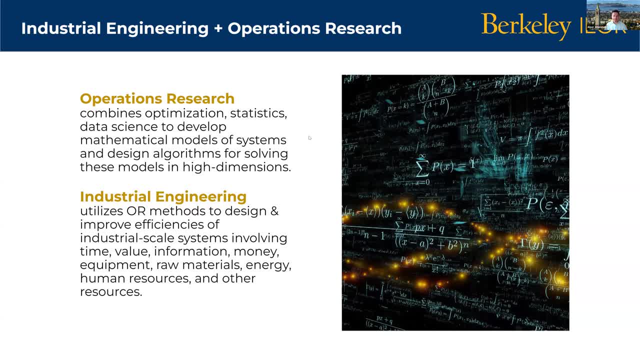 Start. So our department Has. this is named industrial engineering and operations research. It is The combination of two Highly related fields. In case you're wondering What operations research is, It is a field of study that combines optimization, statistics and data science. 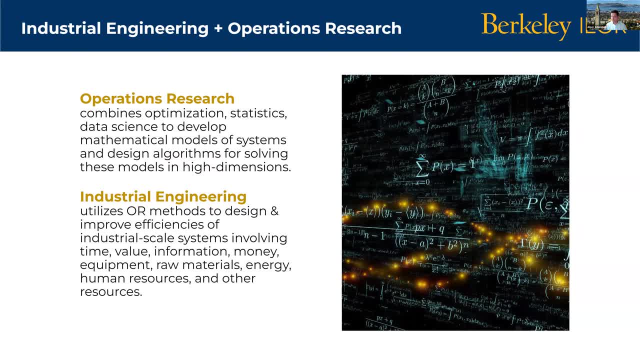 To develop mathematical models of our world, different types of systems, And then design algorithms to solve, come up with solutions to these systems in high dimensions, Whereas the second Related component, industrial engineering, refers To The analysis Of Systems at the 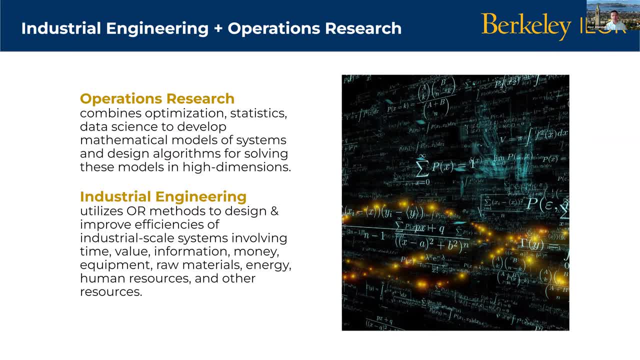 Industrial scale, large scale, and uses the Or methods Developed To Either design or improve efficiencies of these systems and systems. often Time, Value, Money, Information And raw materials, Energy And other kind of resources, And when I 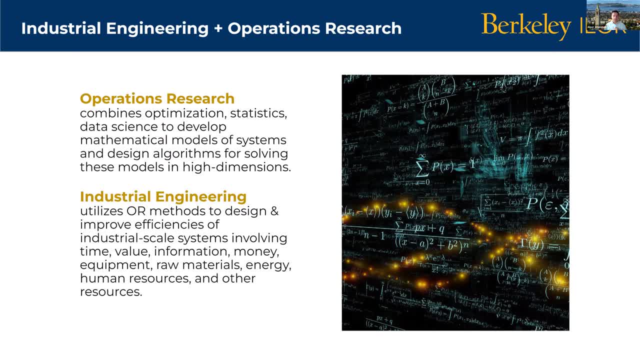 Say systems We're really thinking about In this context? Industrial systems, business systems, such as Talking about an airline, You may be talking about a hospital Right, Maybe talking about a A bank Right, Or or. 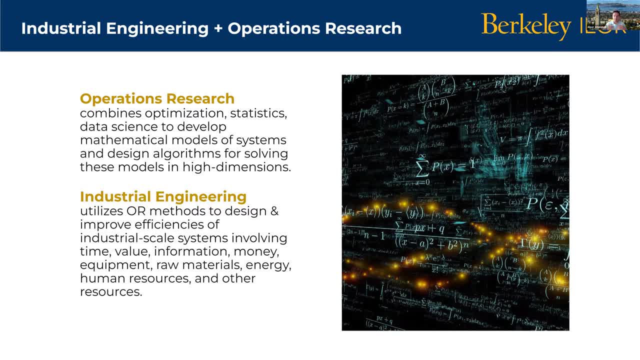 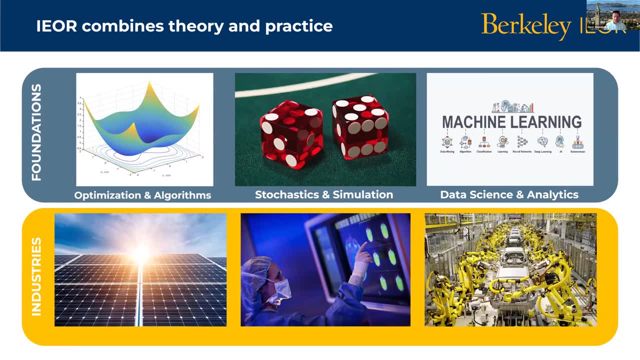 We may be talking about a Manufacturer of some Some product. So Our department combines both theory and practice. on this theory side, On the foundations, We have a set of courses that train students In Optimization, Modeling of uncertainties, stochastics and simulation. 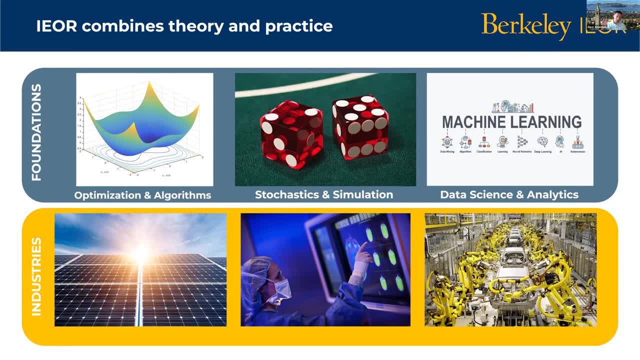 And, and more recently, Data science and machine learning. And then, on the more practical side, We have an emphasis on several sort of areas, Whether it's the energy systems, And we may be Addressing questions such as how to best incorporate 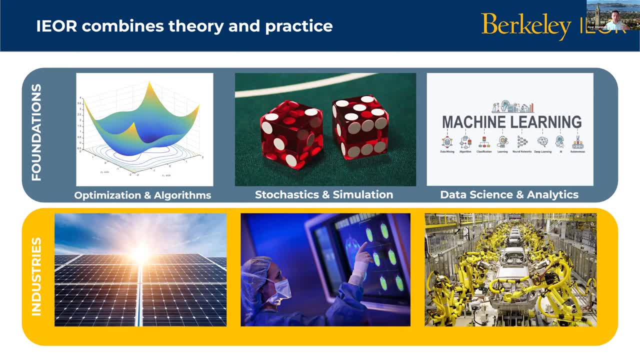 The renewable Generation wins resources and solar resources, which are highly stochastic Into the. our power grips Grids in the most efficient way, Or healthcare systems, And we may be asking questions here: How to best Diagnose Diseases as early as possible and how to come up with 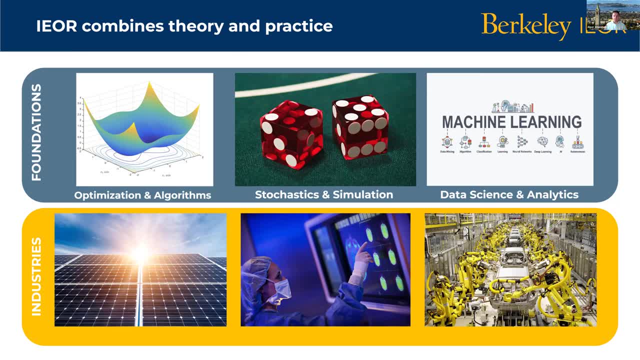 Treatment, Personalized treatment, Highly optimized. that way, And if you go to the sort of the other corner here, We could be maybe Talking about a manufacturing system And how to best Utilize the raw materials, The how to best. 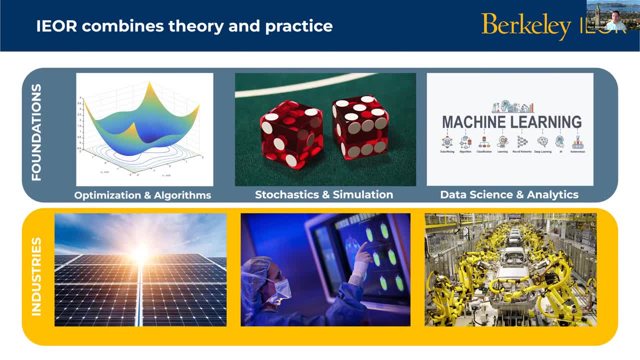 Utilize time In a more efficient way So that we produce The Largest amount of sort of products In a short amount of time at a low cost is as much as low cost as possible. So These are the kind of systems that we're talking about. 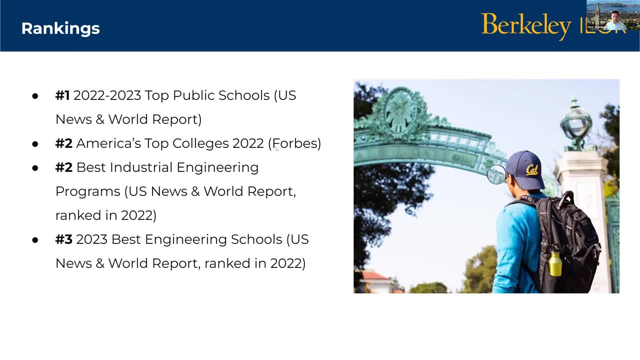 We're talking about the high level industrial Scales of systems. Our department and university is highly ranked. As you know, a U S News and world report Ranked UC Berkeley as a top public school And our Program Is ranked number two. 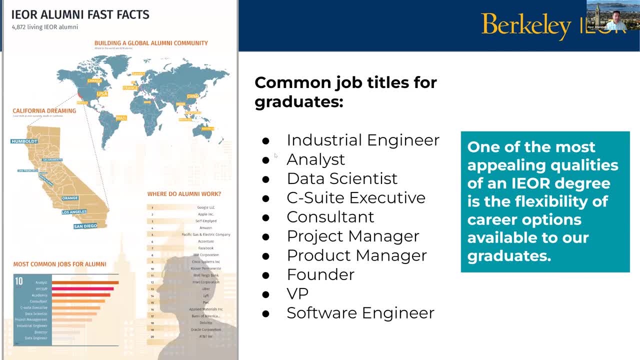 And our college was ranked number Three And And Our Faculty As a top Student, And so We Sort of give, We want to give us sort of Quick sort of Profile of where our alumni sort of go and what they do. 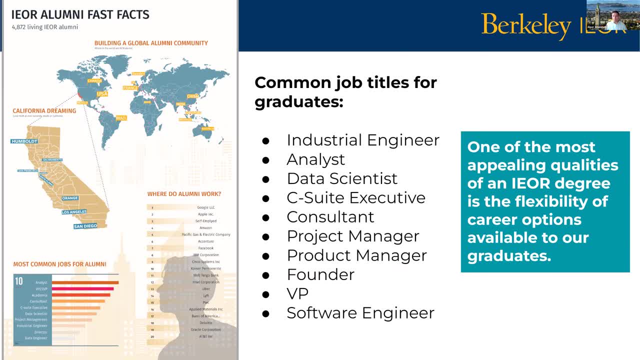 what they come. So you see this sort of job titles of our graduates, Right. So industrial, It's this. no, no brainer. They can be business analysts. They can be Boy as data scientists. Often They quickly move up to. 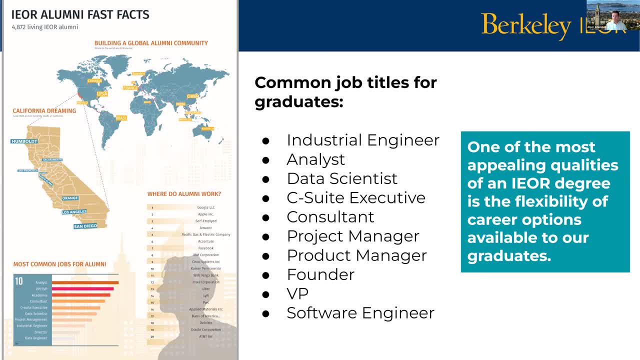 Senior management And of founders of companies, CEOs, CFOs et cetera, of well-known companies that are IOR, are alumni and various other sort of job titles On the left. you see that it is really a sort of broad community. 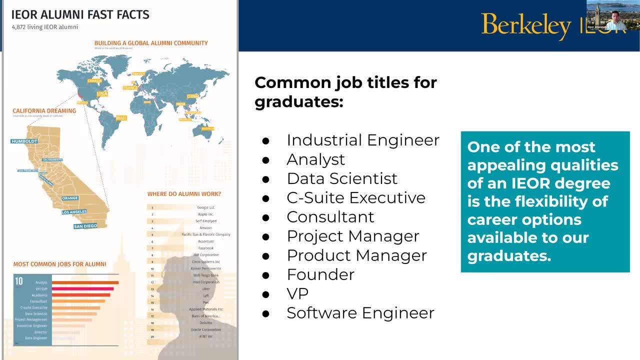 We have alumni that is working throughout the world. It's not just in California, but it's really a global community. One of the very nice features of our field is that, with the skills that students are equipped once they graduate, they can find jobs. 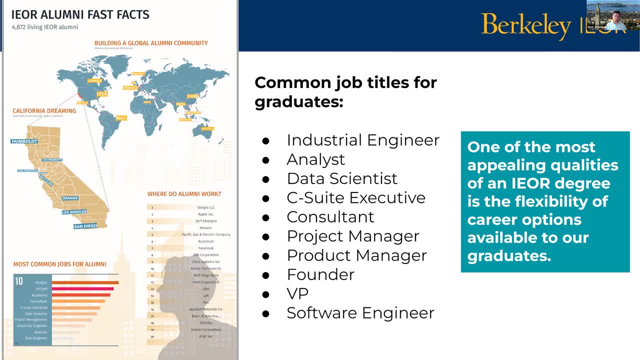 pretty much in every industry, all right. Not restrict to a particular industry, whether it is in construction or just in electronics, right. So they can pretty much work in every industry. so it's highly flexible And it is also highly resilient. As the economy is booming, industrial engineers find it easy to find jobs like in every other profession. But on the other hand, when the economy is contracting, businesses start seriously about how to run their operations most efficiently, and then they need even more industry. 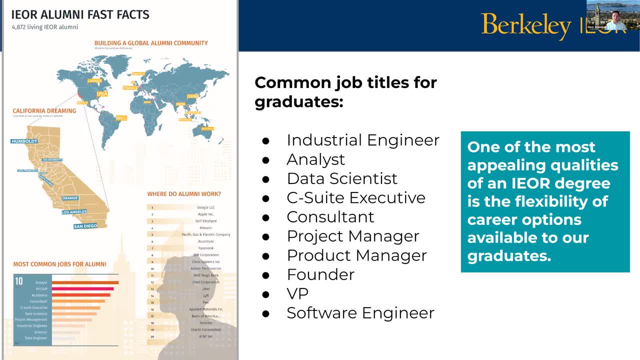 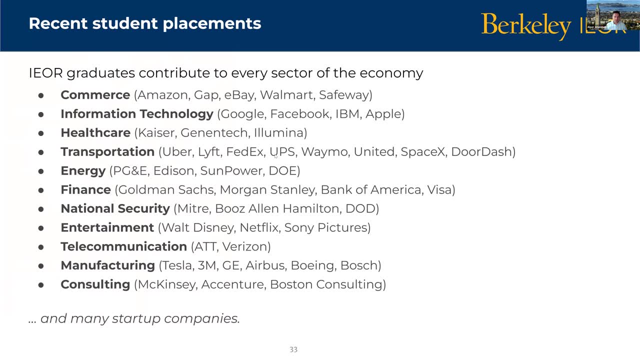 engineers, So it is a very resilient profession with respect to the ups and downs of this economy. This slide shows some of the recent placements, and the point I want to get across here is: really, our students contribute to every sector of the economy, whether it's e-commerce, information technology. 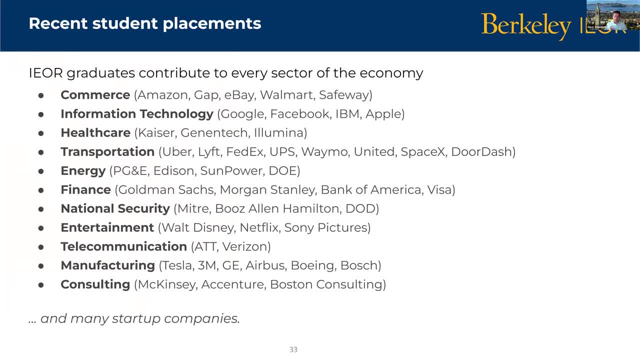 healthcare. I see that SpaceX is very much interested in our students recently, and so definitely in entertainment, in manufacturing and many of the startup companies in the Bay Area employ our students, and many of them are actually started by our own students, In fact. 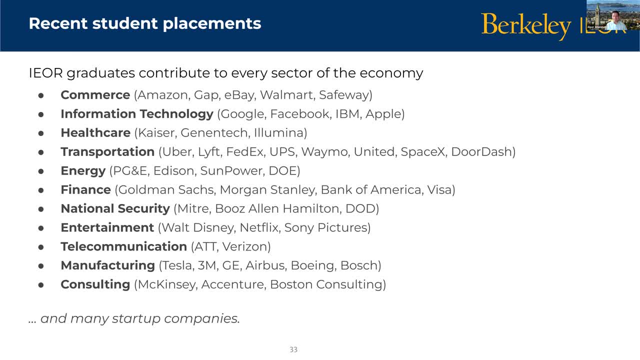 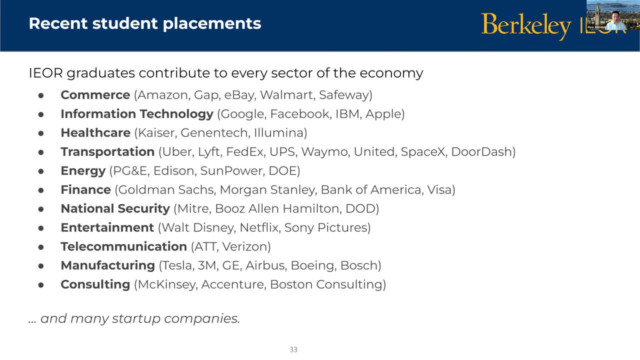 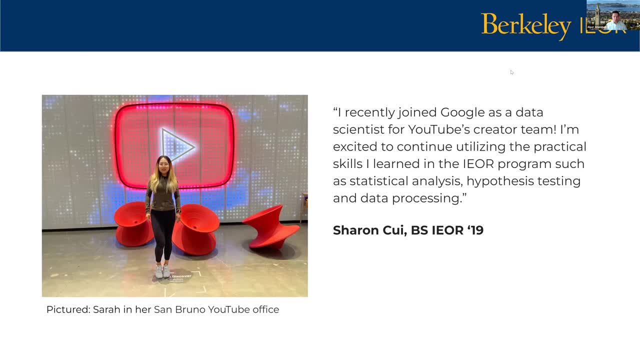 been working on this for a long time. They have been working on this for a long time. They have become extremely successful in the last few years. A couple of profiles that I want to list here. A recent IOR graduate, Sharon. she mentioned that she recently joined Google as a data scientist for their YouTube creator team. 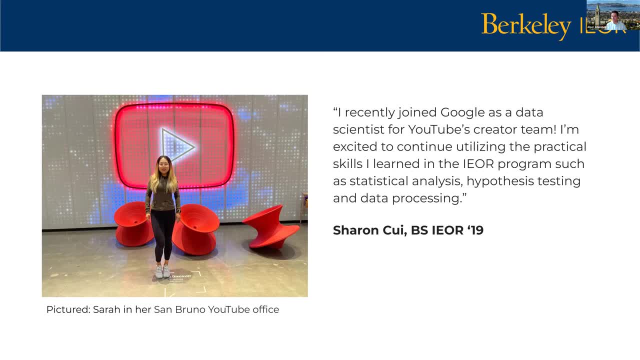 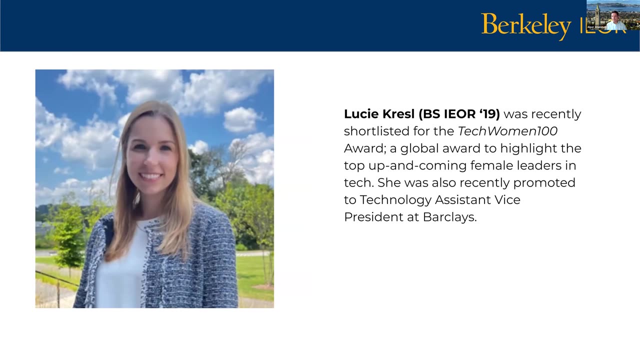 She is very happy to utilize the skills that she learned in IOR, such as statistical analysis, hypothesis testing and data analysis. Another profile: Lucy Kressle. she's been recently shortlisted for the Tech Woman 100 award. She is in the finance sector and recently was. 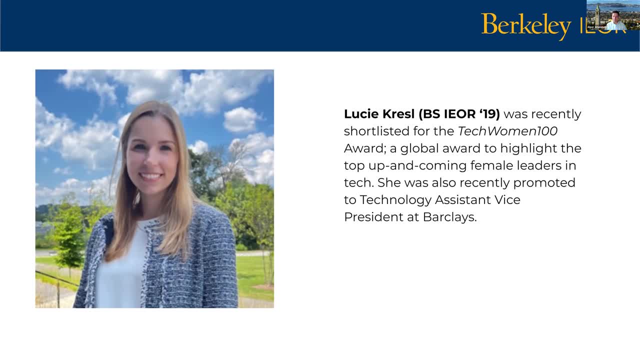 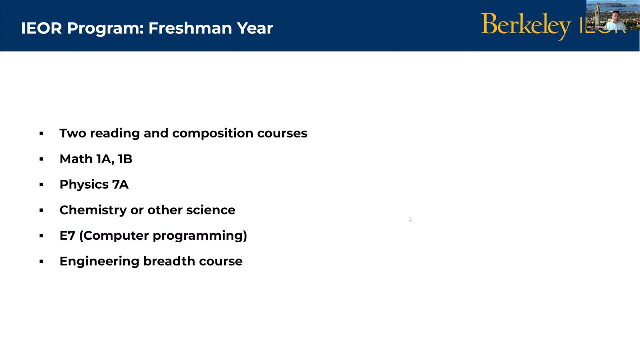 she is in the finance sector and recently was promoted to Assistant Vice President of Technology at Barclays. With that I want to quickly go over this high-level introduction. I want to quickly go over our undergraduate program For community college students, the first two years. you probably 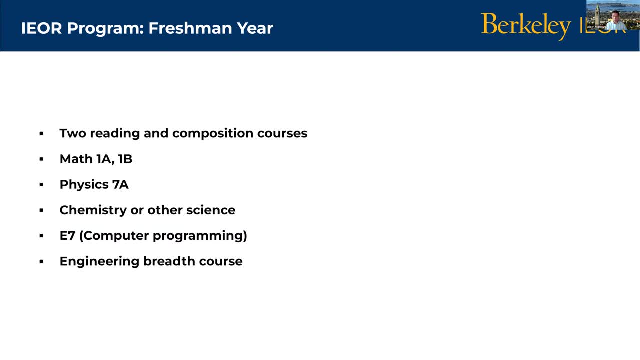 have taken these courses, but it is an opportunity for you to see the courses that our freshmen and sophomore students take. In case you don't have those courses, you may find it valuable this year to go ahead and take those courses so that you're ready to take on upper. 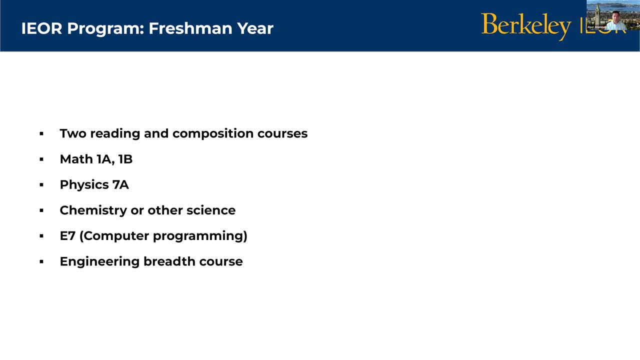 division courses in the IU Art Department. So the freshman year. typically the general requirements of some degree courses are the following: First of all you're going to have to complete the reading and composition courses and math A1B. These are basic calculus courses. physics 7A. 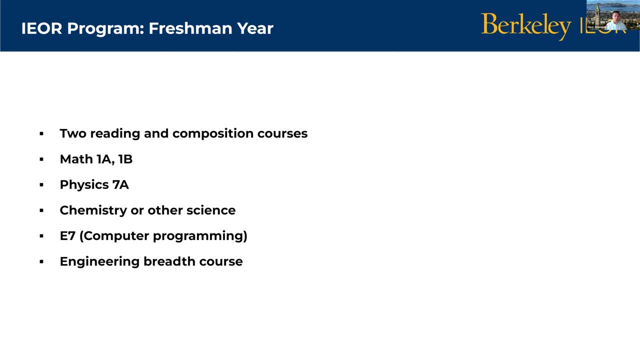 and chemistry. We have a computer programming requirement- E7, or there are some other alternatives to that particular course. It doesn't have to be that particular. That's a MATLAB-based course, but you may if you have fluency in some other languages. 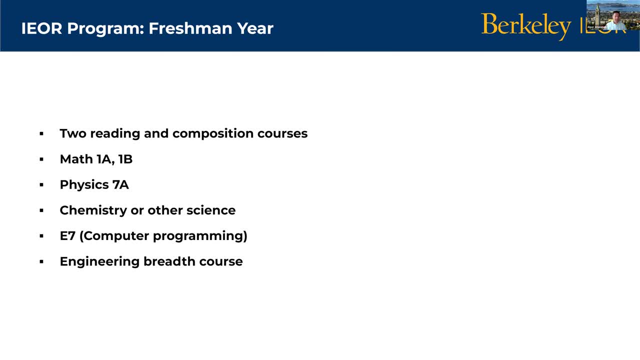 through some other course. that is fine as well, and students start taking engineering breadth electives And then sophomore year goes into a little more advanced math. that includes linear algebra, differential equations and physics. 7B Students use this year to take additional 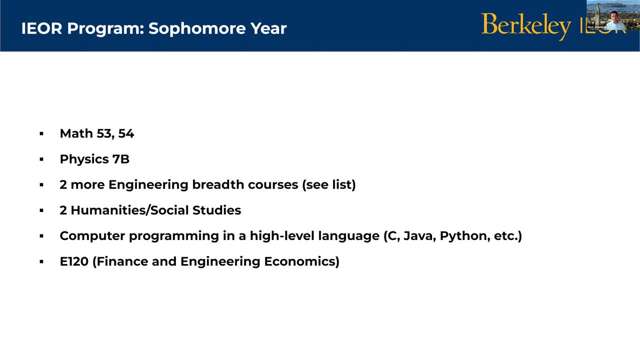 breadth engineering breadth requirements. These are required across the college, typically courses that are outside of the department, And I have a list of what those courses might be in the following slides: Two humanities and social studies courses and another computer programming course. So we asked our students. 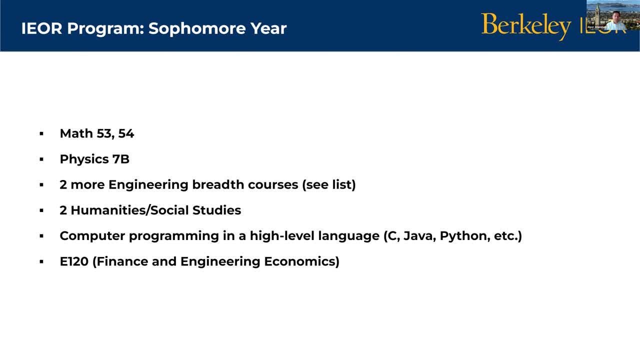 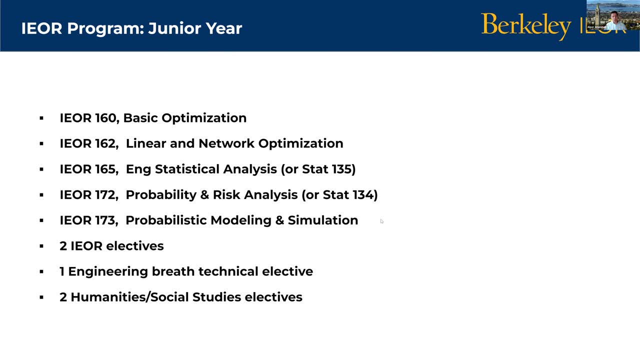 to take two computer programming courses And then engineering economics course, the L1, torrent C. Thank you. So if you're joining the department from a community college, typically you start in your junior year and these are the courses that you'll be taking: The courses in the junior. 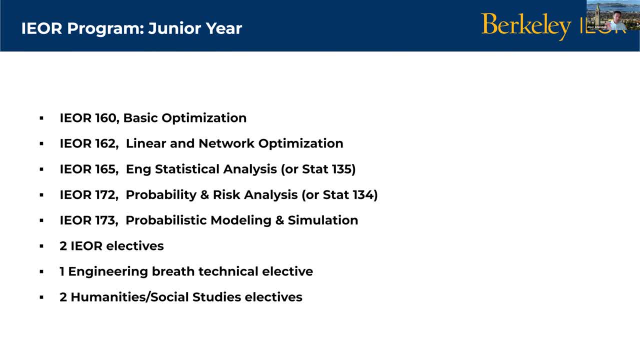 year are these foundational operations, research topics courses. So they include basic optimization, 162 linear and network optimization statistics course, a probability course and a probabilistic modeling simulation statistic analysis course. Then students also start taking IEOR electives- I have a list of them coming up soon- And also they use this year to 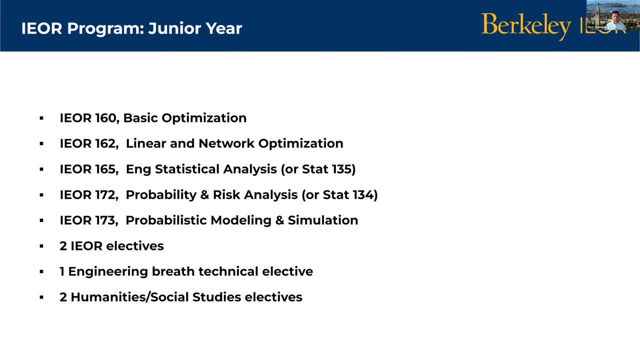 continue with their engineering requirements. Typically they take also humanities and social studies electives. So this is a recommended list. There are obviously variations of it depending on the needs of the students, And you may find a more technical course you may take. 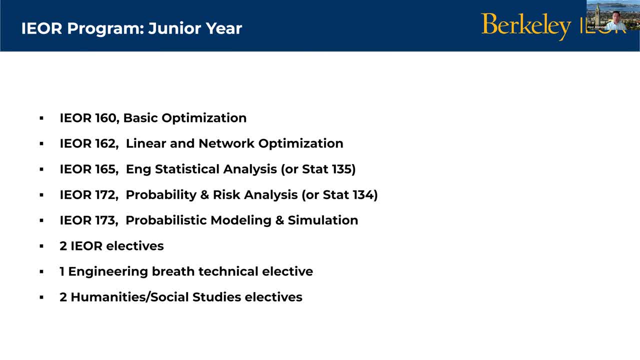 three technical courses instead of two, or you may take more humanities courses this semester this year And then more technical in the senior year. So there is flexibility around these. But the basic optimization, probability and statistics course- they are prerequisites for the senior year. So 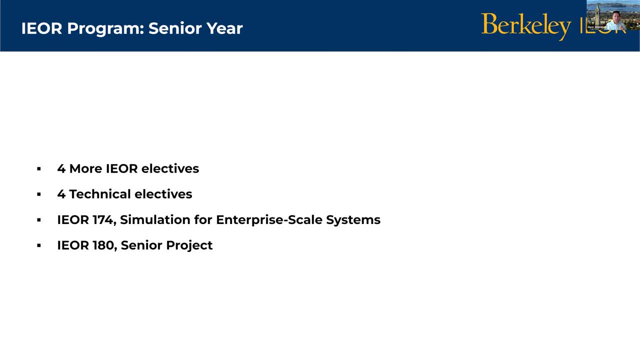 they must be taken in the junior year. In the senior year students take four more IEOR electives and four additional sort of technical electives which are outside the department- a senior year- And they do a senior project design course where they work in teams as in groups. 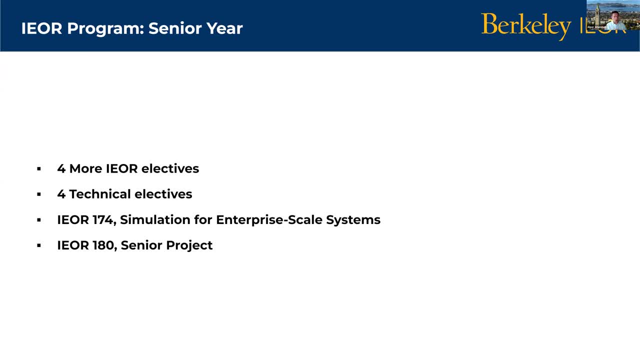 and work with companies. So they go out and utilize all the knowledge they have gained throughout their studies in the IEOR department and deploy them in an industrial context with the firm. And then they, you know, write a report at the end of the semester, do a project presentation. 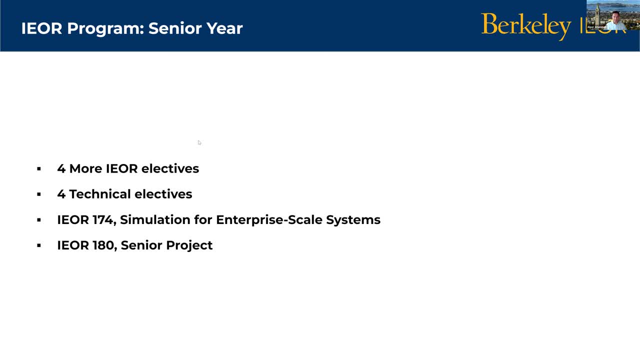 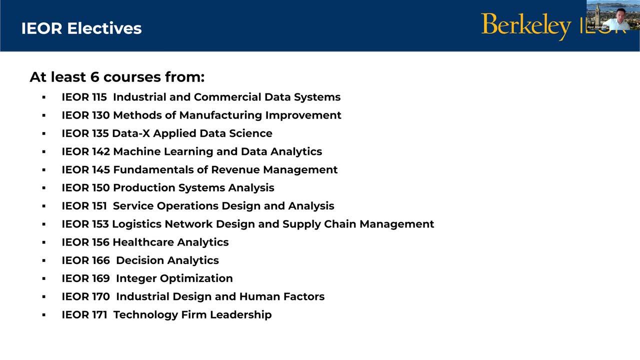 So technical communication is part of IEOR. So here's a list of the elective courses that I was referring to And I'm going to go over the names because it tells you sort of diversity of the topics that we cover. The first one, IEOR 115, that's a database course, Industrial and Commercial. 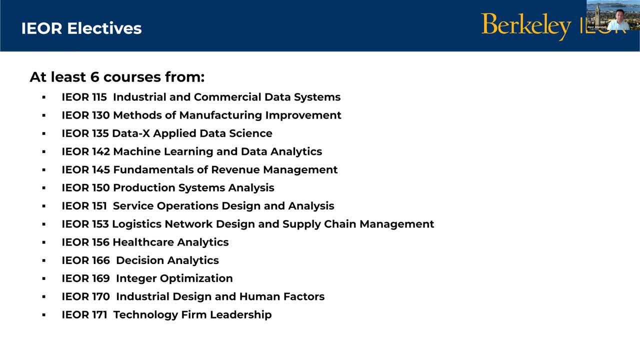 data systems where students learn the language s, sql, um and um. it's a relational database language. and uh, the, the other course in methods of manufacturing improvement. that's related to manufacturing, obviously, how to run manufacturing operations much better. uh 135, a very popular course, an experimental applied data science course where students do a lot of hands-on projects. 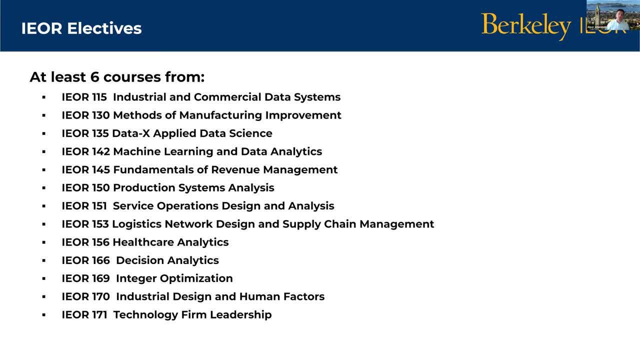 142, but more so advanced machine learning and data analytics course. these two courses are were introduced uh in the last five years or so due to the demand uh that we have seen in the uh data analytics, machine learning some area from our students and also from uh the industry. 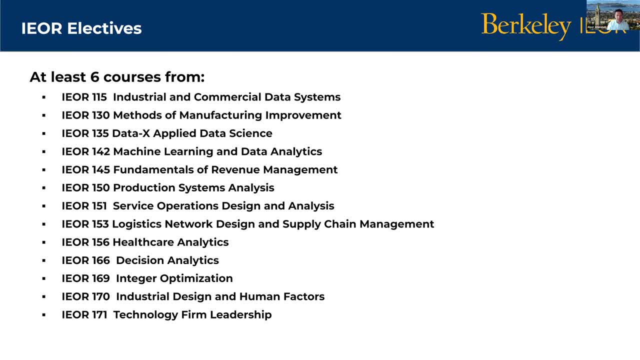 um uh iur 145: fundamentals of revenue management. uh was introduced by uh professor rajan rwani uh very recently. is uh his uh research area expertise and um 150 production systems analysis. it's uh a bread, bread and butter of our program based on how to again uh improve uh production and inventory. 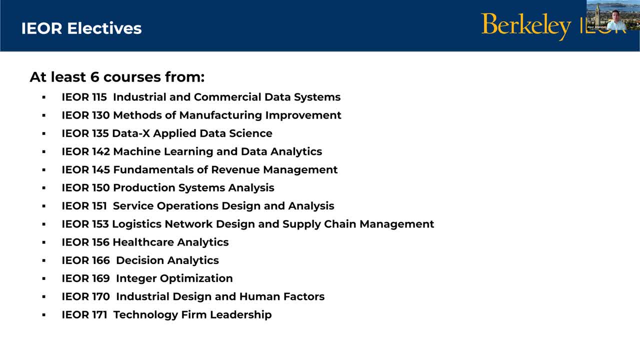 systems 151- service operations. so we are interested in improving not only manufacturing production but also the delivery of services. a big part of our economy is the service operation service industry. this course was introduced about 15 years ago so as services started to become occupy a much bigger share of the economy and uh logistics. 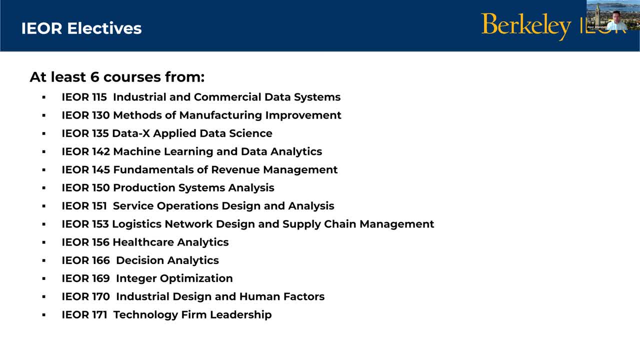 and supply chains: 153.. healthcare analytics is a new course. uh, it's going to be offered um this academic year in the spring for the first time. professor anil is one is going to teach that um again. that is due to the demand that we're seeing in the from the healthcare industry. um. 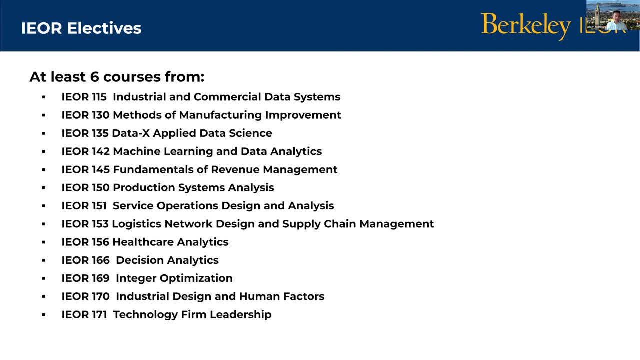 166, decision analytics, uh. 169 of an advanced optimization course related to uh problems where decision variables have to be discrete um plus accommodative optimization. problems um arise when you're designing systems. um. 170 um industrial design, human factors- uh, of course. and finally 171 um firm leadership, um as as we find our 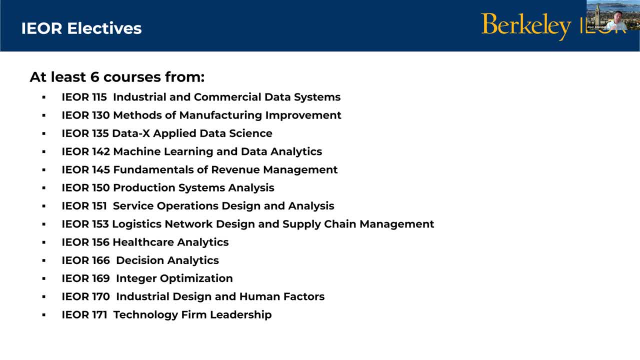 students going these courses, um, going into management, uh, very rapidly and creating their own companies. we found it really that it's important to educate them on leadership and entrepreneurship as well, and that is the topic of that, of course. so i'm going to stop here and open up for the q a session. 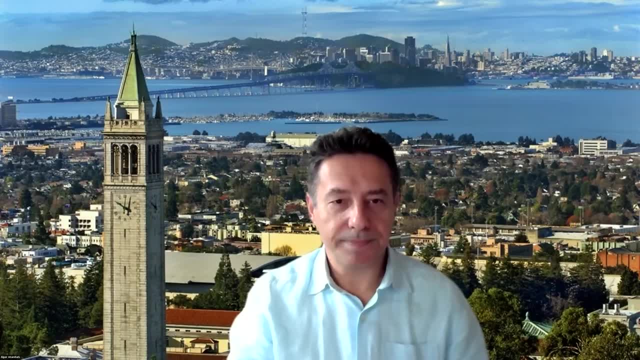 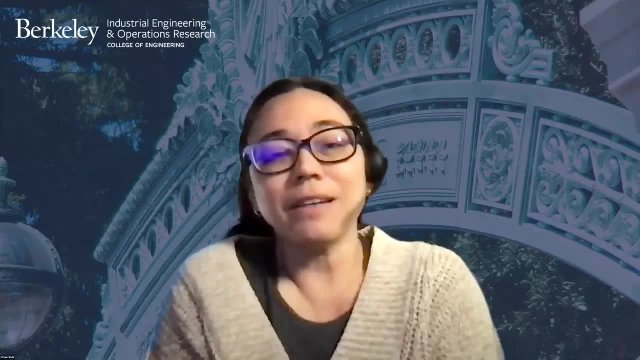 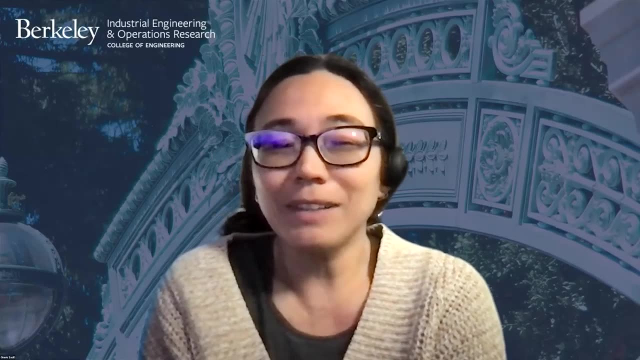 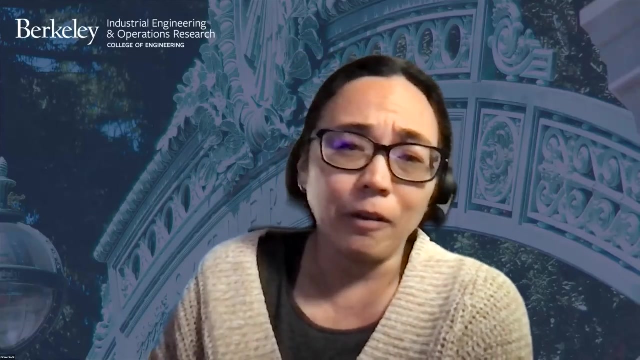 system. we have four great students and and two faculty here, so this is your opportunity to find out more about about berkley, about the program, about the process and what it's like to be a transfer student on campus. um, the the first question i want to ask all of our- our student panelists and 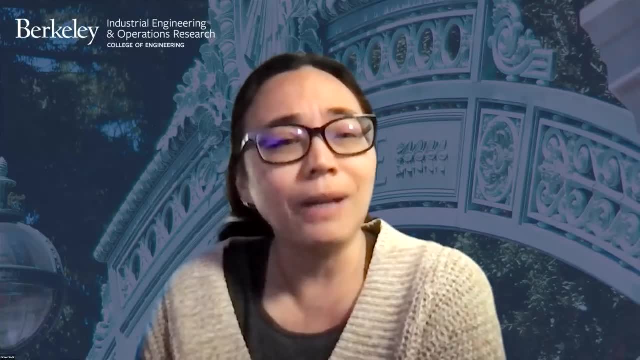 kind of our faculty as well, is: why did you pick i were what, what? what interest did you have written when you started here at journal, personalized storage or student offices, as an example of what is what from um? what are some of the considerations that relacionate eastern 벌써? 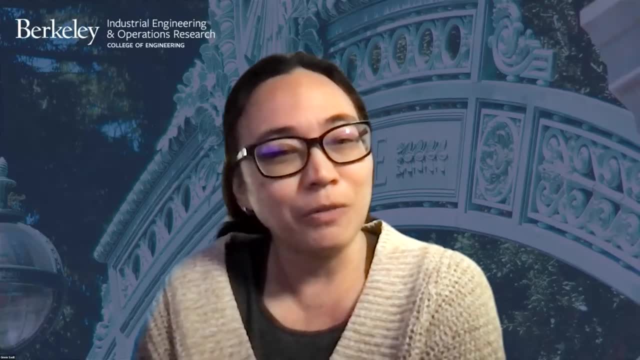 one we like to reallyrolling. what practices and services are that are really important to find in уsharen? i think this is one of the many individuals who have accepted campus and i think interested you about IUR that that brought you to the university or into the major. 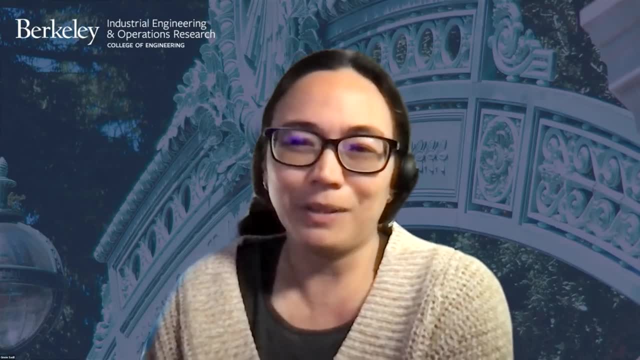 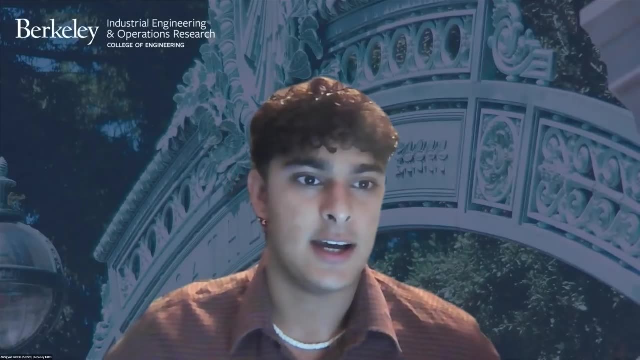 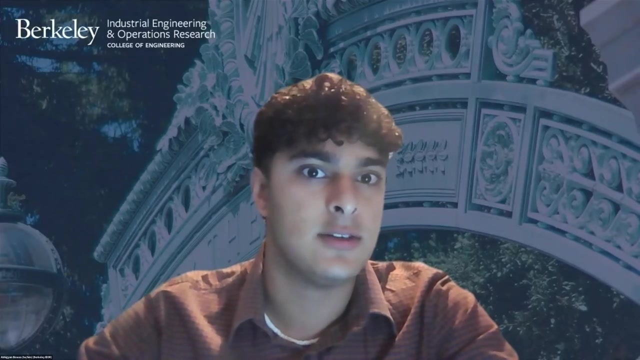 And we'll go with Abby. Do you want to? do you want to share your thoughts on that? Sure, definitely, Jenny. One of the reasons that I chose well IUR in general as a major is because I felt like it was the perfect intersection between engineering, business operations and 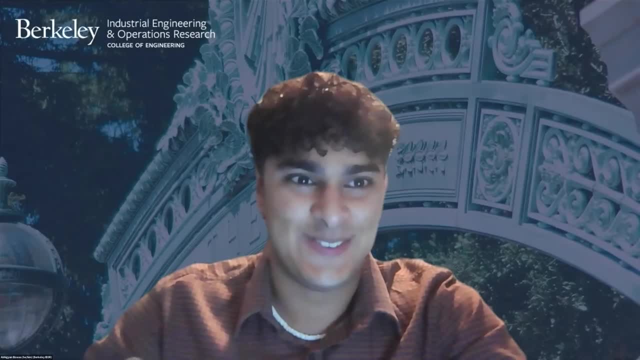 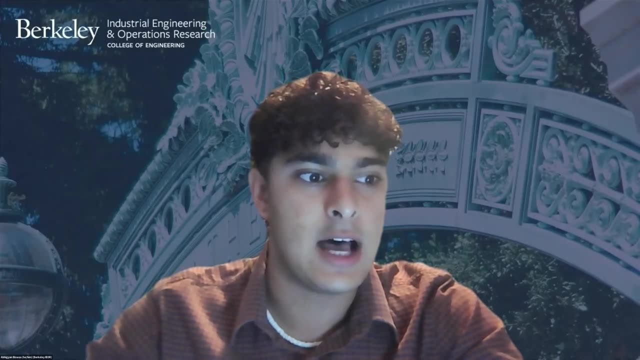 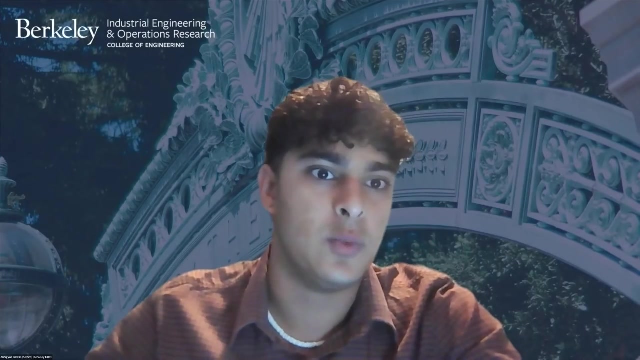 optimizations, which is kind of all of my interests, a lot of interests, I know, but IUR just blends them together so beautifully that it allows you to kind of build skills in all of those areas such that when you go out to the industry and you know the first year. 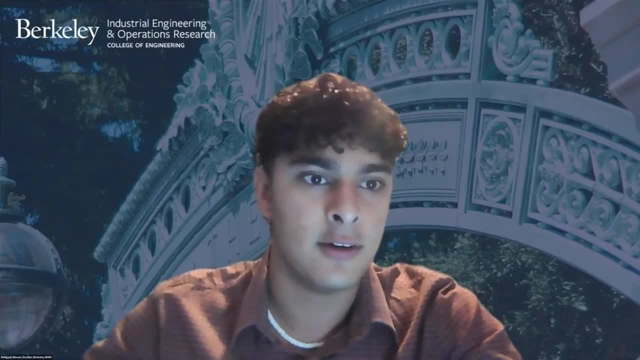 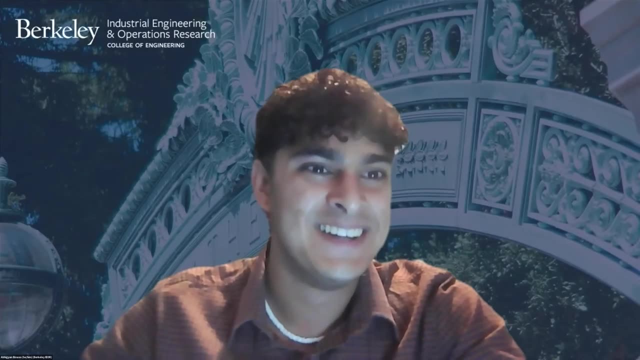 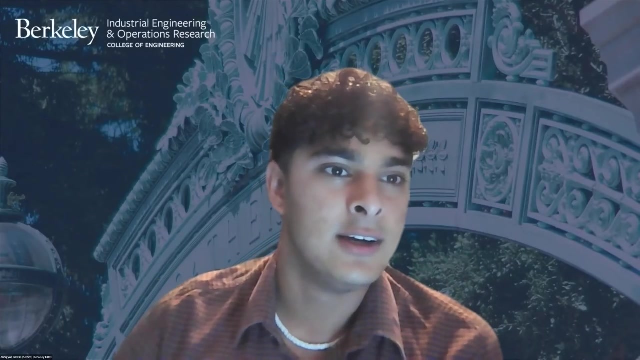 first two years you're trying to figure out where do I really belong. All those skills help, help propel you towards success, inevitable success even, And then I mean I think Professor Adam Turk elaborated on it earlier, You know. 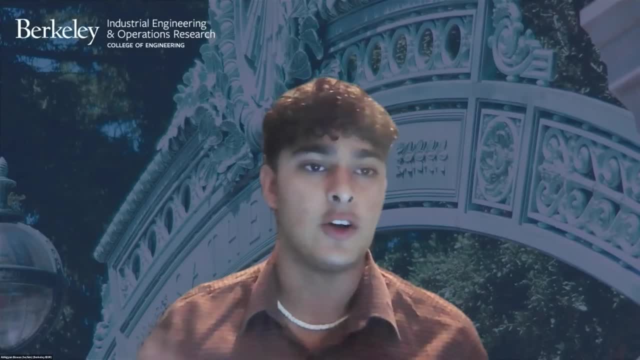 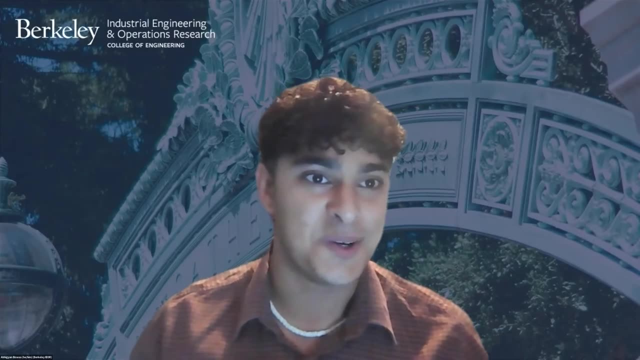 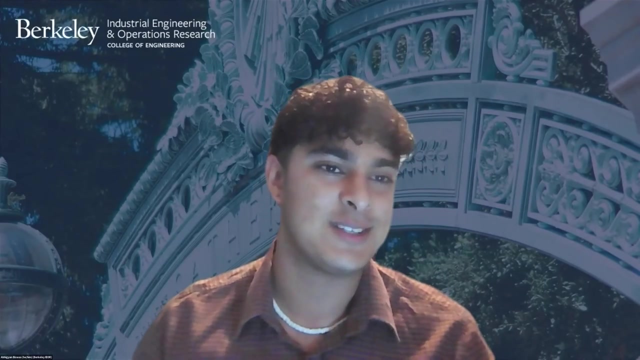 a lot of the things that we work with are have to deal with large scale systems, And in the modern world the large scale systems are so complex and so interesting And, you know, improving those even slightly can lead to like large improvements across the system And just interest in all of. 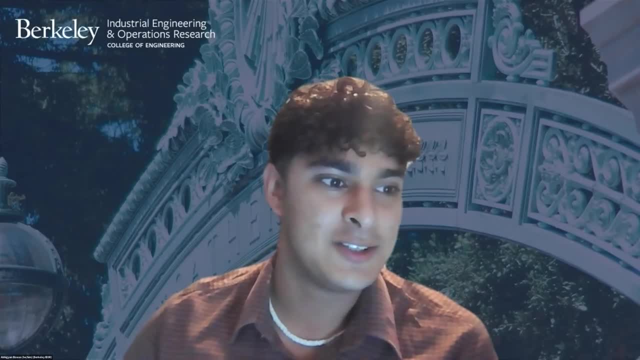 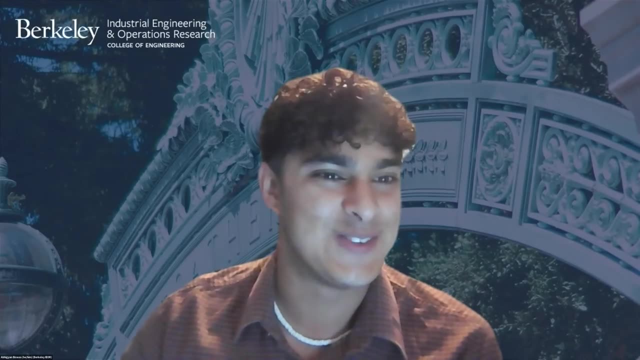 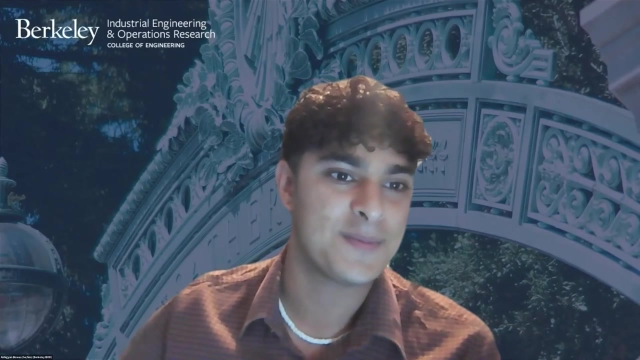 those different areas is kind of what drove me to choose IUR as a major. I used to be a mechanical engineering major before I transferred- full disclosure- but I am in IUR now and I love it. I absolutely love it. Thanks, Avi. Anybody else want to share? 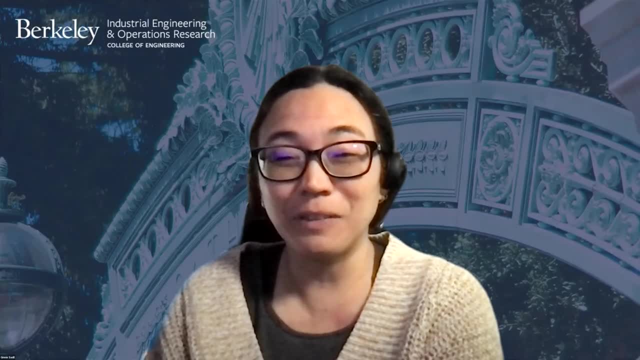 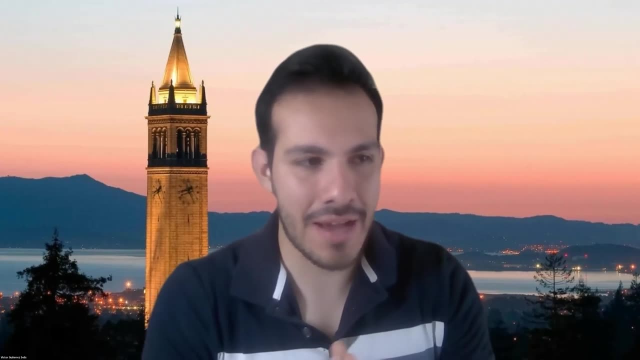 Or even one of our faculty, want to talk about why they picked IUR. I mean because you've you've dedicated yourself to it. at this point I can talk about a little bit of my experience. Okay, I'm from a foreign country. 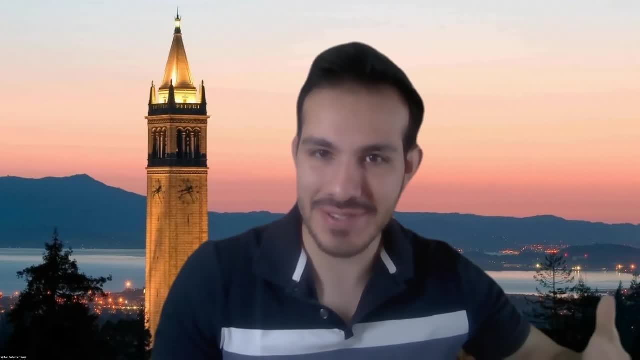 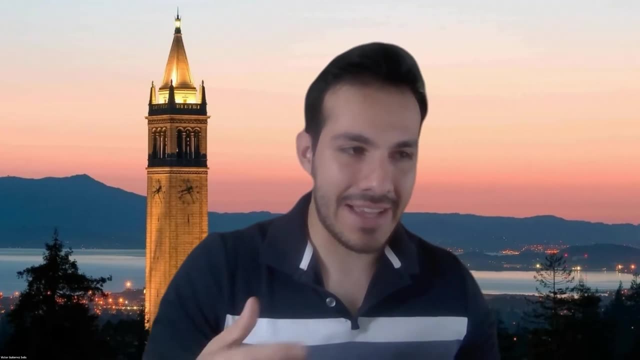 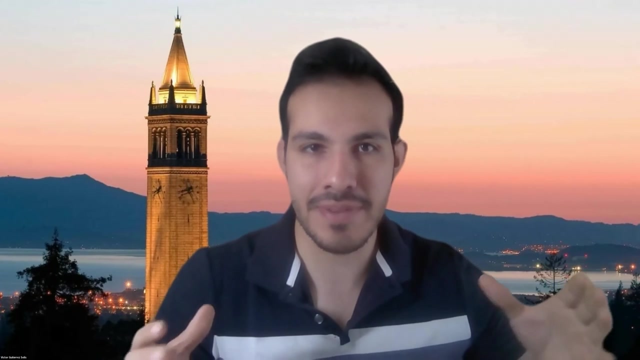 I'm a foreign country. IOR is a pretty common major to choose after you graduate from high school, So it was kind of a logic fact for me to follow it. But then I actually chose a major because something similar to what Avi was saying is: like it blends. it blends branches of the industry. 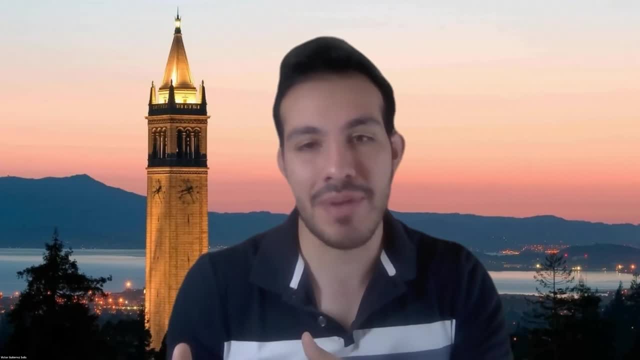 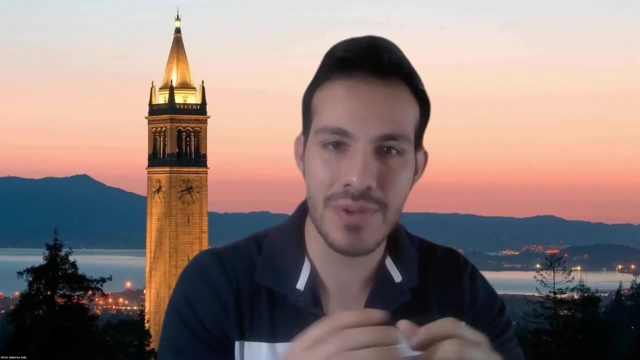 into something that is useful, like you have to use math, but you also have other skills that help you to like relate to people. you are not like all technical and stuff. you also have other skills that are really useful in the industry and i really like that about the major. honestly. 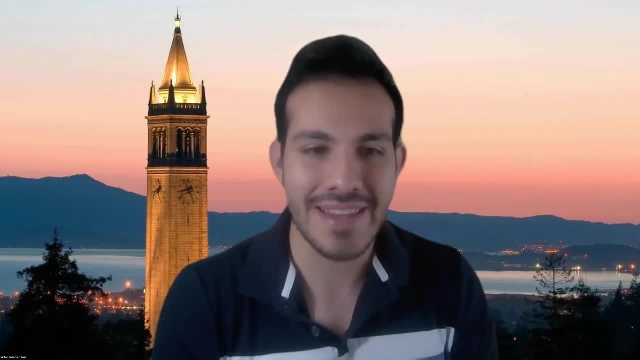 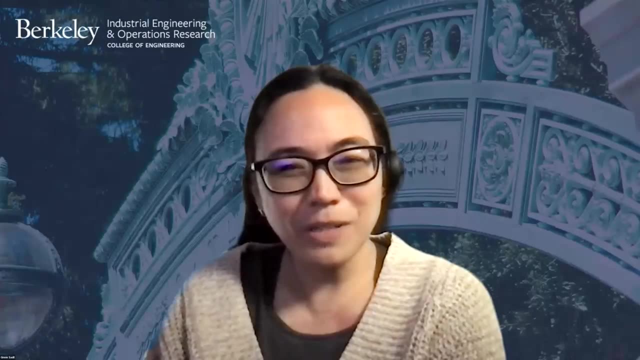 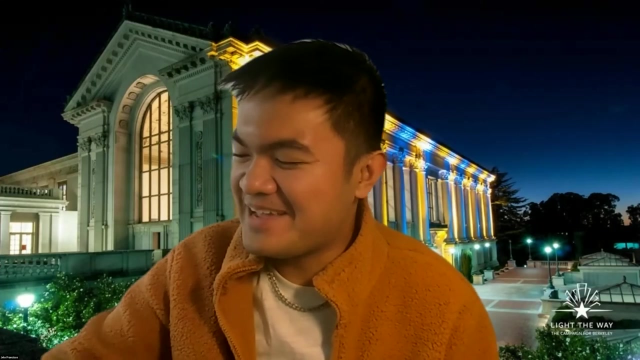 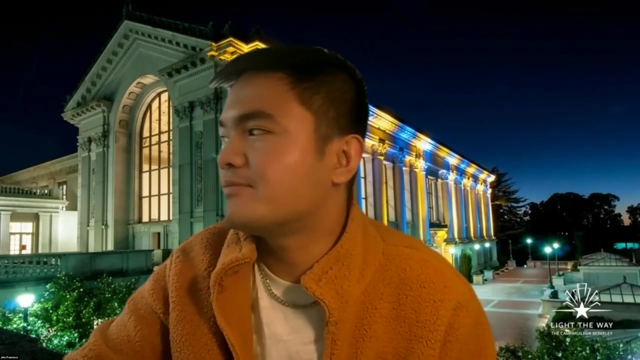 like how blends a lot of areas into something that is really really useful. great. what about you, jello? they kind of stole my answers, okay, um, but yeah, it's very similar to what they said. um, i love that it's very interdisciplinary, um, that i could go to data science or business or operations, or. 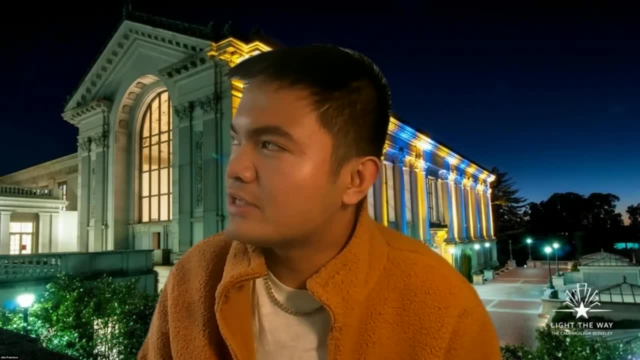 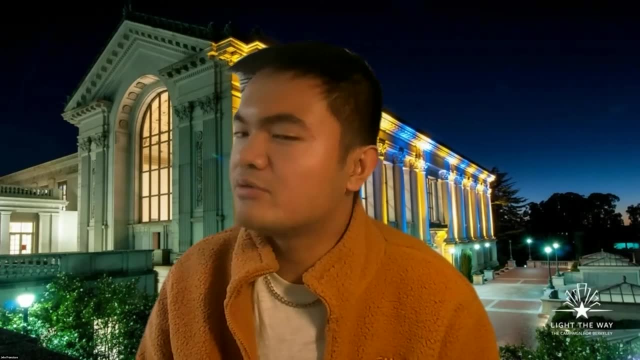 engineering, uh, but i think what really attracted me to iowa in the first place is, um, how i grew up, you know, with limited resources and so, like i just grew up being very resourceful, trying to optimize my life, you know, finding the shortest distance to walk to some place or 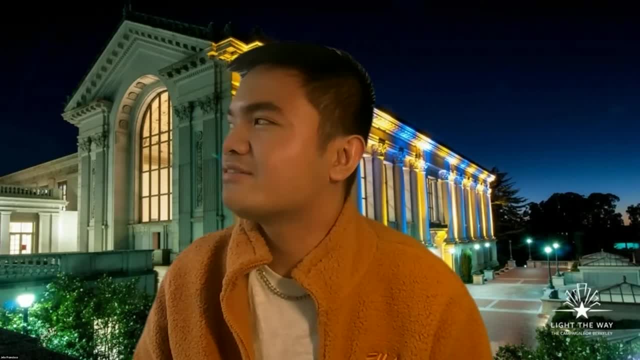 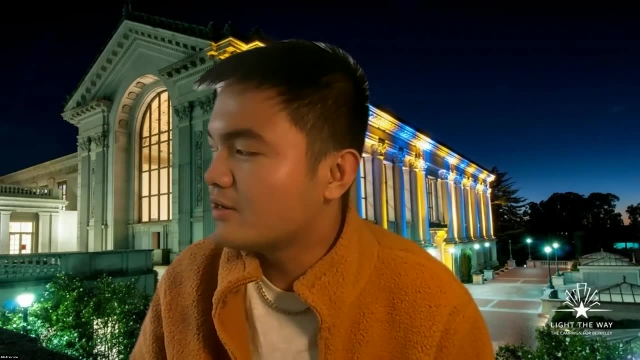 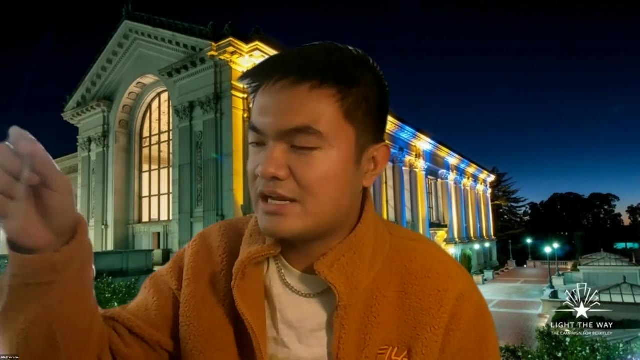 finding the cheapest great food in a city. so like those, um, those little things just built me up to be an iowa major and i chose berkeley ior in particular because i was looking at the classes that they offered and all of them really seemed interesting and, like professor adam turk was, 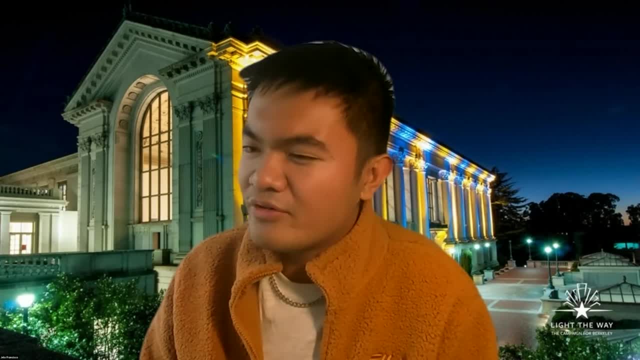 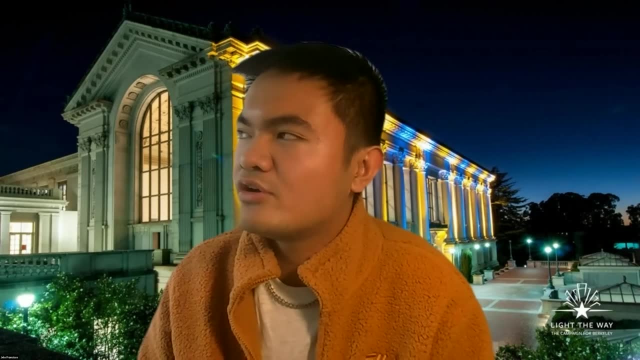 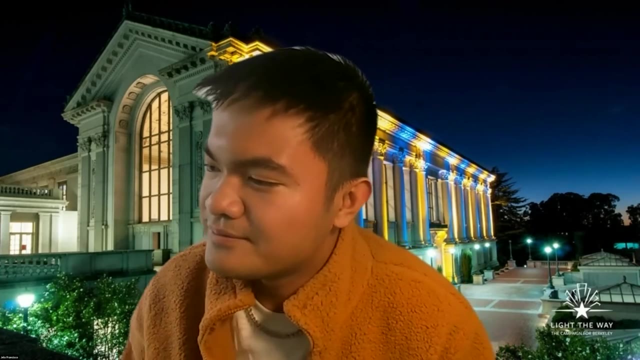 showing all of them. and, like you could take a lot of classes, you have more flexibility than most engineering majors, because other engineering majors are required to take specific classes, but, as i or that, you can take six electives that you choose on your own. so great, what about you? sujong? absolutely. i'm going to share a bit of a small anecdote before i even 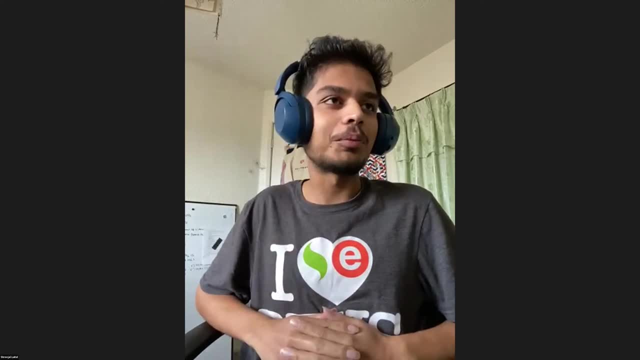 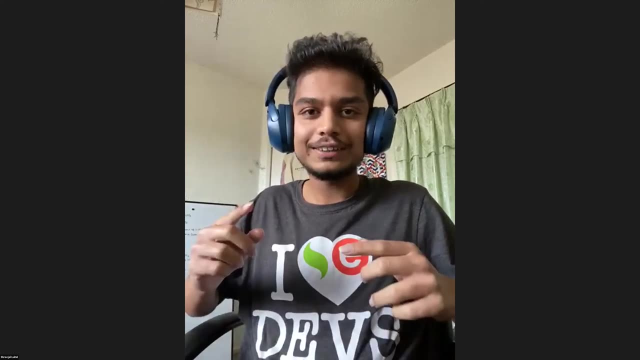 answer this specific question, but it definitely connects uh with uh. it definitely connects with, basically, my response. you know, whenever i cross the street, it's quite funny- i always try to cross uh and and you could imagine, like a triangle and that intersection it's, i think it's called. 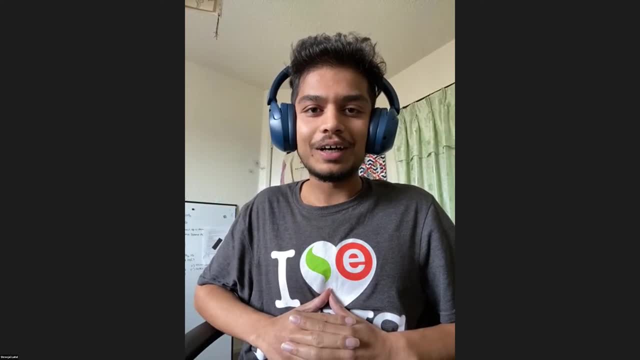 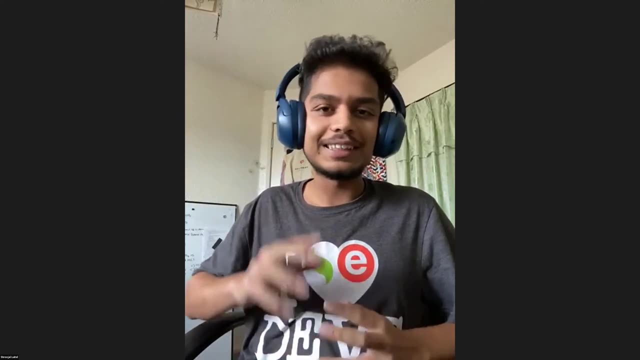 a hypotenuse. it's been a while since i actually looked at, uh, a lot of uh, you know, like geo, like geometric math, but it's, it's always funny whenever i cross the street, i started realizing, uh, that i cross it in a hypotenuse. and one day i was walking with my friend preston and i tell him: you know if? 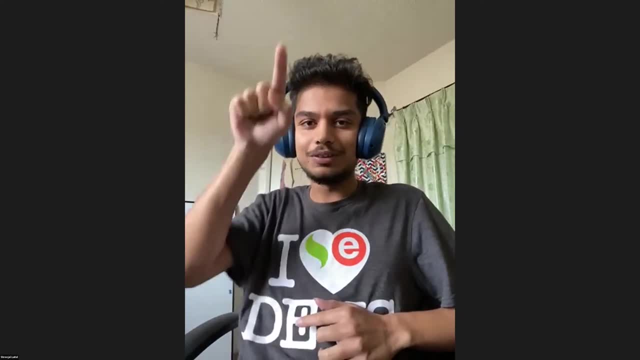 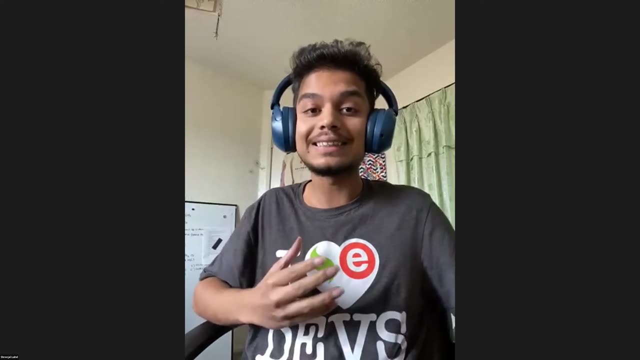 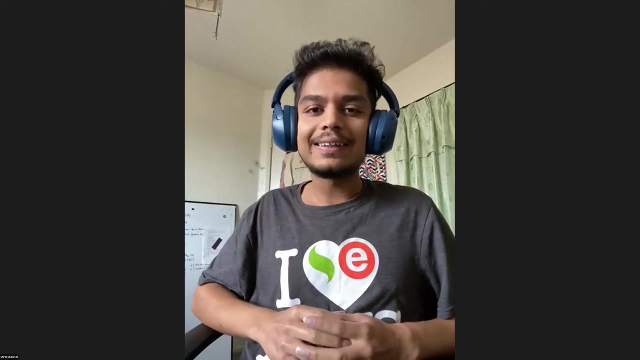 you, if you go all the way across and then you go like that right in, like an l shape, it basically, uh, cuts down on that optimization. so, frankly, i've been doing it since high school, uh, and and now when i think about you know, going to a different university, i think number one- the fact that it's 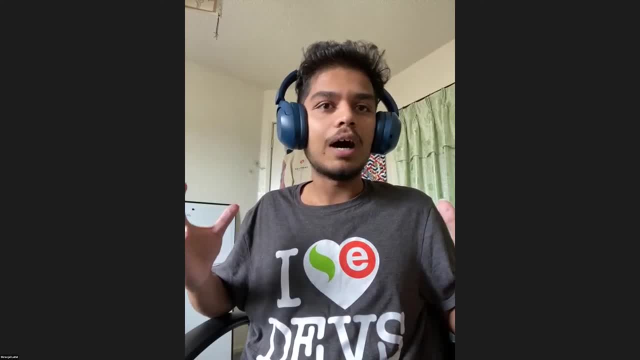 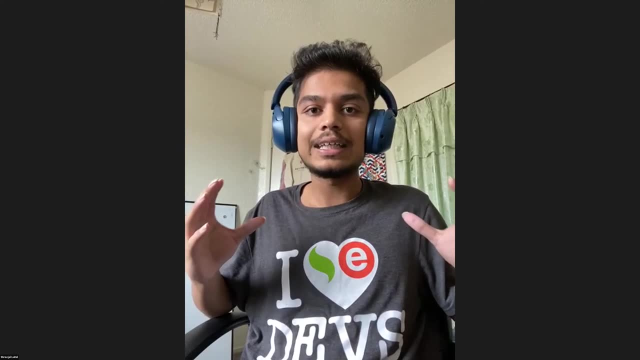 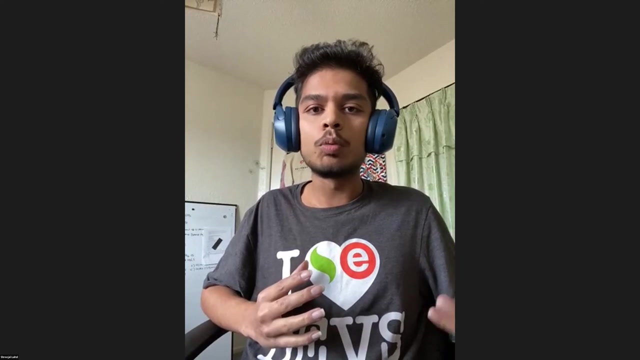 interdisciplinary and it blends in so many different, uh, fundamental principles, not just within engineering, but within within data analytics, within within statistics- right, i think it allows for you to become more interdisciplinary and that, in turn, helps you create and design more efficient systems, right, uh? so i think that's that's really, that's really key. here is the fact. 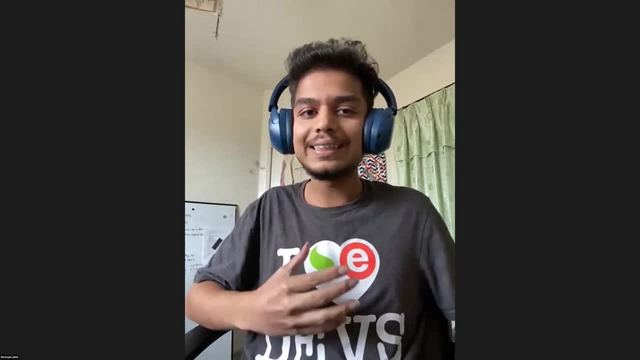 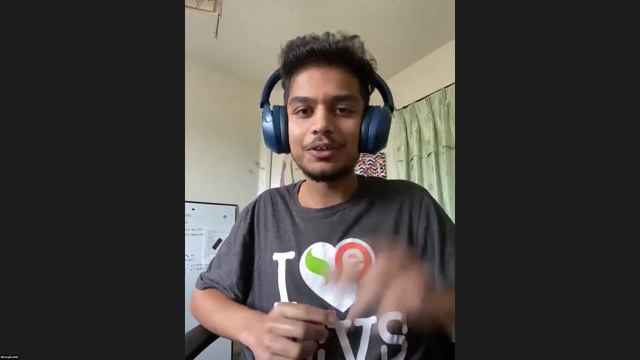 that it's interdisciplinary, because i'd rather be a jack of all trades than than be a jack of uh one trade. you know, i that's the first time i probably uh said jack of one trade. i don't know if that's actually a key term, but uh, definitely. 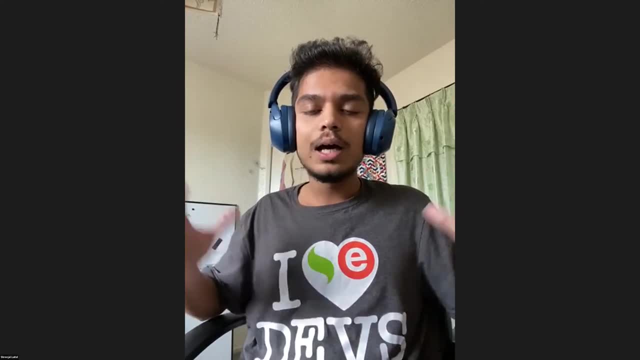 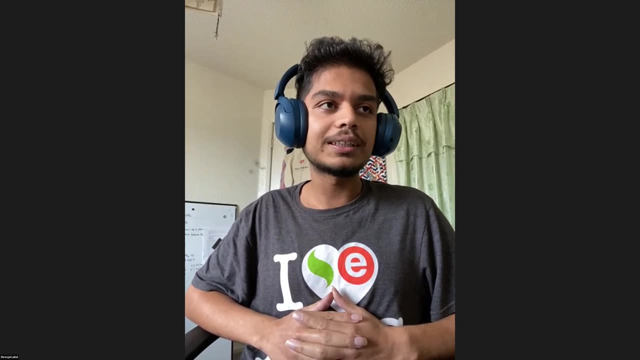 you know, i definitely want to be someone that that's more branched out, uh, because it allows for greater flexibility. right, and that's something that everybody here has been echoing. uh, number two, i think it's important to consider that uh outside of the prestige, within the berkeley. 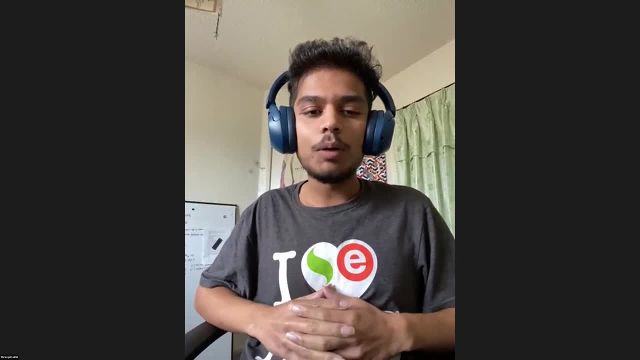 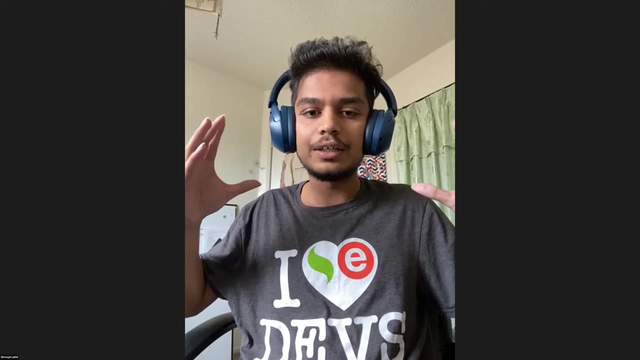 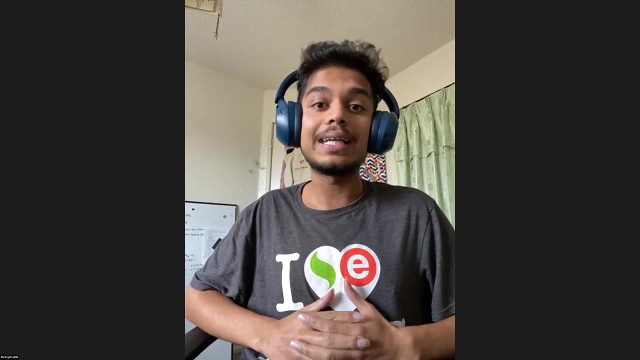 environment, uh, the fact that it's niche, right? uh, when i say niche, i'm talking about a very uh, a very small department, um, and and that allows for greater opportunities to frankly just network around and and and find more people. uh, it's, it's quite funny, you know, in in my day-to-day classes, uh, i see so many of uh people from like one class. 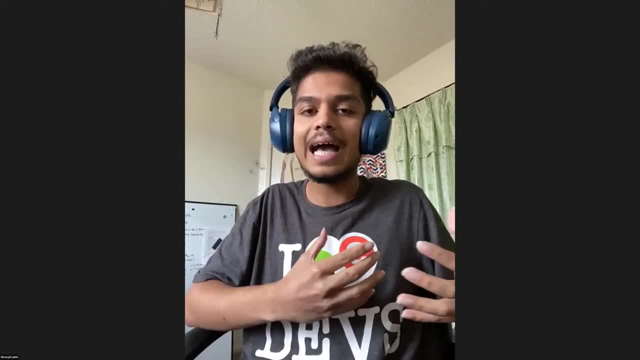 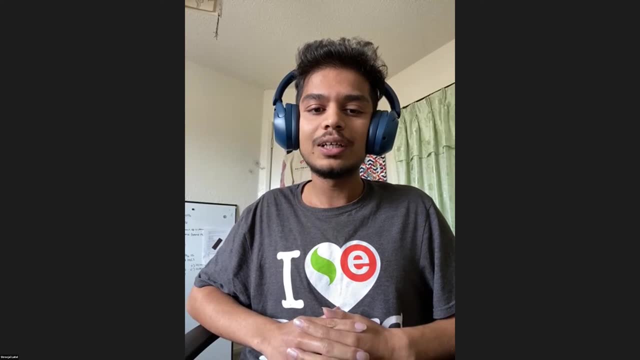 to a different class and that allows for people to kind of bond and actually form relationships right. whereas if you go into electrical engineering, for instance, there's so many people within that uh that it creates. it doesn't allow you to kind of develop like long-lasting and forge these. 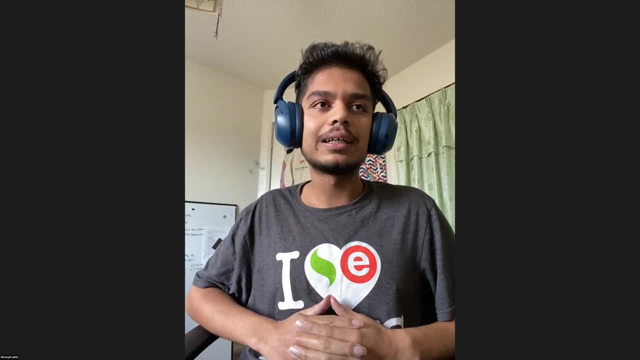 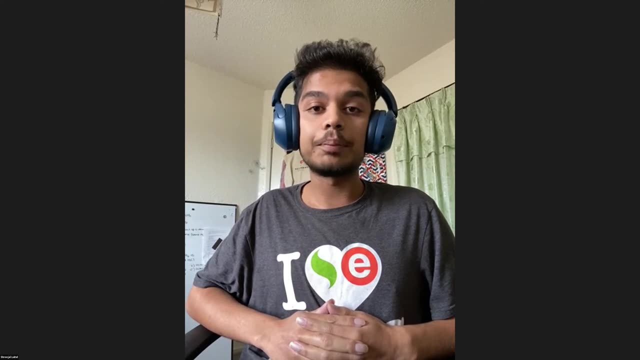 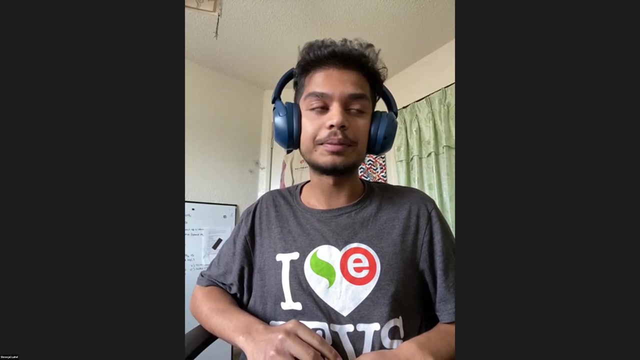 long-lasting relationships, right, uh. so i'd probably say like the, the combination of those two uh kind of propelled me within iur uh, like specifically at berkeley uh. but it's fundamentally it's about, uh, it's about optimization, because i've always thought about optimization, uh, and taking formal. 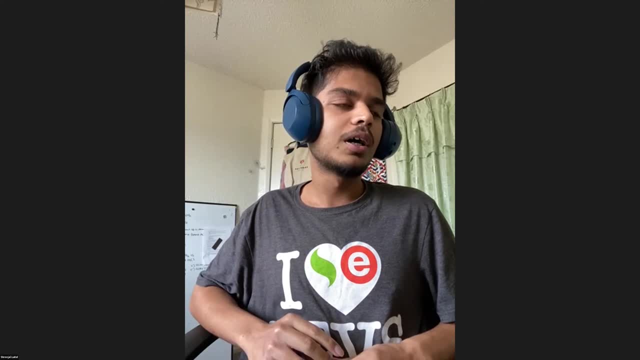 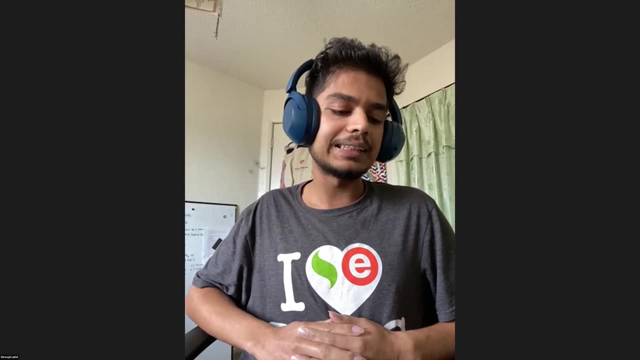 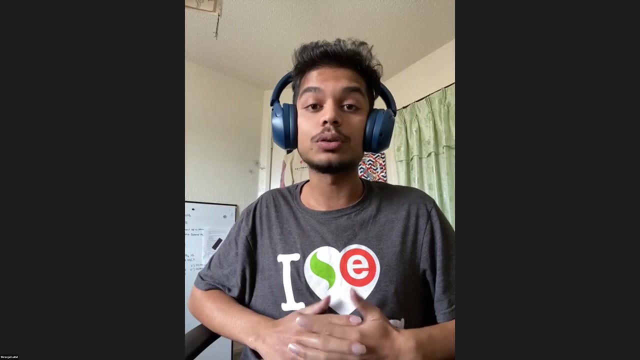 courses on. it is really imperative. and and number two, it's also about understanding and and having like an interdisciplinary approach to problems that you want to tackle. um, and number three, lastly, it's about: it's about, you know, like a very niche- uh, niche- segment, you know, and and trying to forge relationships and actual, like actual bonds with. 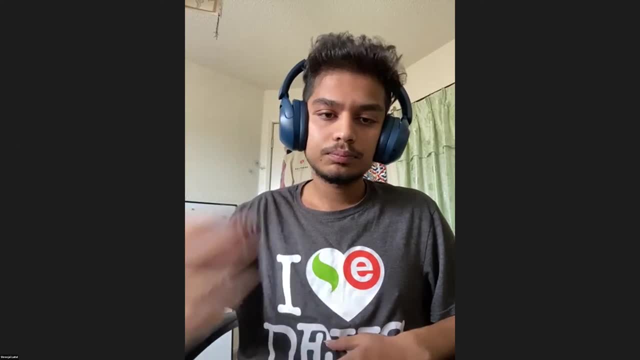 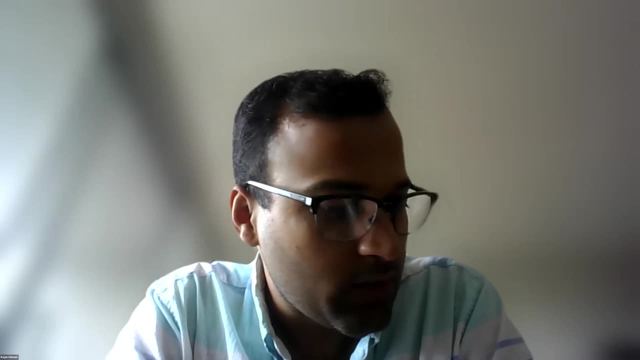 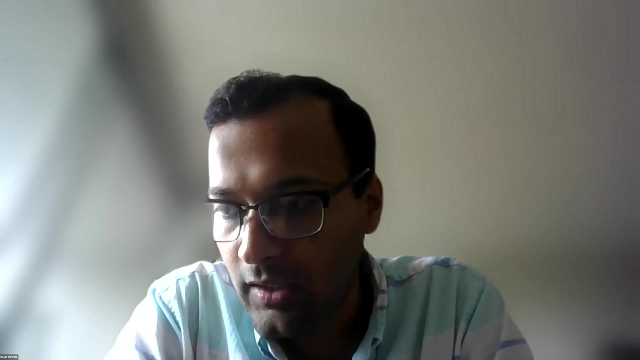 with different people, right, um, you want to go, and then sure, um, i guess. um, i can maybe just essentially add to to the answers that, um, i have already come out. so, from the research point of view, the reason I guess I'm an ior faculty as opposed to. 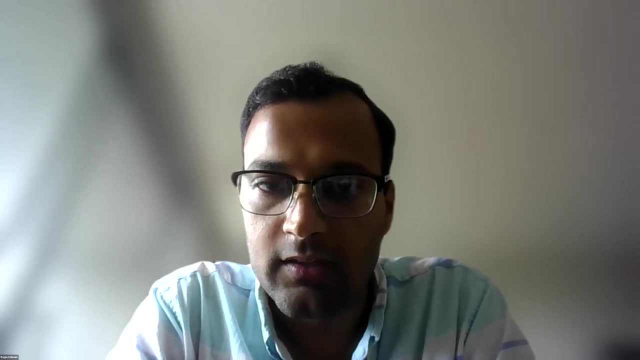 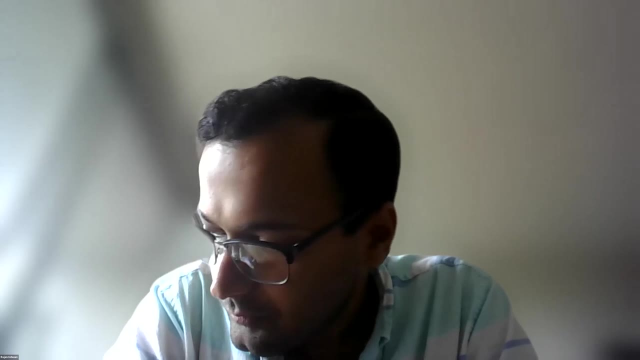 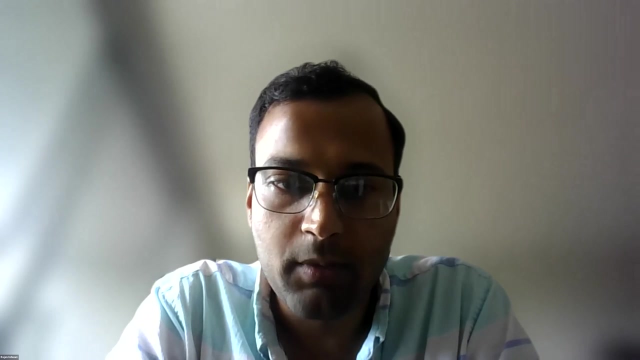 something else is because, um, I like math and and ior gives me, I guess, an opportunity to um kind of think about mathematics with an application in mind. and then, I guess, from the educational point of view, my undergrad was in electrical engineering and then I did a PhD in. 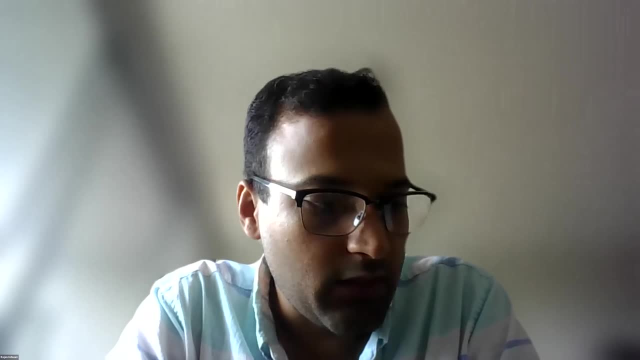 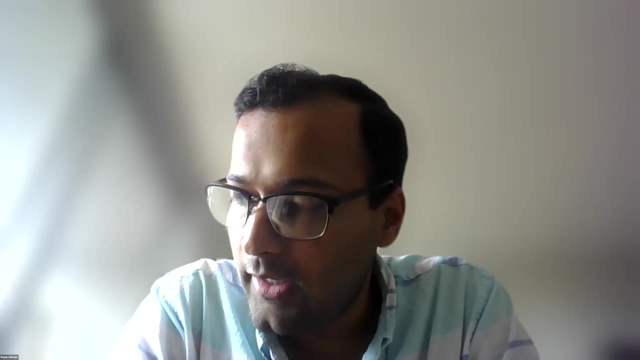 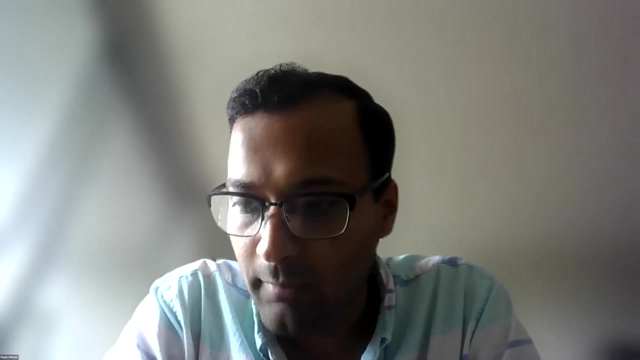 operations research. so, uh, my sense of the main difference- since that was something that we just thought, why you should take this versus that- is that basically um or or ior, uh kind of. is uh going to have you think about um concepts in in optimization, statistics modeling software. 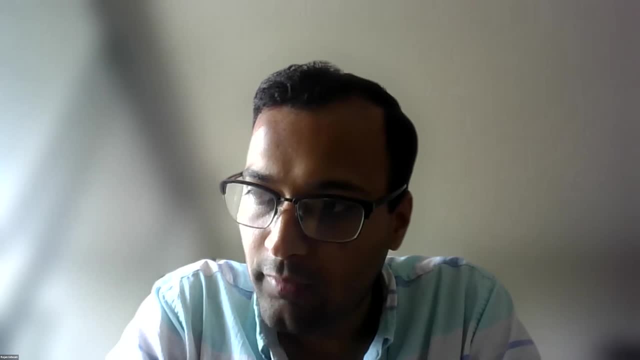 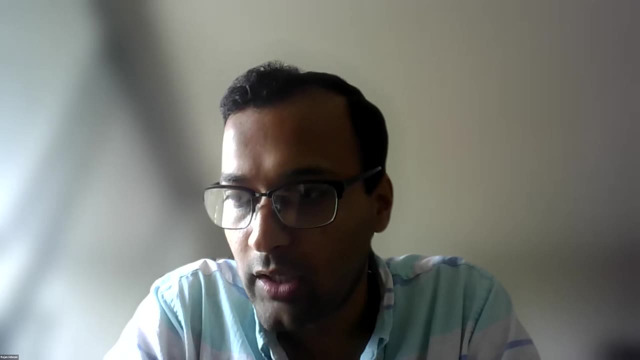 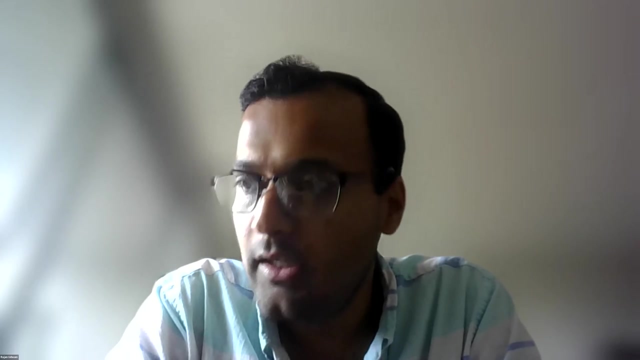 algorithms, Etc. but from sort of an industrial perspective that you can perhaps have pick and choose. okay, what kinds of industry you want to Target? do you want to learn more about supply chains at Amazon, Etc? do you want to learn more about health care, Etc? whereas um, EE and NCS, uh, focus on hardware and software. so Industries that basically, either. 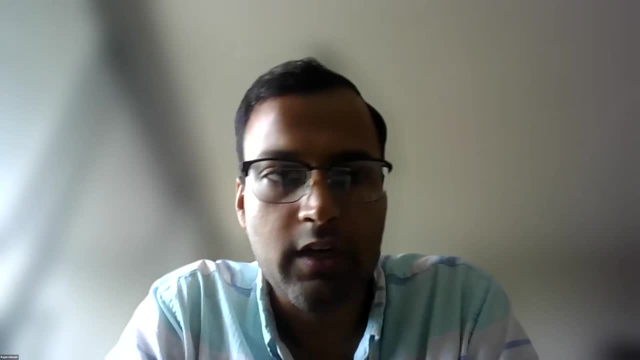 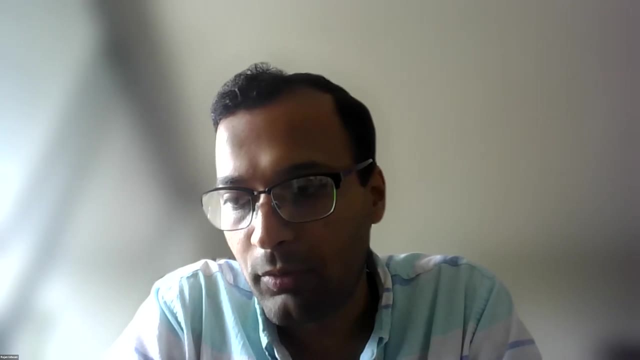 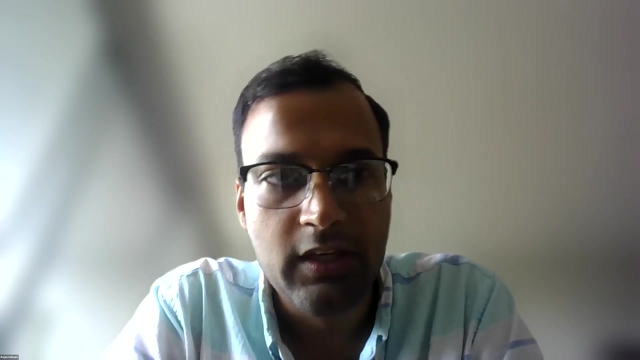 want to write large-scale industrial code or circuit design, so so it's distinct, in my view, very much, even though there is overlap, from the point of view that we both care about algorithms. at the end of the day, we are living in an online, automated economy and growing more and more towards. 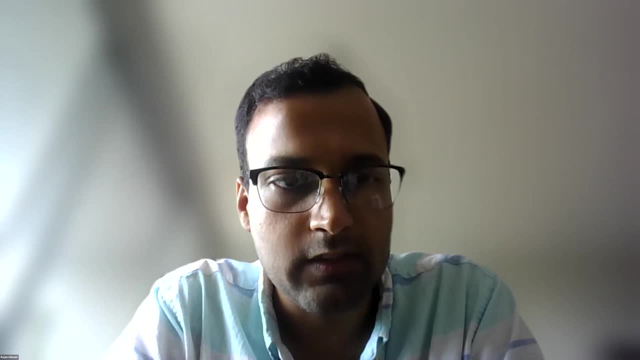 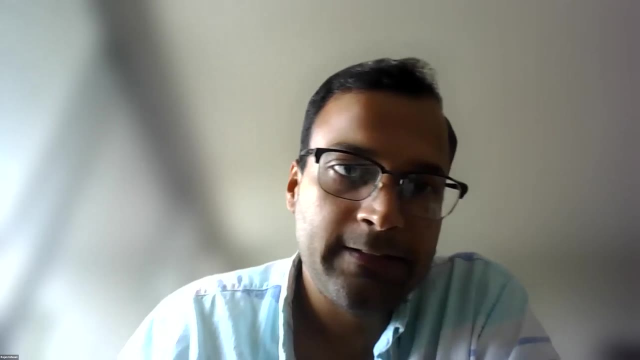 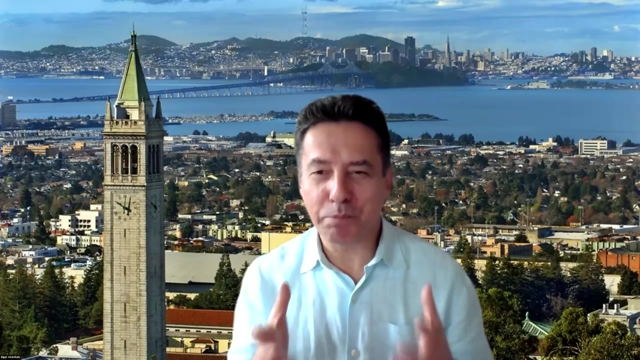 automation. but, um, I think the choice is very uh distinct, uh, even though people tend to think of uh it all as the same. um, that's, that's, I guess, what I would share. thanks, thank y'all. so for me, um, it was uh really about not being confined to a particular uh device development or technology uh development. I wanted. 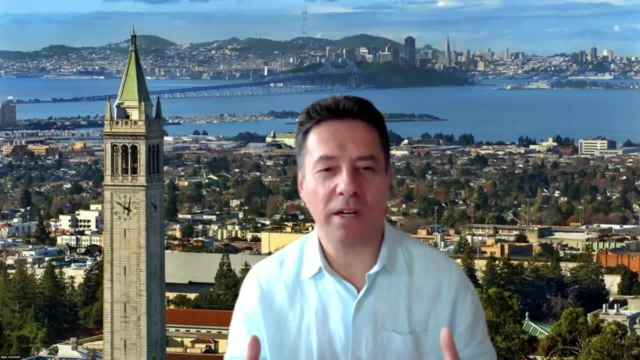 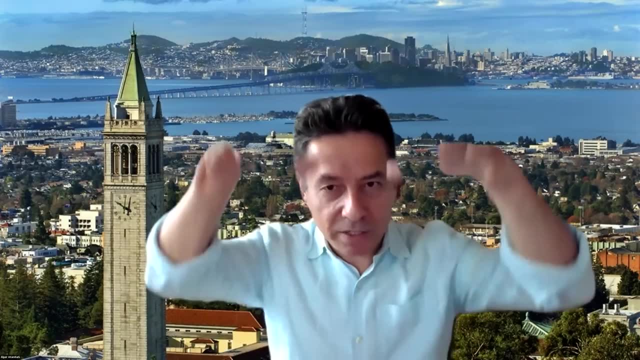 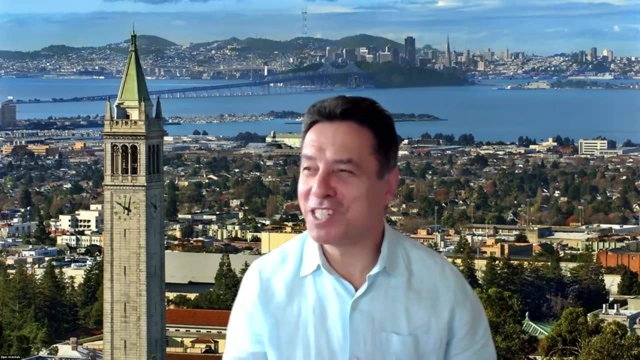 to be broader and I knew I wanted to be an engineer: um, um, um, but um. but I wanted to be able to have a sort of bigger sort of perspective picture, um, um, and I'm very happy, obviously, with the choice that I have. I've seen my uh sort of friends who 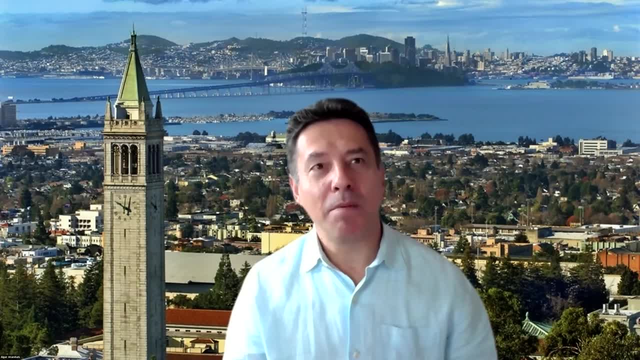 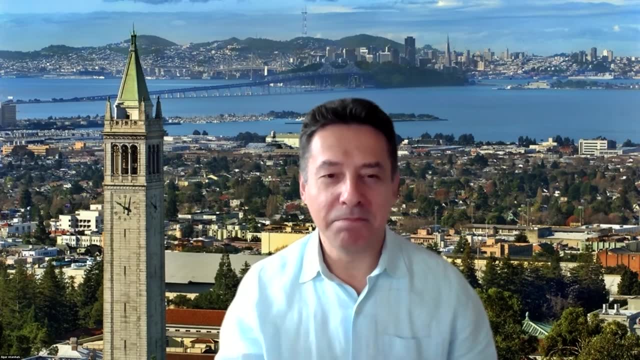 have gone to other engineering fields and and they have become Experts in a particular technology and device and, um and down the line, uh, that particular Technology has become obsolete, uh, replaced by something completely else. and they could have come back and say we would decrease its size and we now have a number. immediately, can you convert it into something completely new? they have the number would be half of the Championship each round and we can achieve ultimate profit. um, I'm very happy, obviously, with the choice that I have. I've seen my uh sort of friends who have gone to other engineering fields and and they have become experts in for a particular technology and device and, um, I'm down the line of that particular technology be completelyет by the officials. 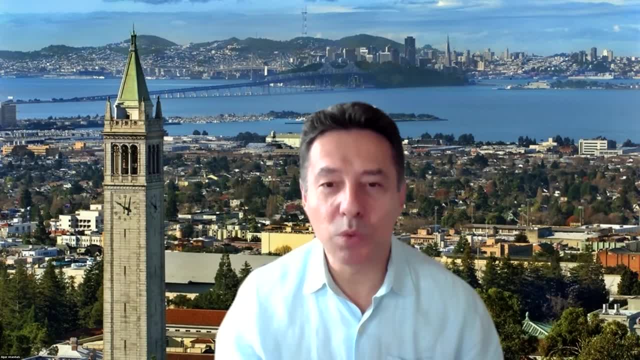 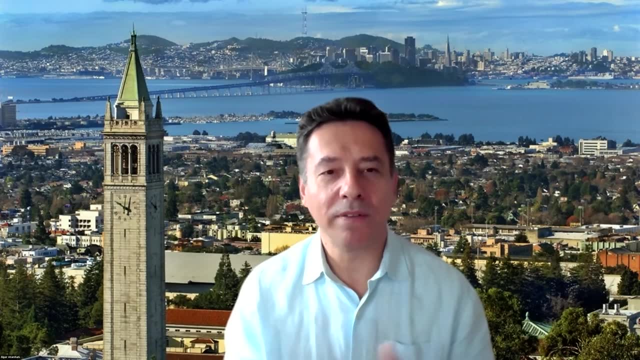 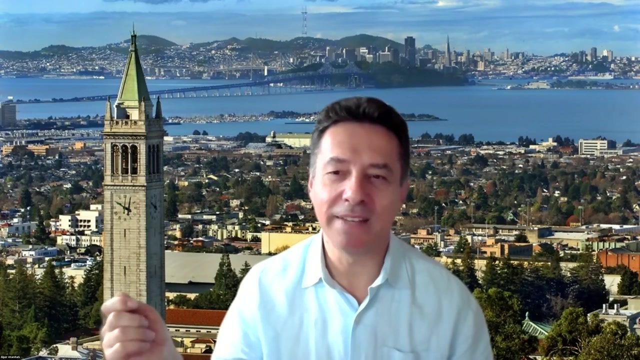 themselves in a very difficult situation in the job market and so that the resilience of IUR, the flexibility is, really has huge advantage over the career of a person and I've seen our students to even move from one industry to another quite seamlessly with utilizing the skills that they. 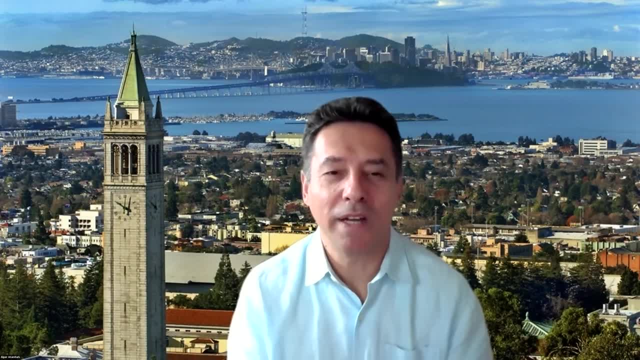 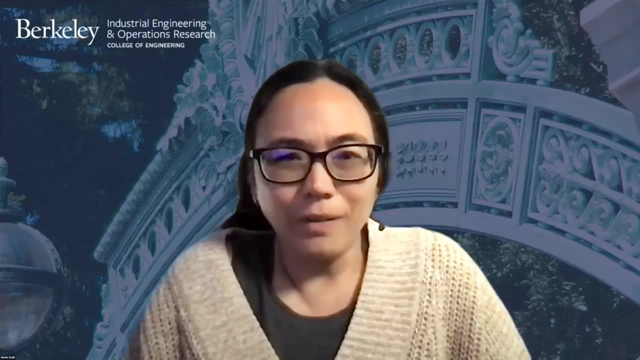 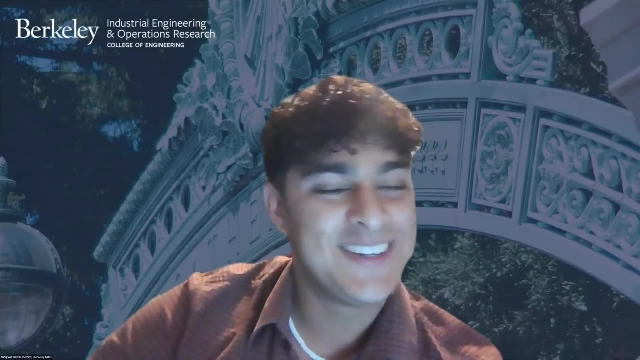 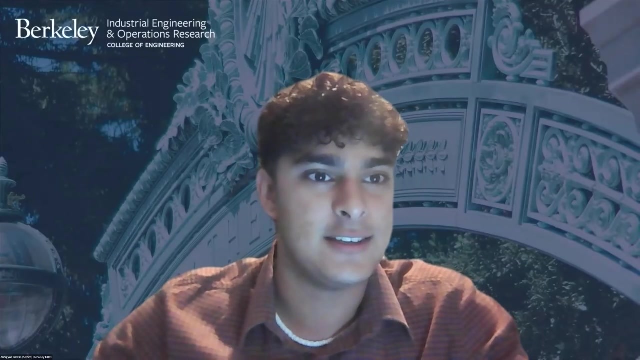 have that can be operated up, can be utilized in their industry. Thank you all. Abhi, you wanted to say something else? Yeah, I'll just add, like maybe like three quick things. just listening to everybody just reminded me to Srijal's point. yes, the IUR community is, it's kind of like a family. 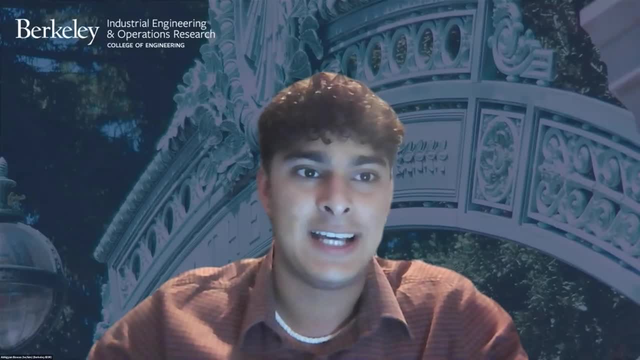 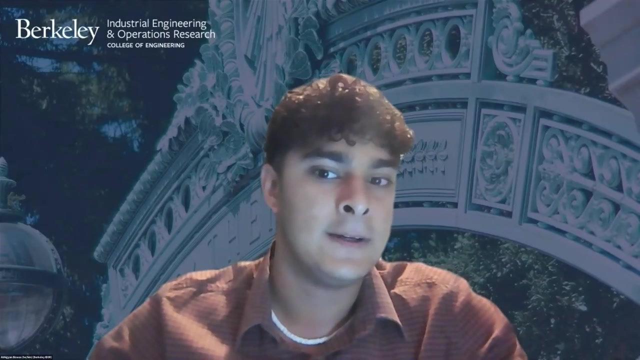 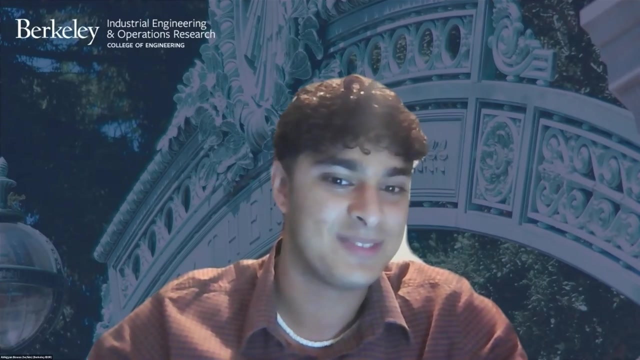 right, everybody knows each other, everybody has met each other, everybody to some extent hangs out with each other and it's a close-knit community that's here to support you. right that I feel a little bit different from the other majors because they're a lot larger and they have a lot more students under you know. one like trying to. 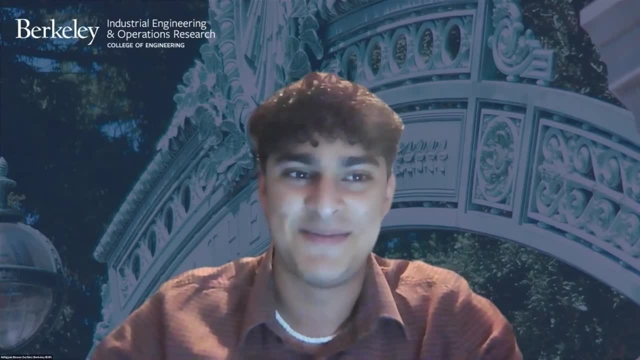 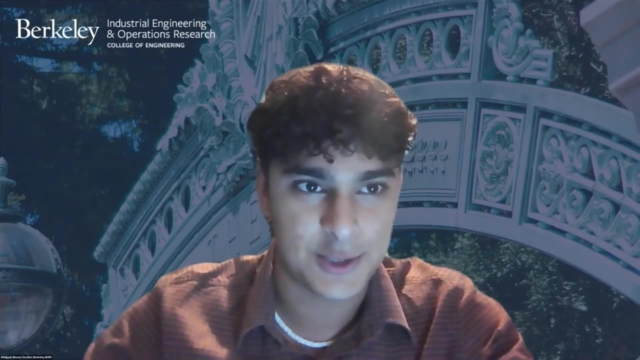 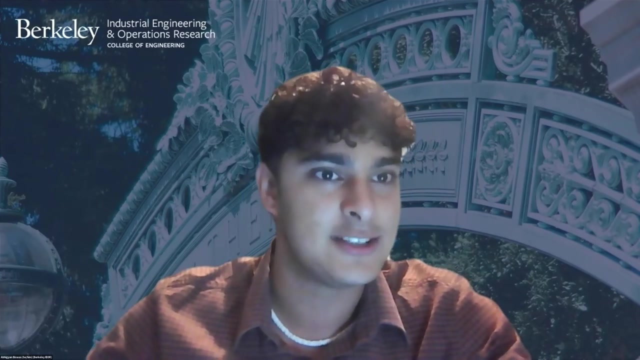 organize together, whereas in IUR we're able to organize more efficiently and optimize our social interactions and professional interactions. and on that note I'd like to plug ISC at Berkeley. so if you do end up coming to Berkeley, please join ISC. ISC stands for the Institute of Industrial. 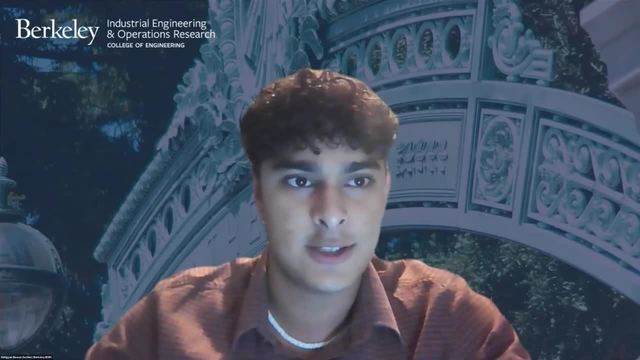 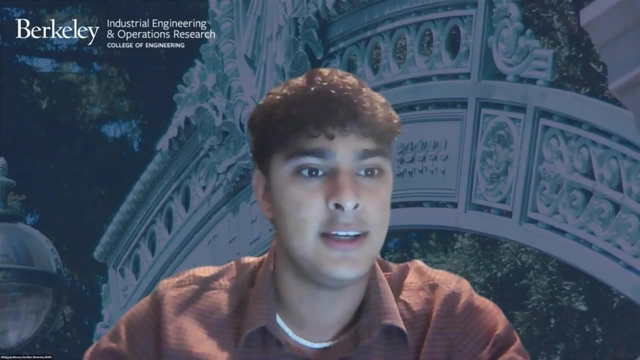 and Systems Engineers here at Berkeley. I am currently like a VP there and it's a great community and we're all here to support you. you're able to, you know, meet with professors, meet with staff. we have a big culture center and we're able to have a great time together. 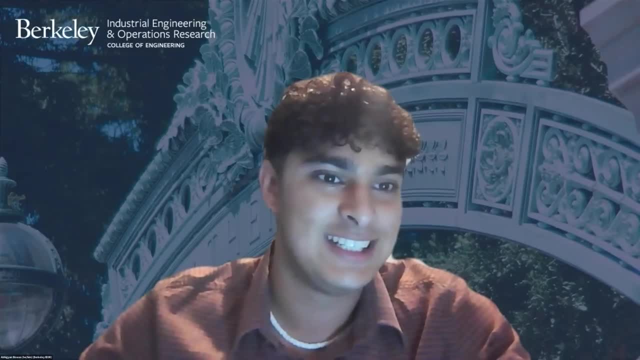 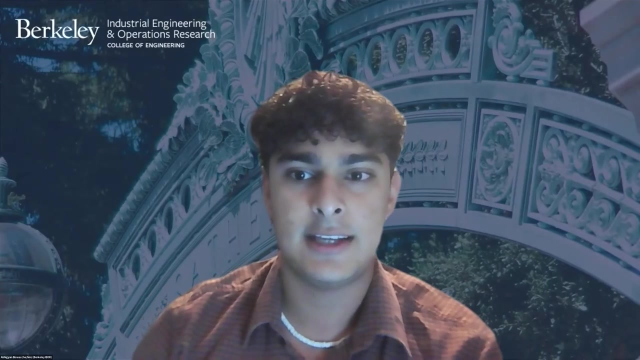 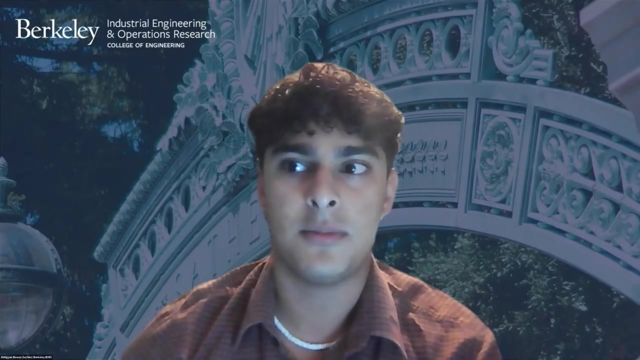 Thank you guys. Thank you an amazing talented crew of professors and an amazing talented crew of staff who help us, including Ginny and Goldie. so that's just one point that I wanted to make. another point is that one of the things that I don't know if we have discussed yet is that the Berkeley IUR program. 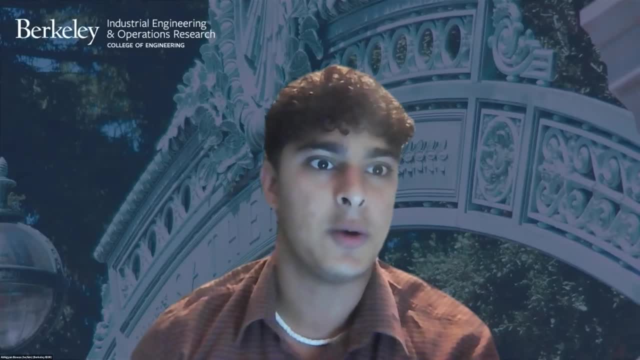 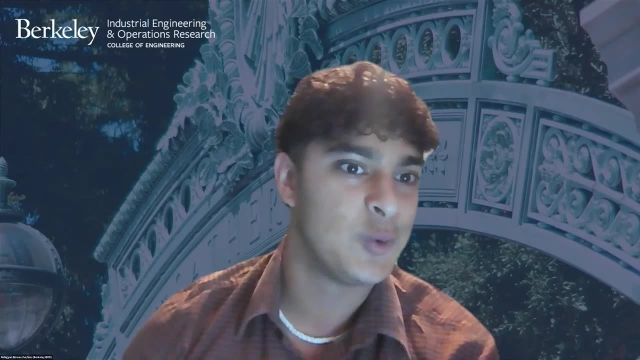 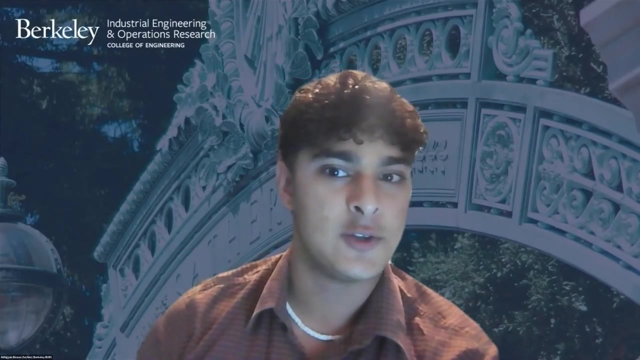 is the Berkeley. Berkeley in general, but also the IUR program, is one of the top programs for startup founders and which is another reason why I chose Berkeley IUR is I'm really passionate about entrepreneurship and and innovation and looking to what is the next big thing that we 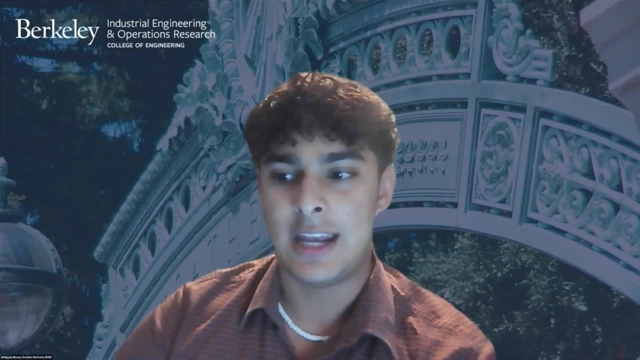 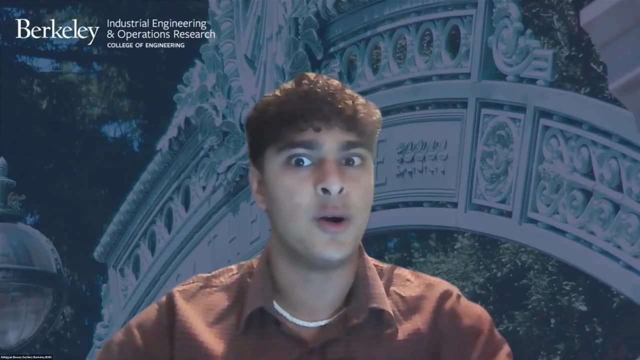 can develop, or what is, you know, the next industry that we can change and, you know, make more efficient, and- and I think that's one of the things that I'm really passionate about, and I think that's berkeley iur- really helps develop those skills and lets you get perspective into how to change. 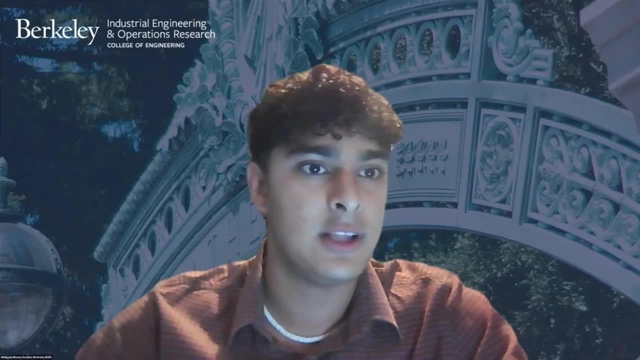 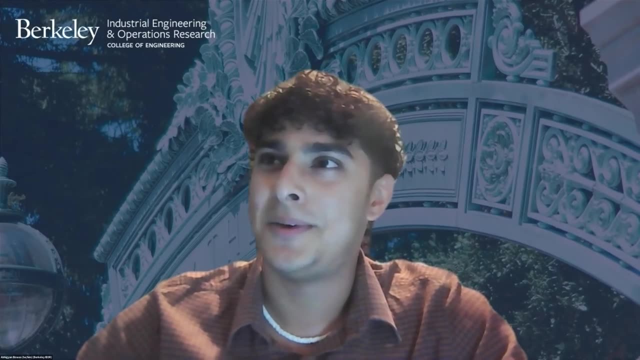 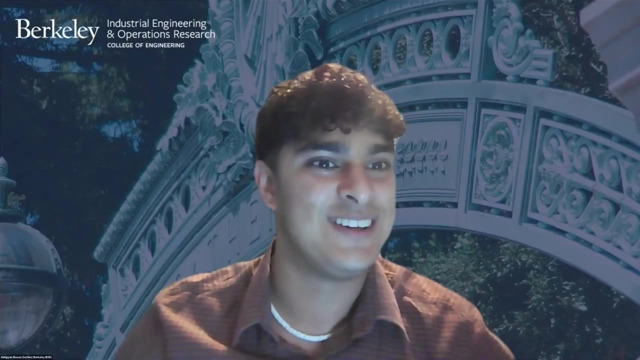 these industries, um, from a fundamental level, from a technical level and and from an operations level, right, um, and what was the third point? uh, i, i, i think i forgot the third point. but well, that's, that's all for now. yeah, thank you, i began. the first two points were amazing. 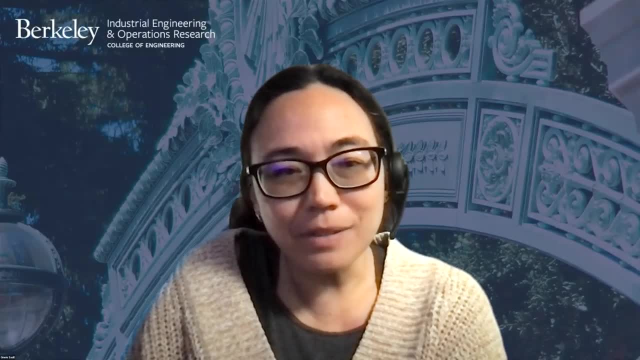 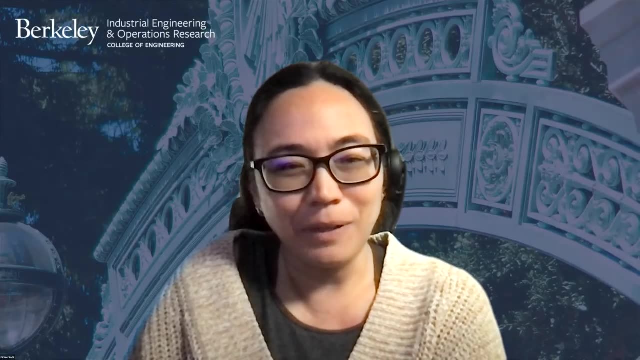 so i want to open it up to questions from our um, from our students, um i. you can either put your question in chat if you don't want to unmute, but if you want to unmute where there's a um, we have uh, there are enough of you and enough of us to answer questions that you might have um. 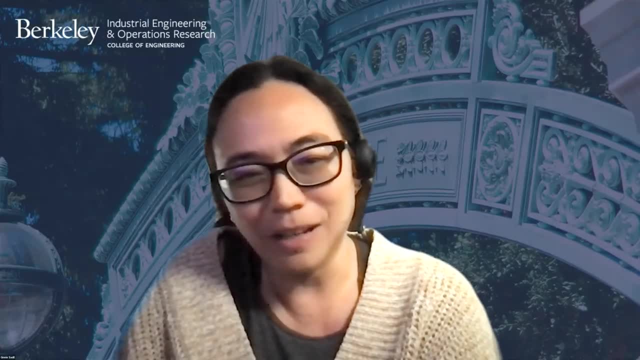 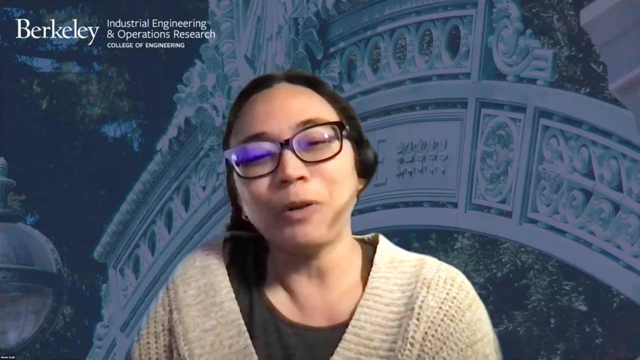 you're welcome to either to say it out loud or to add it to chat and um, we can get your questions answered. this is the only time you're going to have this many- uh, two faculty and four students before your admissions to berkeley to ask any question you want about the major. 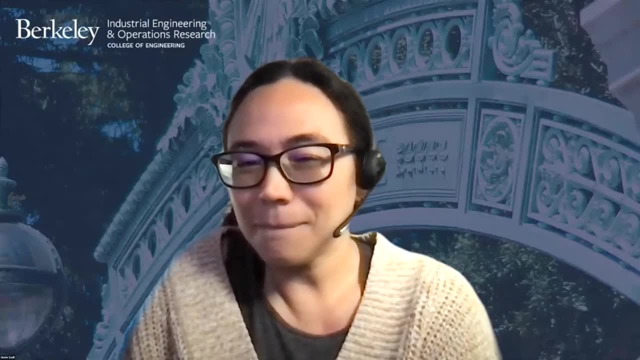 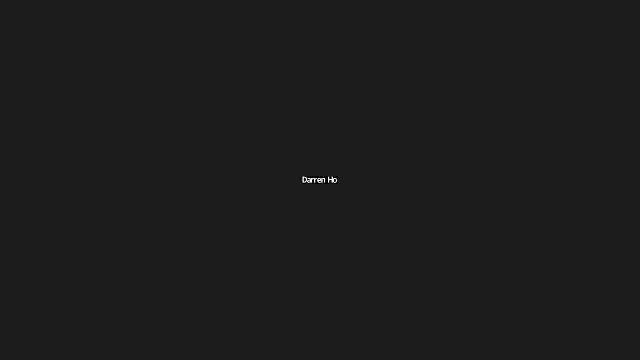 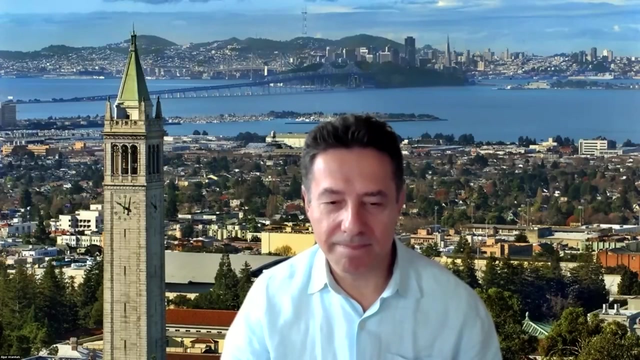 um, yeah, i guess i have a quick question, um for someone who's interested in energy systems. can you guys distinguish, like, what would maybe be the benefits of majoring in io eor versus, like, electrical engineering? sure, i guess? uh, i could like maybe expand on that question, um, for someone who's interested. 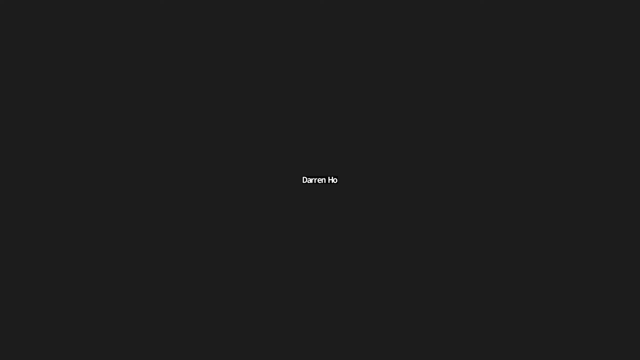 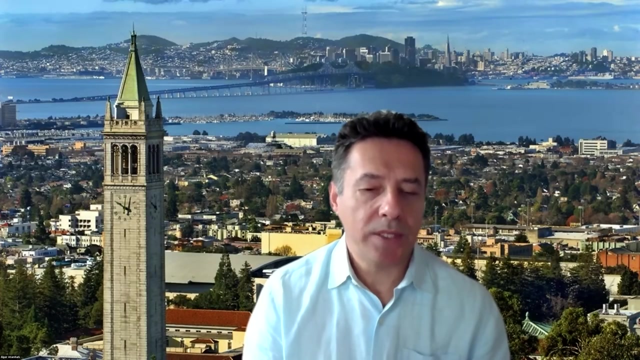 in like power systems, uh, like operations and optimization of you know, like integrating renewables and storage systems and renewable technologies. great um, for for these interests that you just mentioned, all right, so some system levels of power, um, how to, how to design and operate power systems efficiently. iur is a great, great, major um if you're interested in building devices. 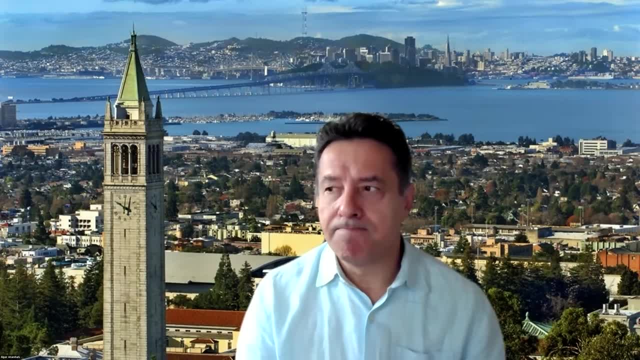 that go into the power system, right um? eecs may be a great major, right, but if you're interested in how to run these systems, uh uh, how to make, how to uh design a grid, right um, it is. iu are exactly the right major to do that. many of our students um. 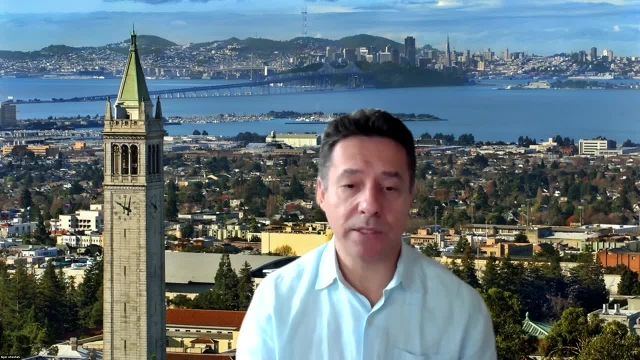 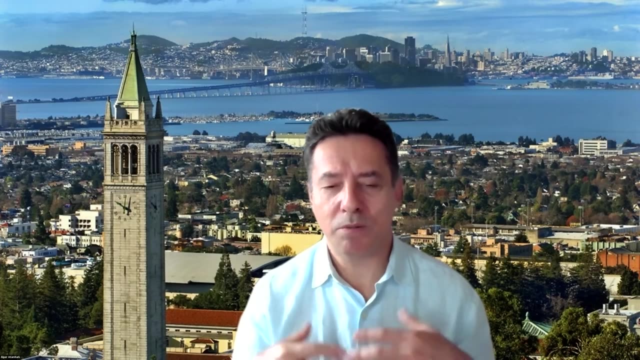 work in at utility companies, uh, pg, any courses that serves the bay area. they have a crew of operations research team that they do where they do research on- uh you know, on on pricing of electricity, on where to manufacture, when to manufacture, what kind of resources to use to 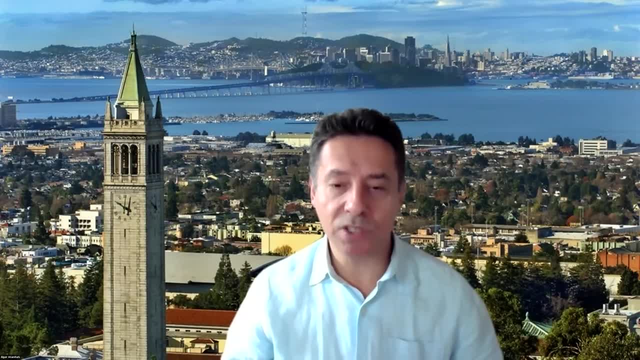 for the supply and demand is that isos independent system operators hire our students and and our faculty uh work at isos, as is on their advisory boards, as consultants. um our faculty have grants from the department of energy. uh, uh and, and you know, participate in various competitions. 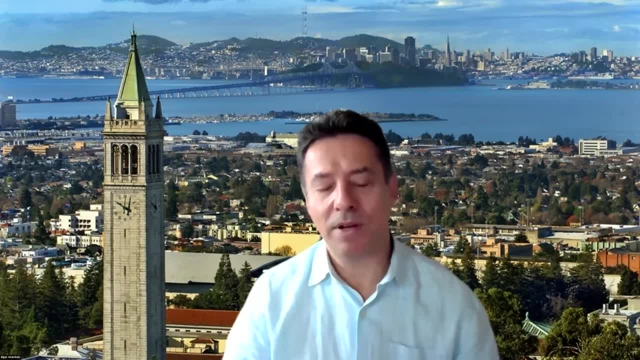 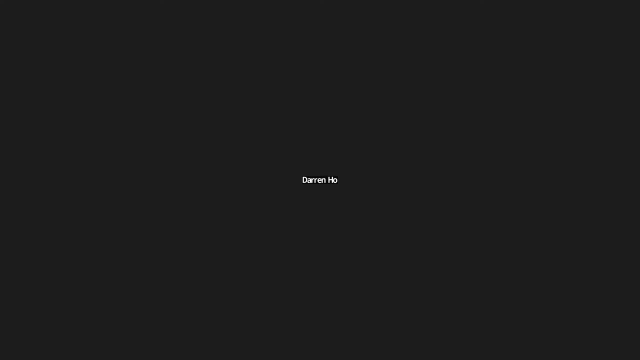 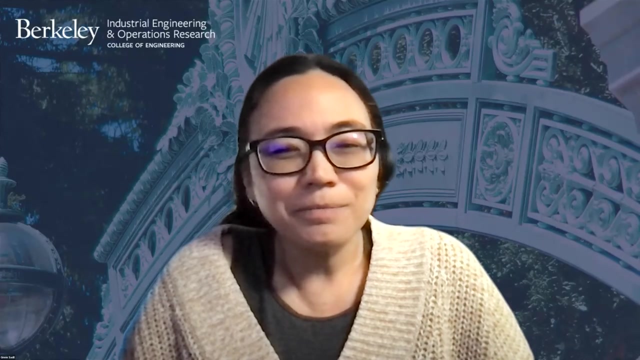 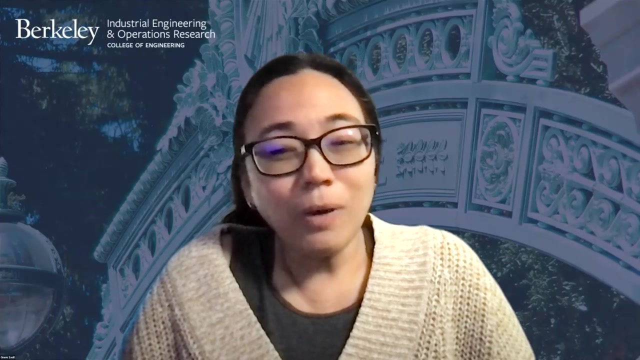 in this area. so it is a highly active uh uh branch. i would say power systems of uh iu water cup field would be a great choice. thank you, thanks, darren. anybody else any other questions about the program, about berkeley, about being a transfer, okay, well, how about? oh, here we go. um, we have a question about 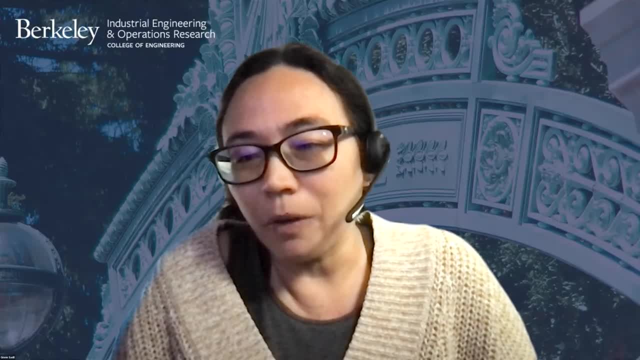 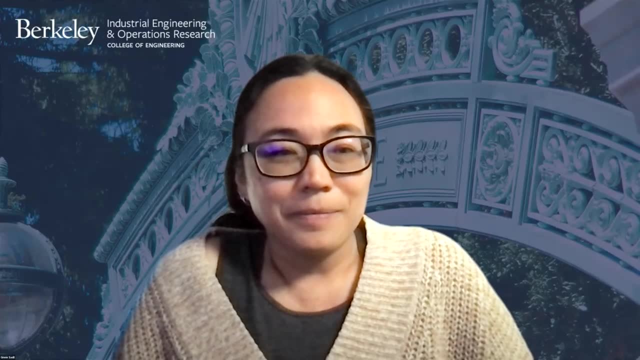 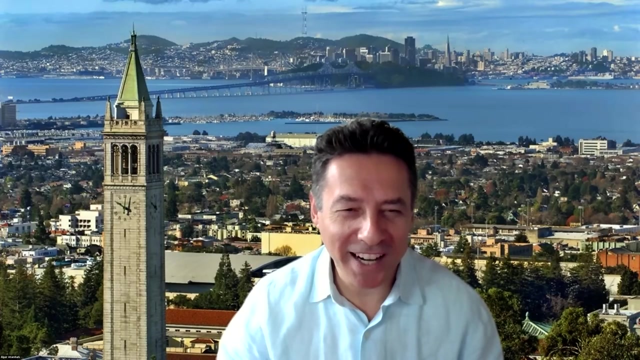 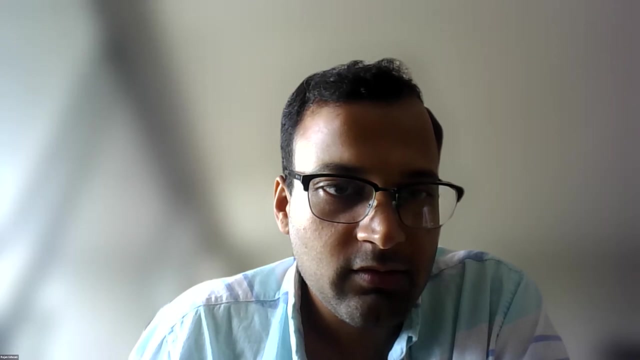 what kinds of internships, apprenticeships, are offered uh within iur and an ia se. would you like ANS? então, yeah, i know that the student uh organization is very active. i think victor wanted to say something as well. um, so, yeah, you can go ahead, victor. 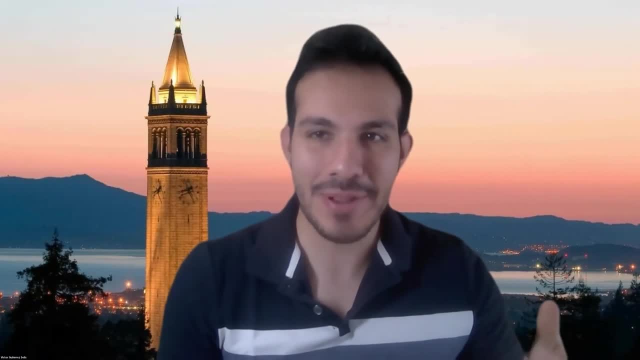 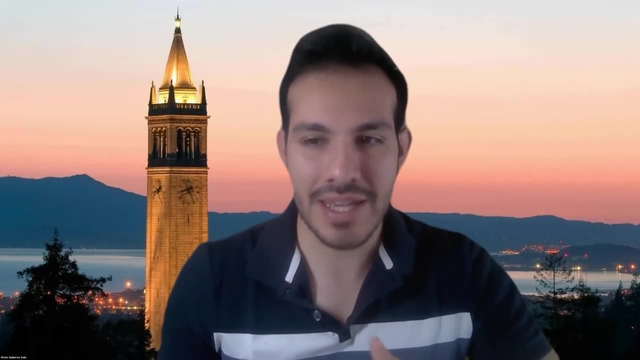 okay, i'm just gonna go first, like right now, this is my first semester, i'm looking for internships and it's I really like IOR because you can actually see when you go into websites- like we have, like as a student, we are allowed to use handshake- go to those websites and see what recruiters are. 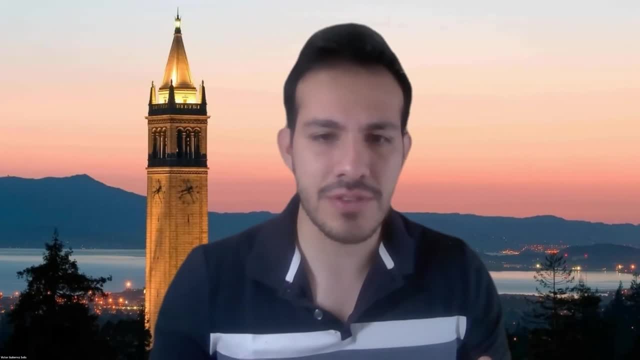 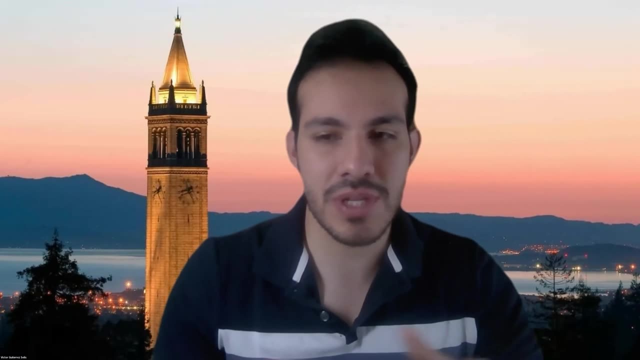 looking for for industrial engineers and the industry. there is like a lot of industry where you can go, but it's mainly like if you want to focus or you like, what internship you can actually do is more like focus on the process, for example, like logistics. I'm looking into one internship. 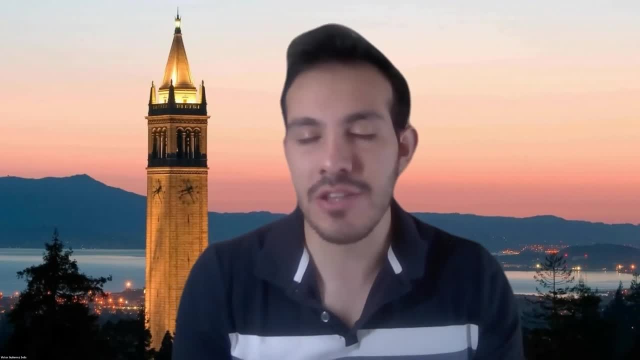 that is, it's a logistic internship that is going to be like a four-year internship that is going to happen. so, like, focus on the logistics, and that's something that I really like, that's something that you can do. but I also heard people going into like more technical kind of. 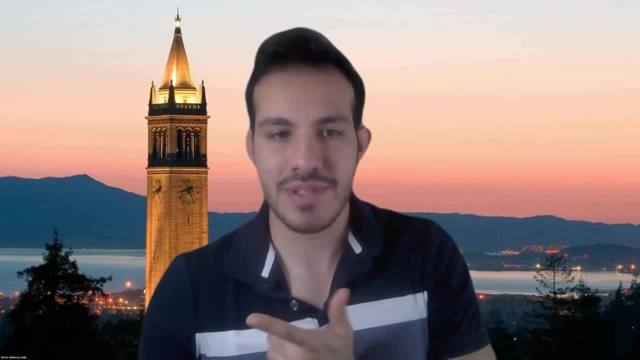 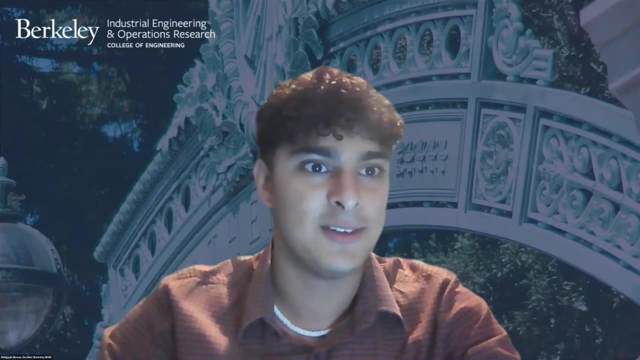 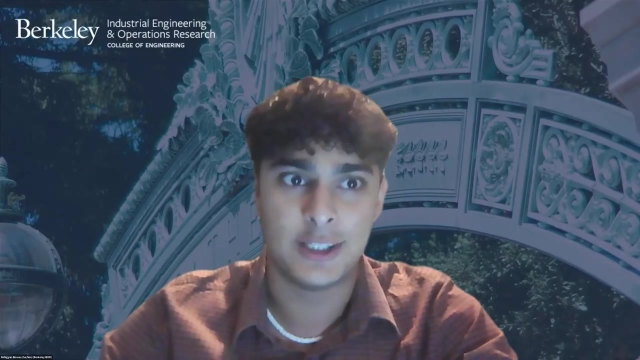 internship they can do. Yeah, definitely to echo. to echo what Victor said, you know, within like- and professor Adam Turk, you know, emphasized this earlier- IOR being the broad, a broad field, a broad engineering field, as it is, allows you to apply for internships within like it, in a broad amount, amongst a broad discipline. right, so it. 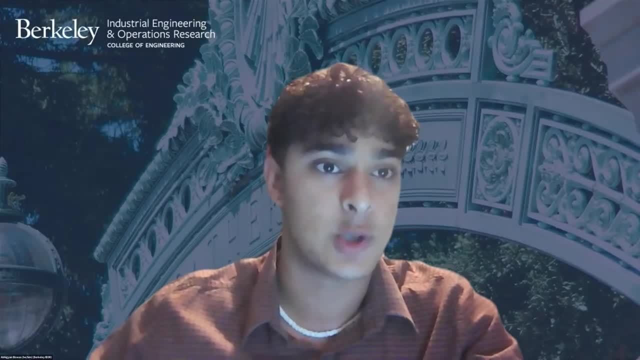 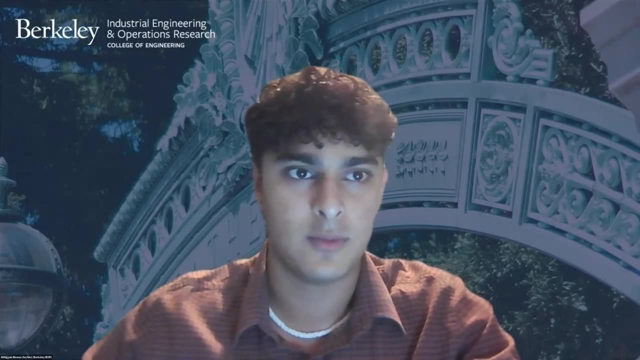 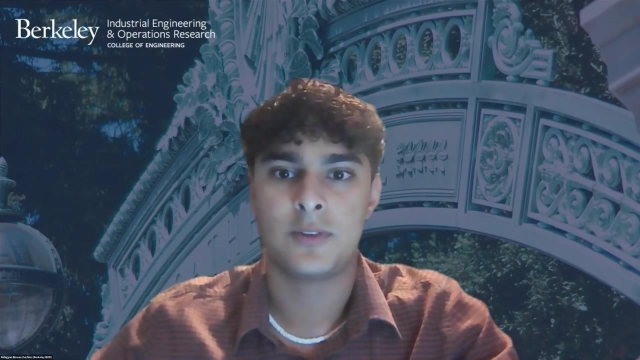 really depends on what you're looking for, what skill sets you're trying to improve and what industry you want to experiment in. that determines where your internship, what kind of internships you'd be getting Now in terms of support for you know, applying to internships and for kind of determining what. 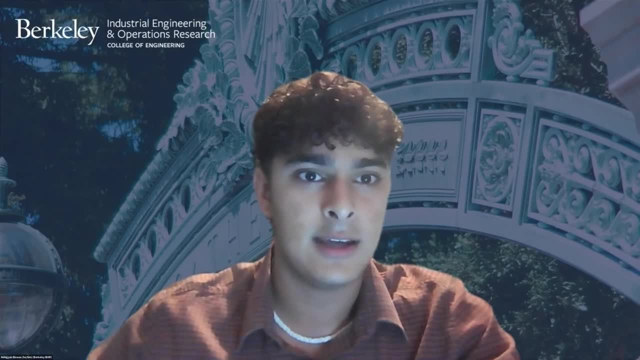 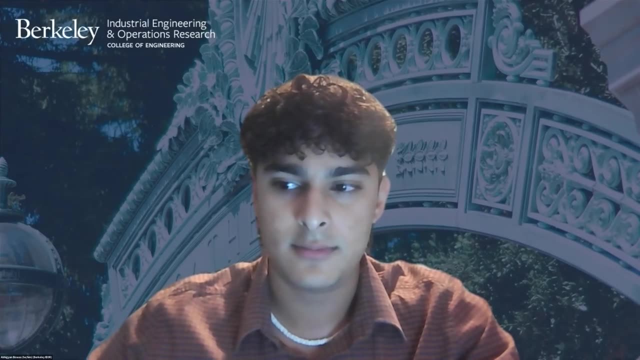 internships you should be looking at, where you should be looking at, ISC comes in and has you know meetings that we host to inform that, to inform where you should be going. what are certain certain occupations within the industry that are popular, how to get to those positions. 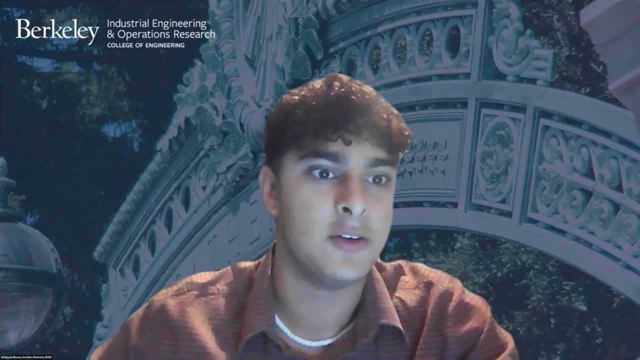 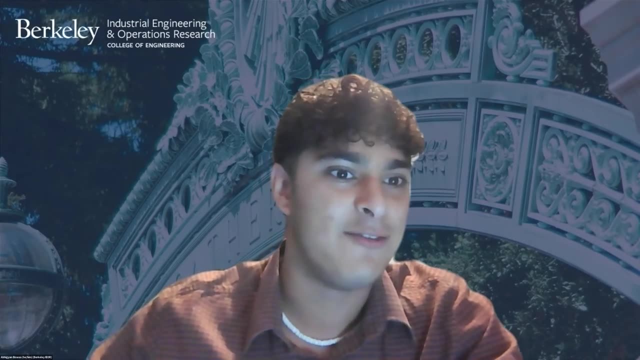 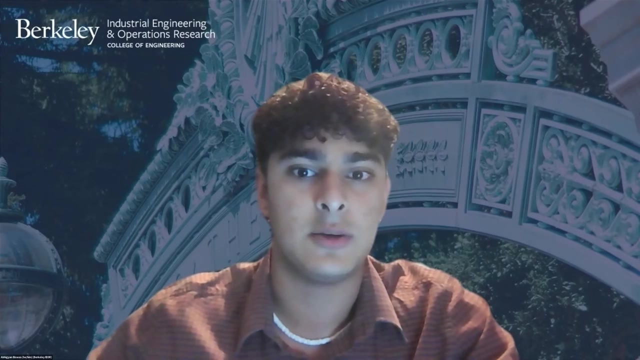 and other than that, we have our wonderful staff. you know, Ginny, I I'm I'm pretty sure Ginny and Goldie send like a hundred emails a week and they have wonderful information about internships, about opportunities, about all of that, including the information that we get from ESS, from other. 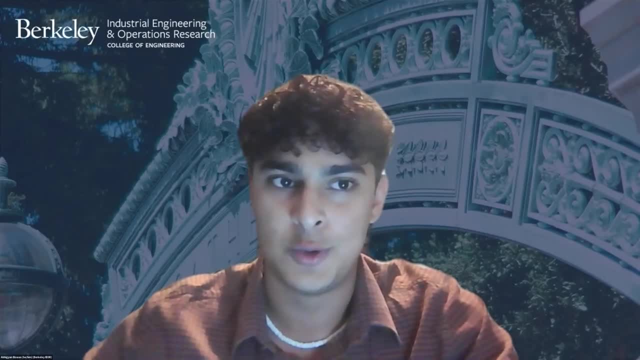 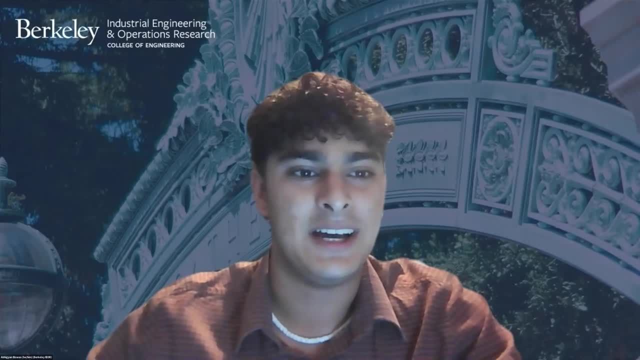 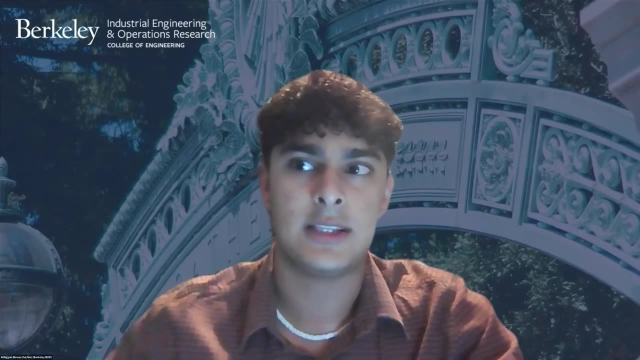 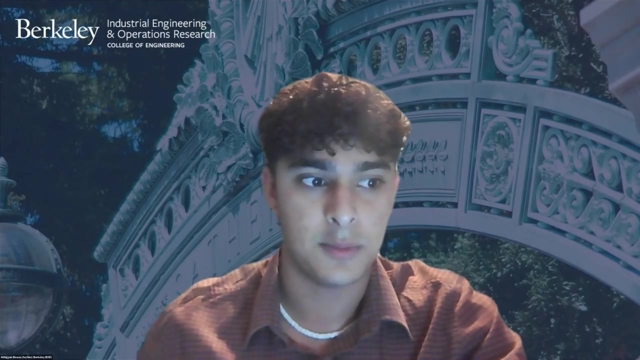 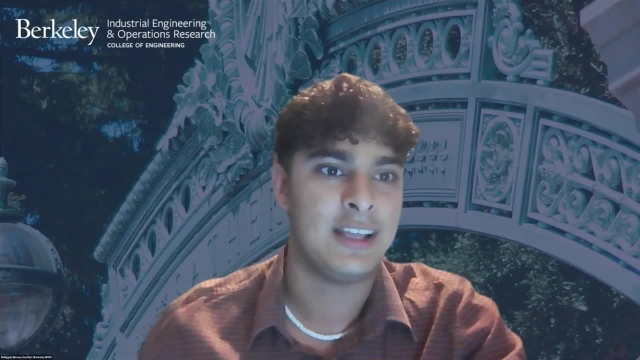 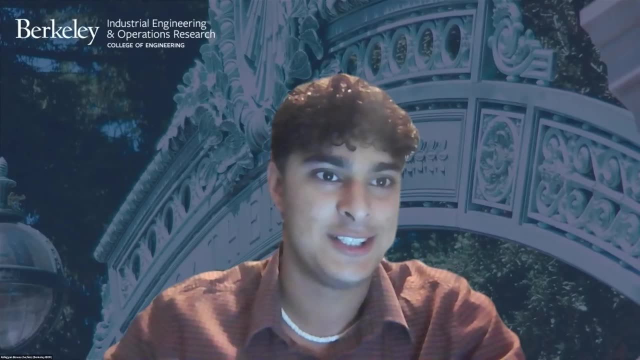 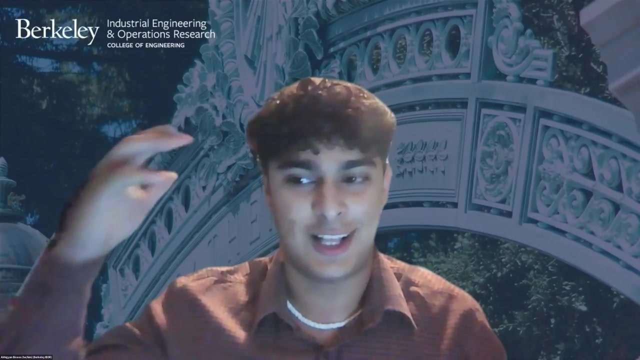 IOR. the difference really is the amount of information and the amount of resources and the help that you get. it's, it's absolutely mind-blowing. I remember my first day at Berkeley. I was given like I don't even know how many pages of information, just just a lot of information. 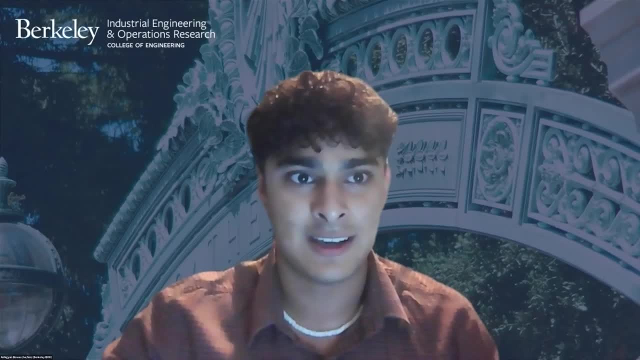 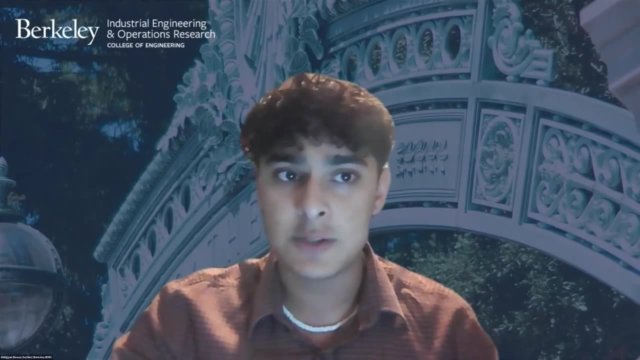 about different things, that you can do, different pathways. you can take post-grad, you know, preparing for those pathways, whether you want to be in academics, whether you want to go into like the management side of things, whether you want to be technical right. I hope that answers your question. 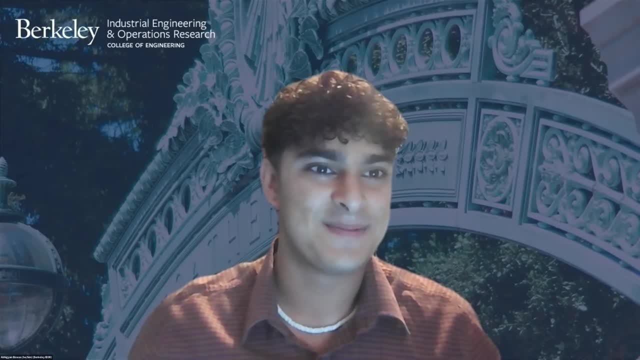 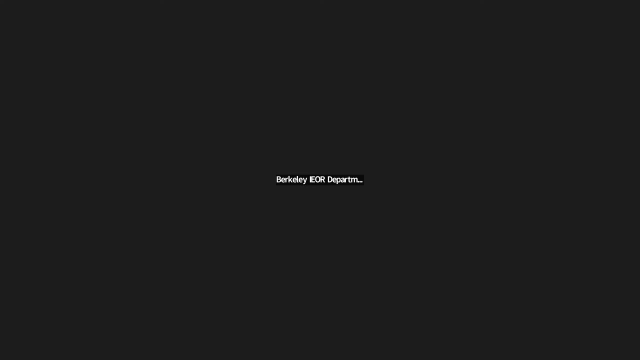 I'm not. I'm not quite sure I did, but yeah, a lot of students participate in summer internships at companies like Tesla, Neuro, SpaceX, and IISC is very good about organizing info sessions, so recently they held an info session with Procter & Gamble, where an industry rep came in and spoke. 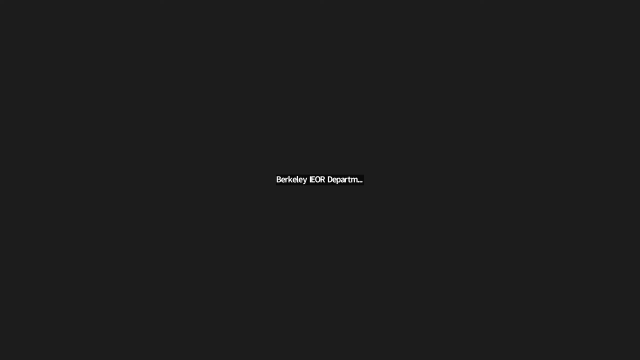 about the different opportunities. this week, Micron came in to talk about um different internship openings, so um the the students are very, very actively engaged with industry um, and typically I think roles include data analyst, product manager internships, um, things like that. yeah, I agree with Goldie, there is a. there's a lot of diversity in the types of 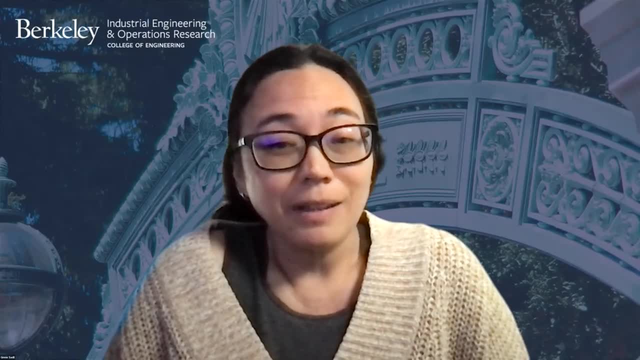 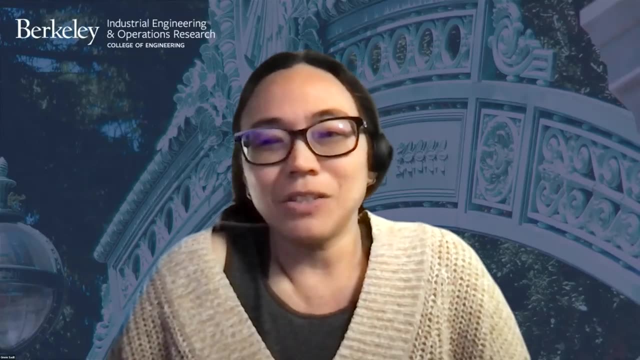 internships, where students do. they work for many different types of organizations, but you know, they're, you know walking the floor on Amazon or they're doing um, they're working as a project manager. I mean, IISC just did a presentation a few days ago, which is one of the reasons our student groups are so active and wonderful about. you know what? 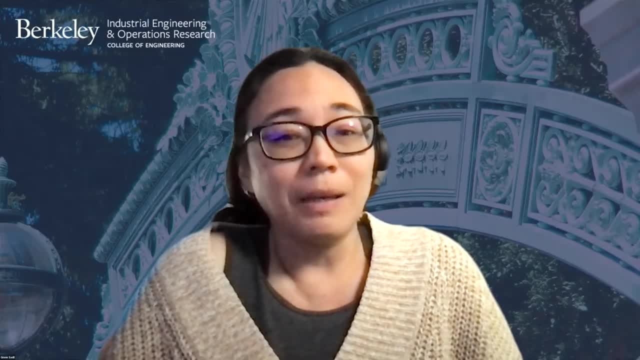 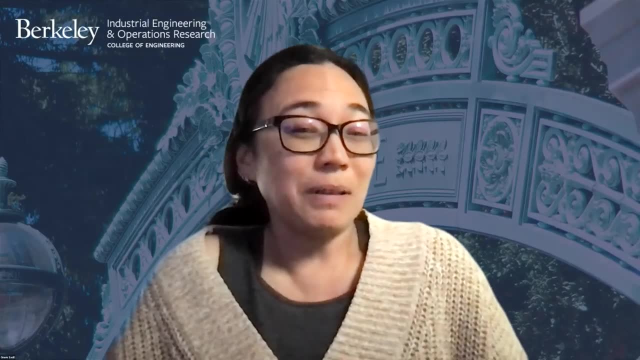 it is to do an internship. they had students who came in who have done uh, who are PMs, during the summer to talk about what it is, what it entails, to give the students the idea of, like, some sort of background before they do their application. so you know if it's something that doesn't appeal to. 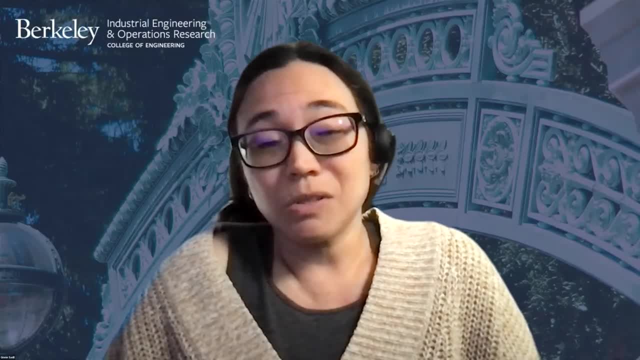 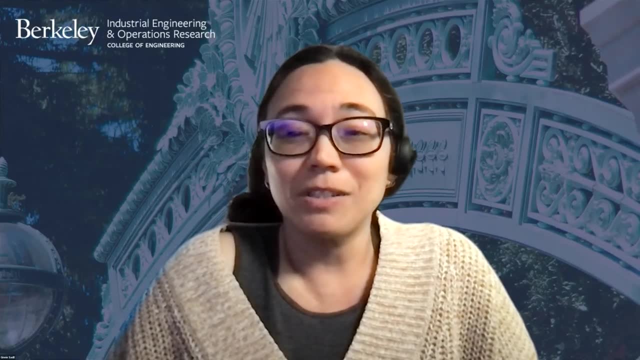 them or something they're really, really interested in, to give you as much information and resources so you can make good decisions about what you want to do, um, and where you want to. to look for your, your pathways, um, because there are many different directions to go um. anybody else have they're. 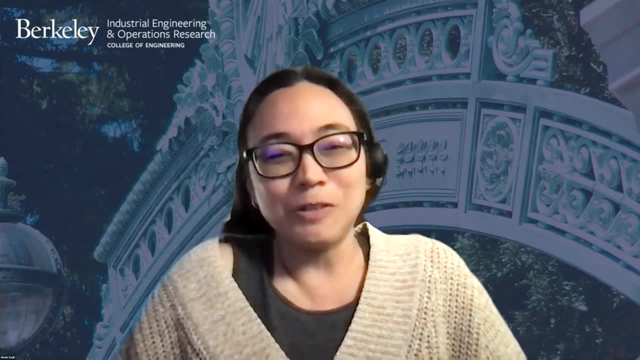 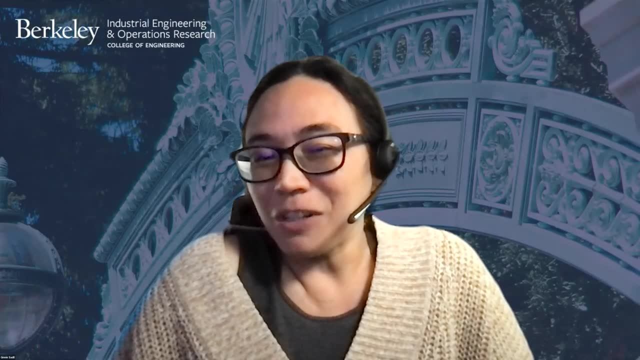 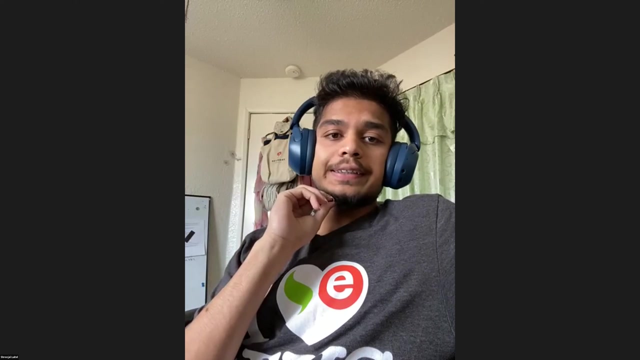 sharing. uh, like I know, Victor and Angela, you're um, you're in your first semester on campus, so, uh, it's kind of hard to say um. but Shijal, do you have any, um any, internship experience you want to share? no, absolutely. uh, there's quite a few uh hands down. I think it's important for you to recognize 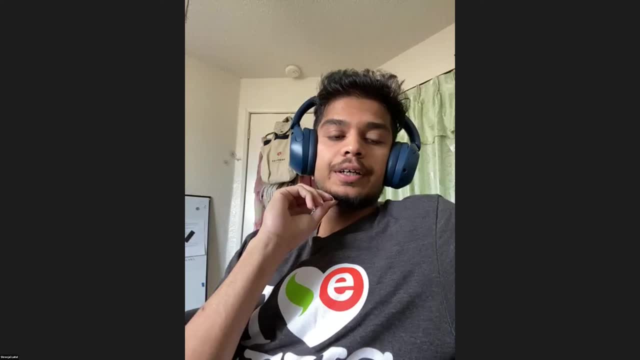 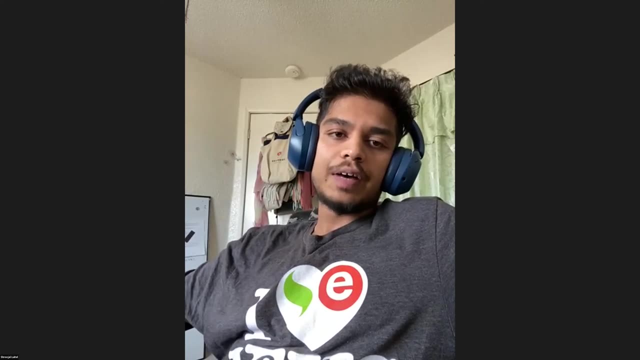 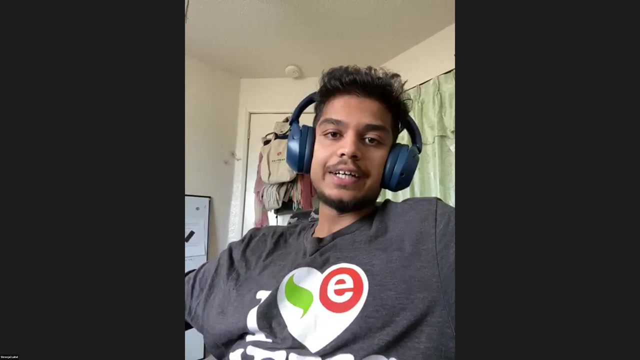 that the alumni community is also open uh to share information about uh different internship activities. for instance, um I was able to present to the IUR advisory board a few months ago and I've still kept in touch with a few people from there, a few individuals from there like specifically. 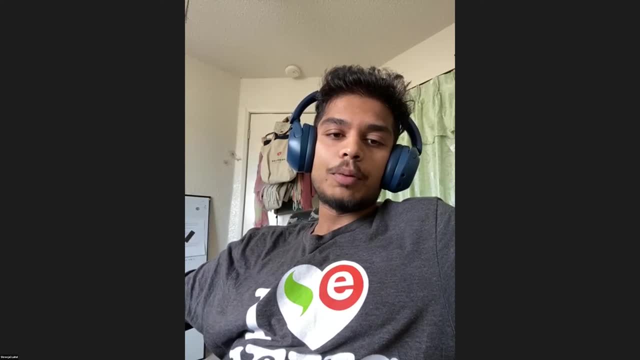 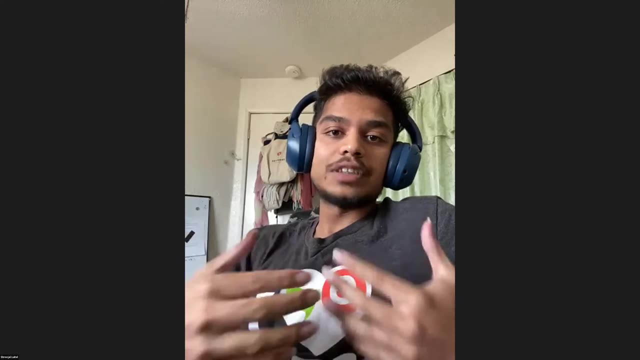 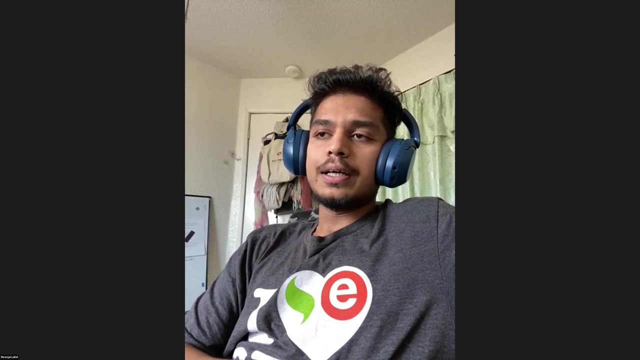 Terry and and uh and Todd um, and both of them are in two different uh segments, right, I think one is in PG&E and the other one is in uh. I mean he he's kind of retired but he went through the entire MBA process and and worked for Sony for quite uh some time. but I think it's important to tap in uh and 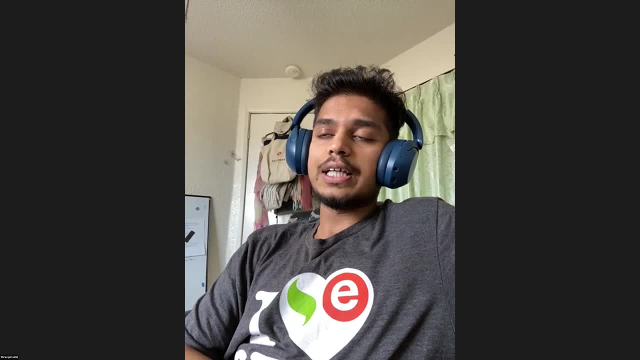 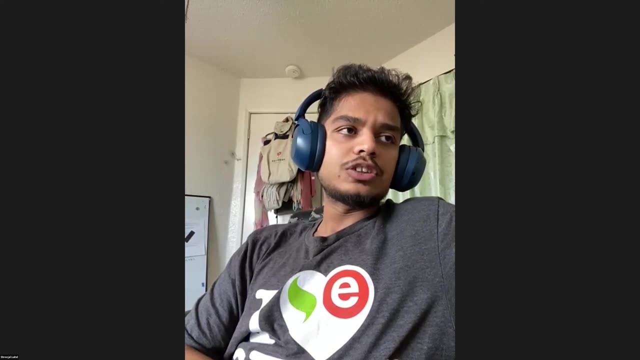 to recognize that you have the ability to connect with uh individuals that that were alumni that can help you uh navigate that entire application process. but beyond that, too, right Berkeley is known for its entrepreneurship. I think, if I'm not mistaken, there's a few LinkedIn posts that I ran. 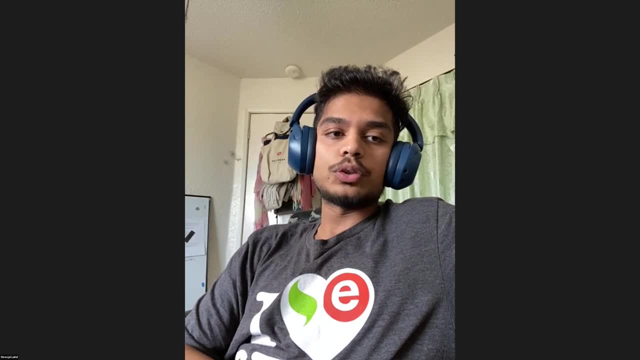 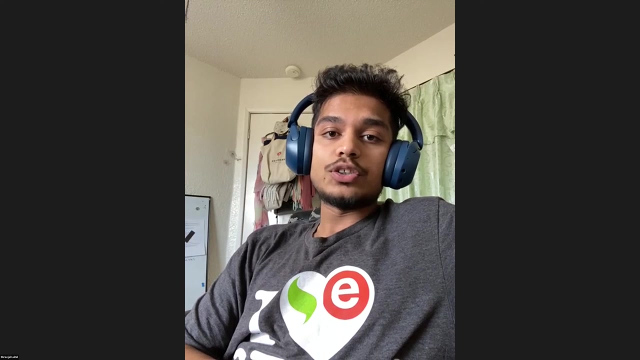 across. that says how. that speaks volumes about how Berkeley's entrepreneurship is. is uh one of the top uh programs basically in the entire world. uh, for, for their entrepreneurship department too. right, so we have a great community. before I've worked on a Skydeck uh startup, um, and and for me to just kind of tap into uh Skydeck opportunities and Skydeck. 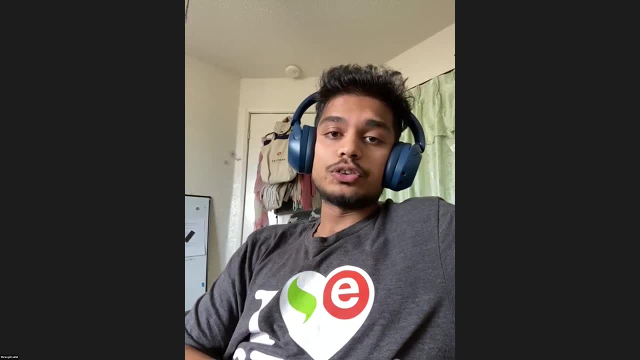 internships for me, that that was quite helpful as well. um, and and also just uh, working with other Skydeck founders on on different projects could help open the door, uh to more internship opportunities. but I will be Frank, you know. I mean whether you want to work for like a smaller uh. 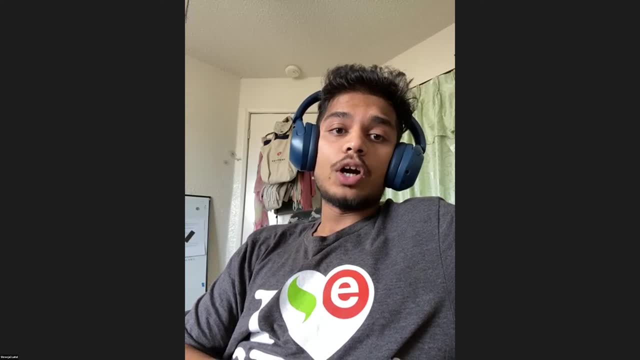 segment, like a startup or if you want to work for, like a larger company, there are definitely going to be resources to help you, um, help you, navigate that entire uh process- uh, from at least what I've found right. of course, there's going to be competition, but I 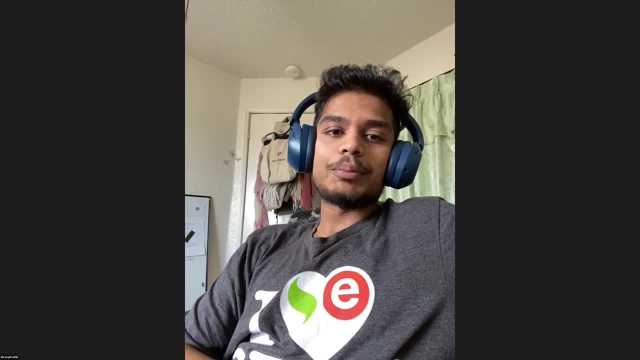 think recognizing like ATS systems like Berkeley is already a brand name in itself. uh, so it it takes a lot more, or it takes a lot less selling for Berkeley students than it does for uh students that that might be uh attending schools uh somewhere else. uh, at least from my perspective. 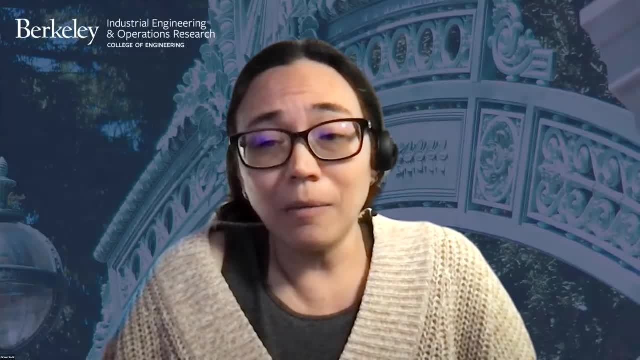 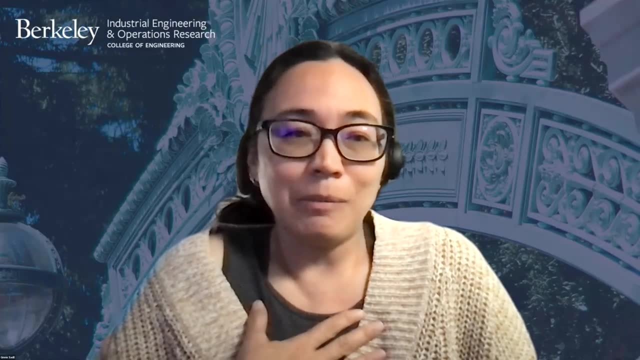 thank you all, and so we're running out of time today. thank you all for coming um. I wanted to uh to remind everyone that if you wanted to have, if you have any additional questions, you're welcome to reach out to me. my um. my email is in the chat now. it's g oh g sadil um at berkeleyedu. 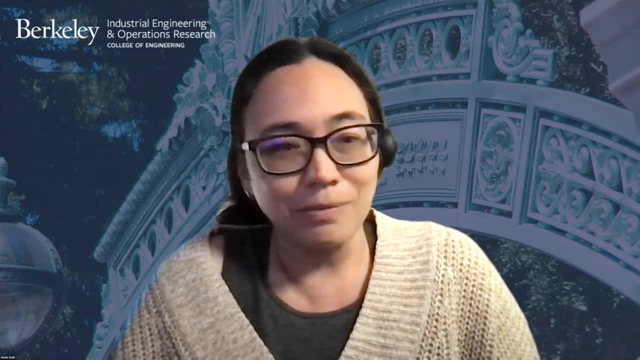 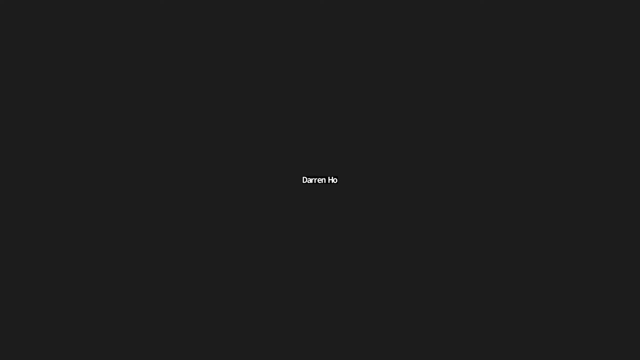 um, and I guess we have one last question, if you guys don't mind going over for just a minute more. um, if that, if that works, we just give her the very last question and wrap everything up. yeah, thanks, Jeannie, really appreciate it. um, so I think you guys made it overwhelmingly clear um, how the IEO our 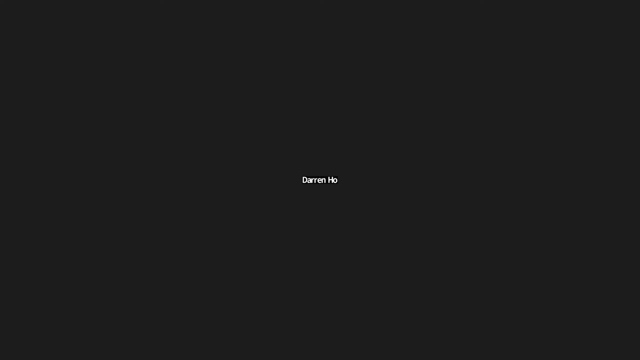 department is moving towards industry and all its applications. um, I'm curious to hear more about like, what like actually research within operations. research actually entails though, um, you guys touched on I mean like a lot of the applications are like. yeah, I'm just curious to hear more about like. 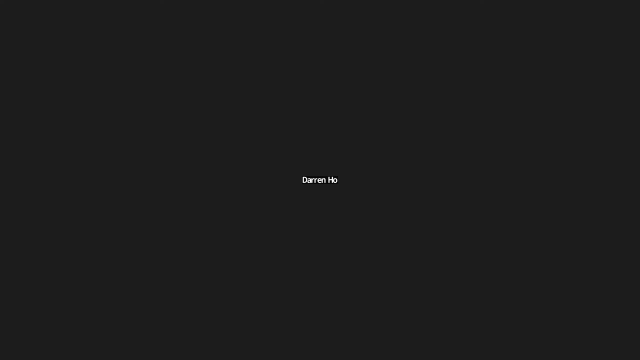 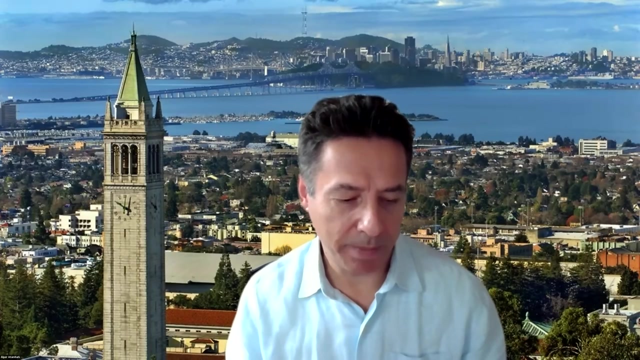 what that process looks like and what your work is like really like, focused on sure, um, um, I, I can speak to that. uh, this is an undergraduate, or at the program we're focusing on the industry in practice and and education, um, um for um. similar info sessions related to the master. 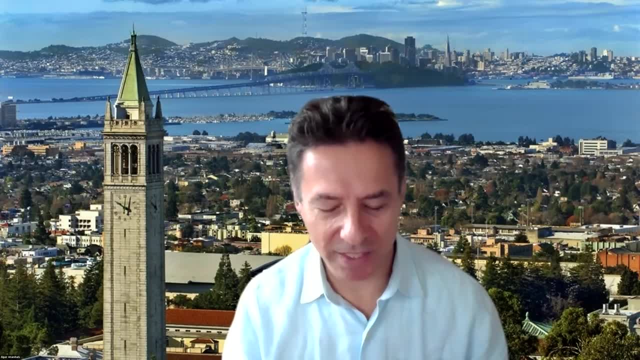 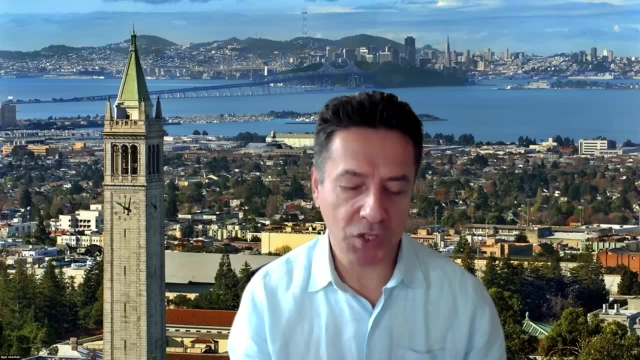 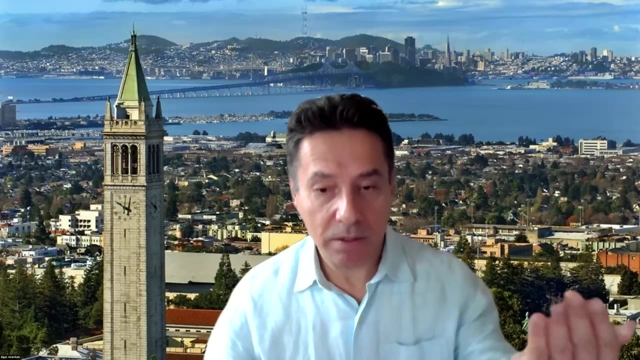 and PhD students. we'll be focusing once more on the research active piece of public department um um. so first up, since we're running out of time, I just want to mention that department web page. We have a research research page there and I would highly encourage you to. 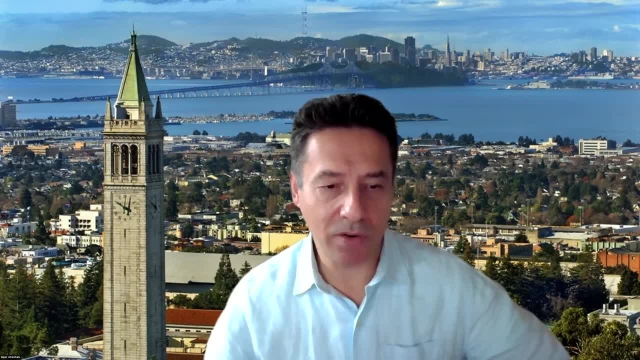 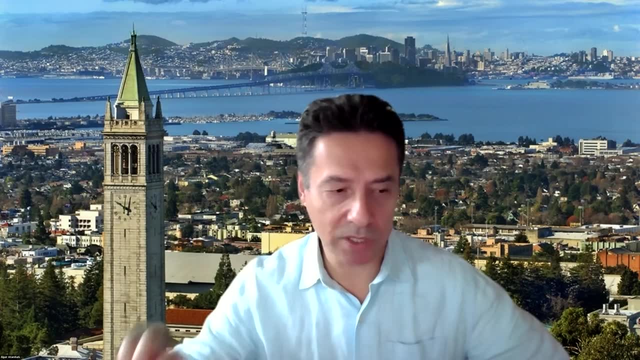 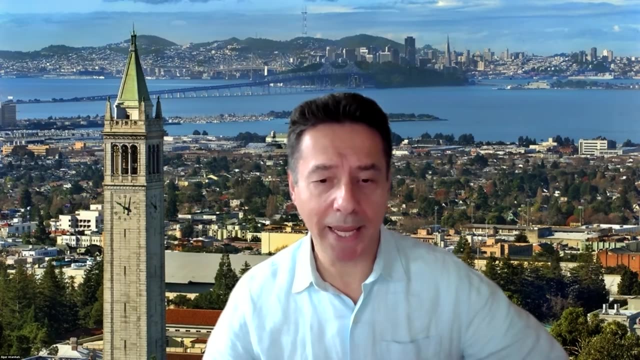 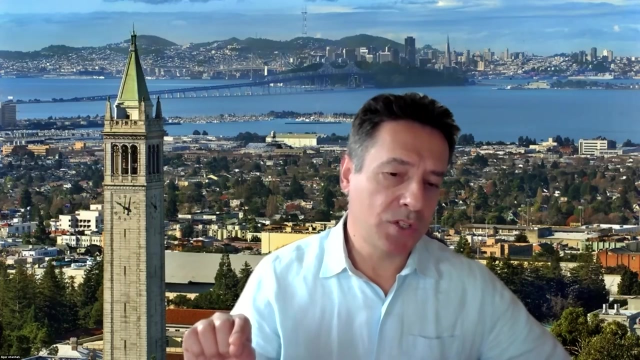 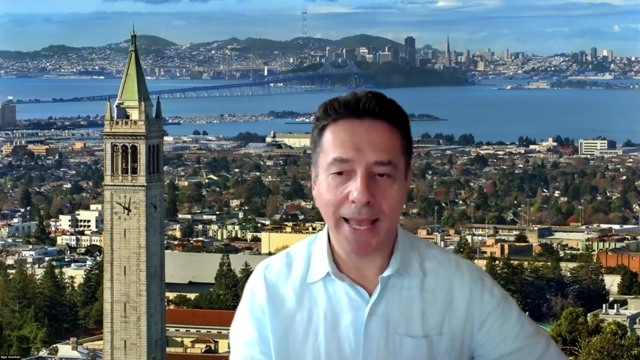 take a look, and it's broken down into some different areas, such as optimization, algorithms, machine learning, stochastic systems, robotics, automation and various industries. Definitely it's something to look at, and there are also news articles there on the web page that show the research impact that IUR faculty and students are doing and- and this is really- 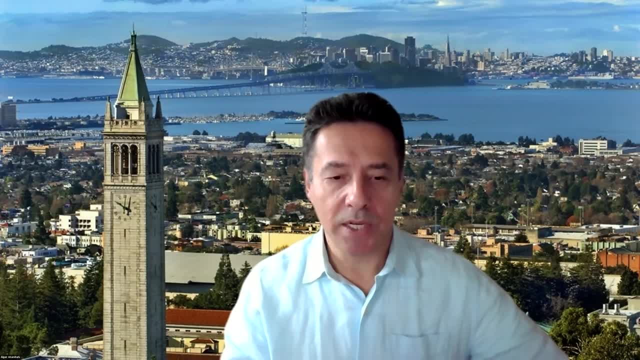 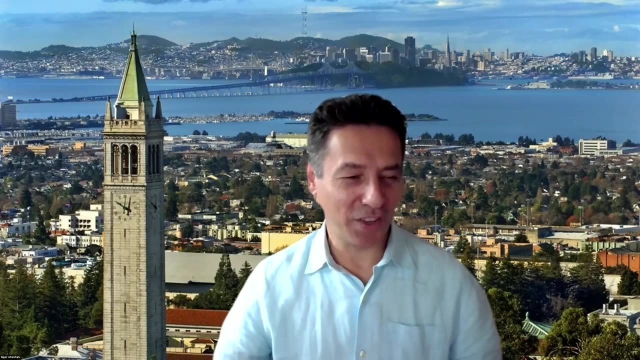 the cross-cutting across different areas, whether it's in, you know, early detection of cancers through education, advanced machine learning methods, or whether it is tele-robotics to be able to do the surgeries, remote surgeries in the healthcare system, or whether it is in the area of the integration of 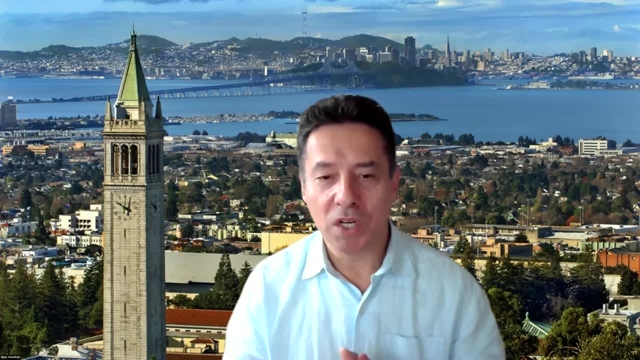 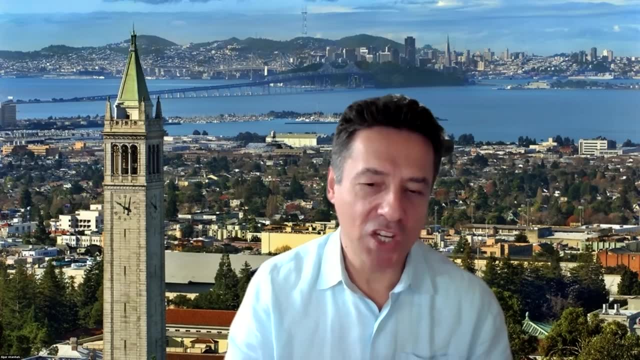 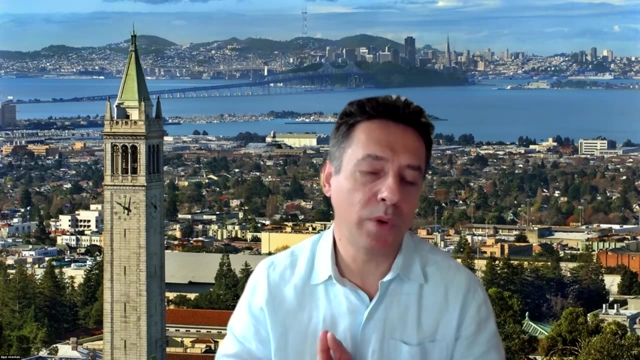 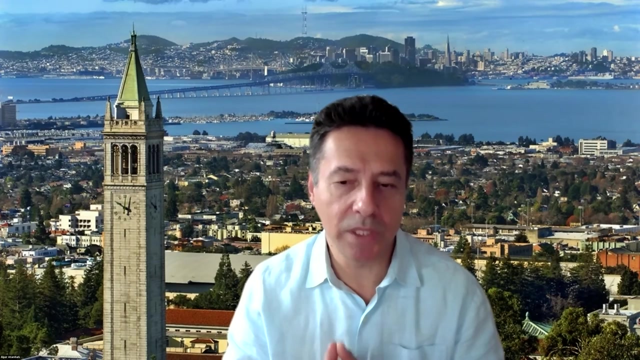 AI and optimization techniques or right sharing and taxis, etc. So we have a lot of information on our web page and even sort of faculty's research papers are can be downloaded from the their web pages. so definitely I'd encourage you to take a look there. but it is really across across the board. our- our faculty, are sort of top researchers in their areas. 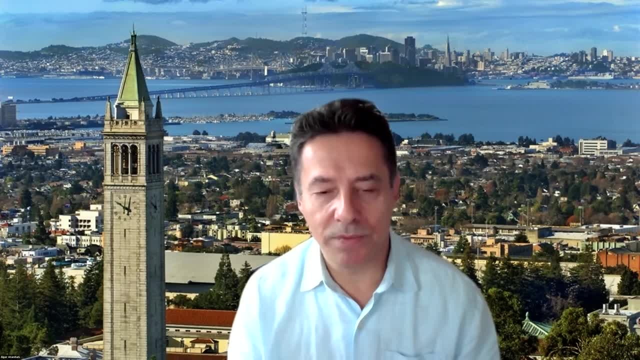 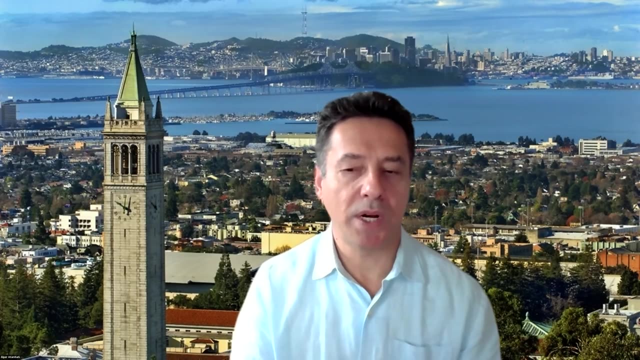 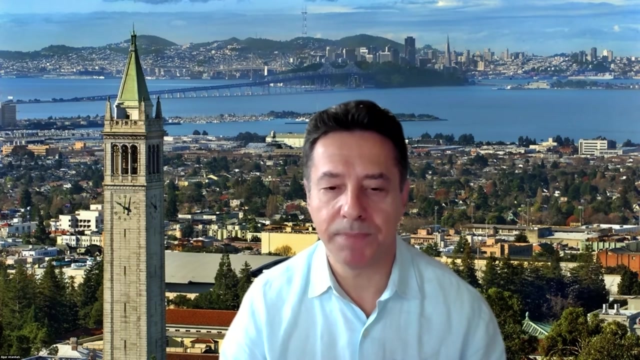 and they are editors of academic journals and referees and and they have all of them for the groups, obviously, And so I'm going to go ahead and give a little bit more time to the students that help with the research projects as well. so, and I'm happy to you know, tell more offline at this presentation if 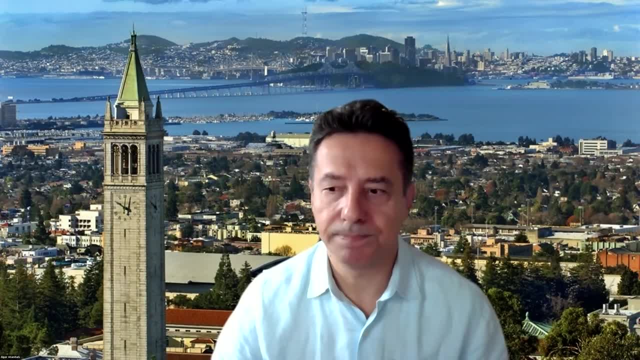 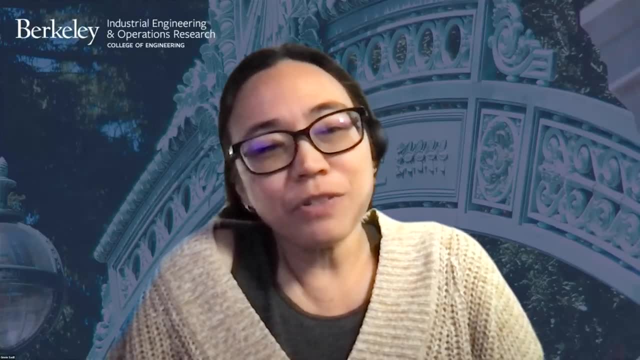 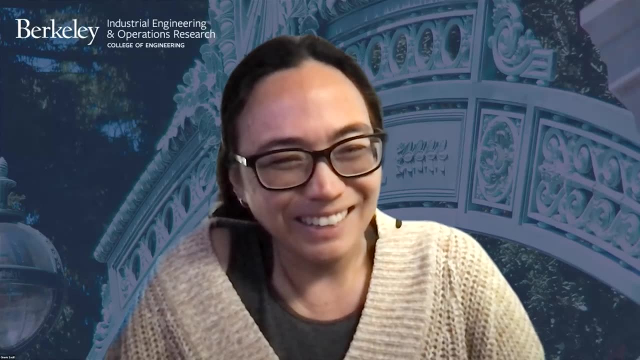 you're interested in teaching that too Great. thank you again. any parting words of advice from our- our current transfer students to the transfer students for applying this semester. I think one of the first things you can do is to stay dedicated. I mean, I think it's a really good thing that you've been able to go to this semester. 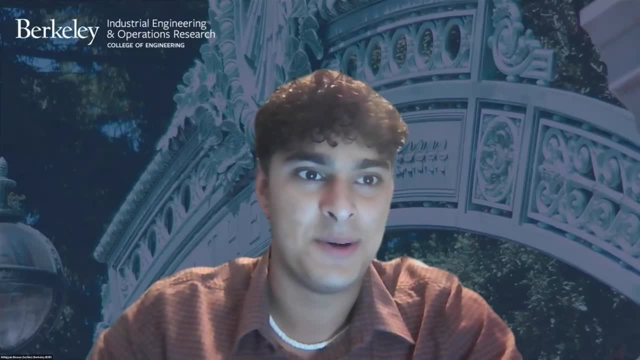 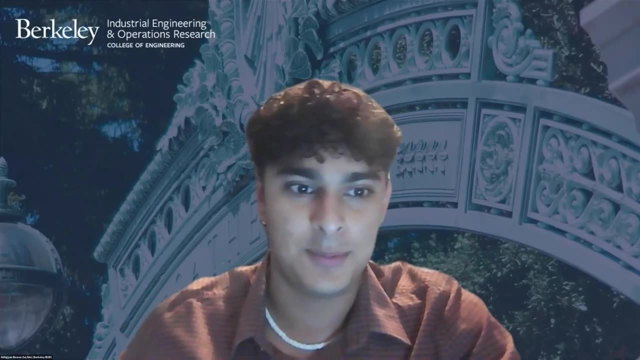 you know, it's not like you're going to be like, oh, I'm going to be, like I'm going to take this month. excuse me, it's November, Just stay dedicated. It's. it may feel like you guys are almost at the end, but even after this, stay dedicated. 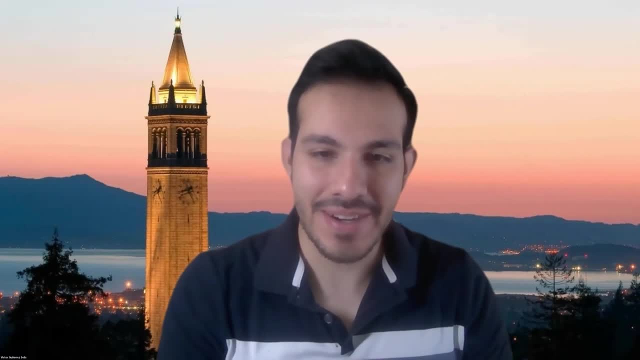 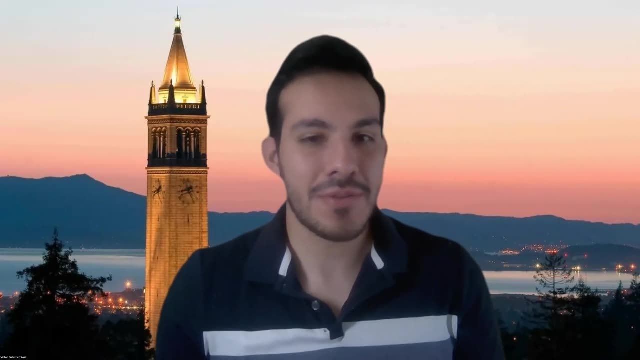 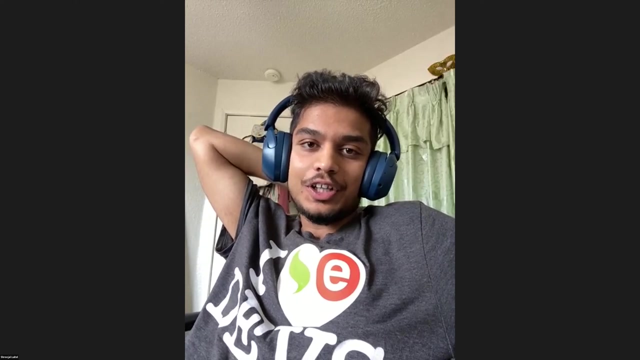 and you've made it so far, so I'm proud of you guys. keep, keep it, keep it going. Yeah, so IOR is a really good major. If you ended up coming here, you're going to have like a better experience. so yeah to everybody. yeah, it's also overwhelming at times because, uh, with the application process, there's a. 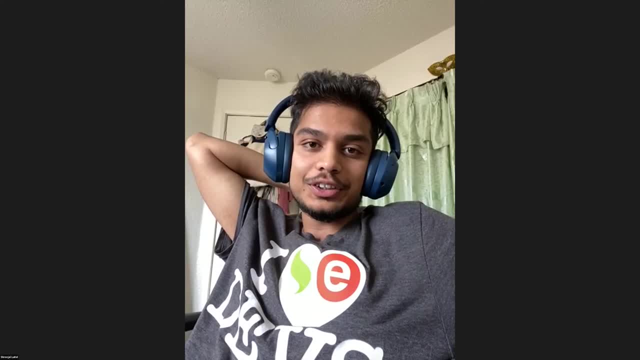 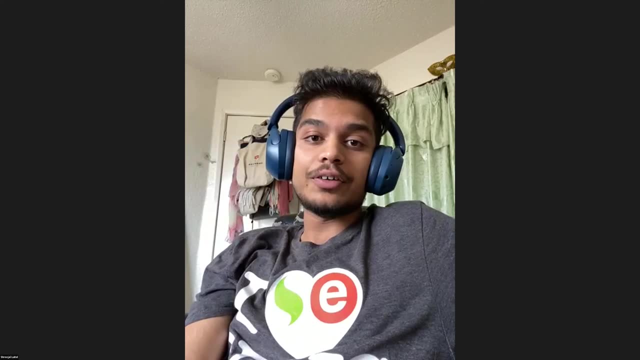 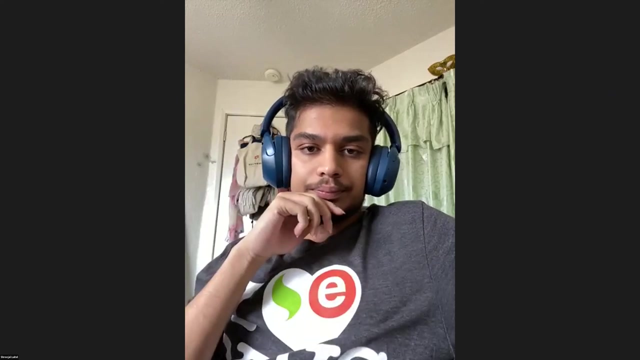 lot of stress, but just know that it's only a few uh days or uh before you know it's. it's all kind of like over and the stress just kind of like calms down. so i encourage all you guys to reach out if you guys want. my email is just my last name, firstname at berkeleyedu and just wherever. 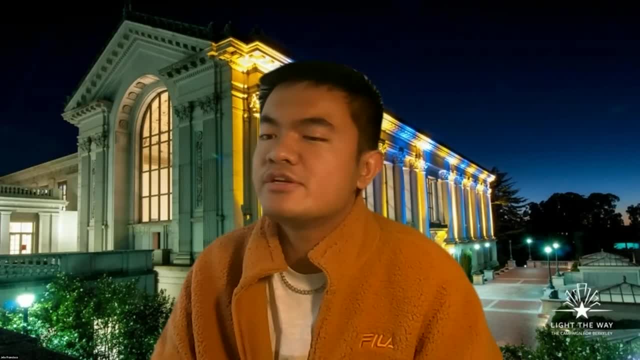 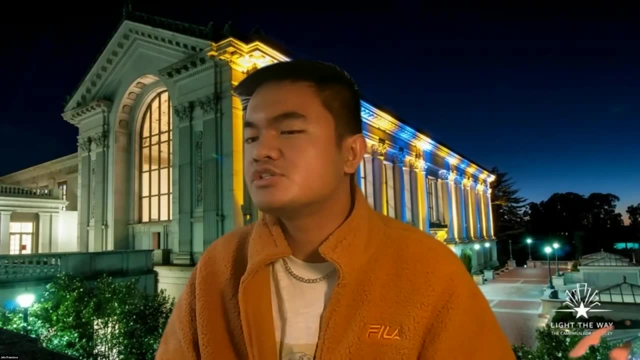 you end up, um, just know that there are a lot of resources in any university. you, um, you get into and don't be, just be confident. just apply to internships, just apply for research, um, even if it's your first semester in a university, because i've been applying and i've been getting some